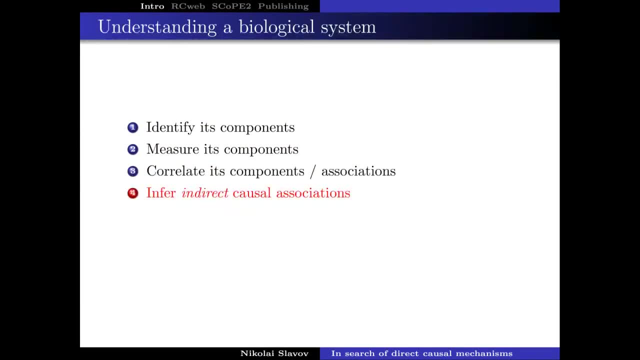 compare causal associations. Now, if these causal associations are indirect, it is actually surprisingly easy to infer them. You might think inferring causal association is the pinnacle, the hardest thing to do. Not necessarily. I will give you some examples, at least in model organisms, where indirect causal associations are rather easy to identify. 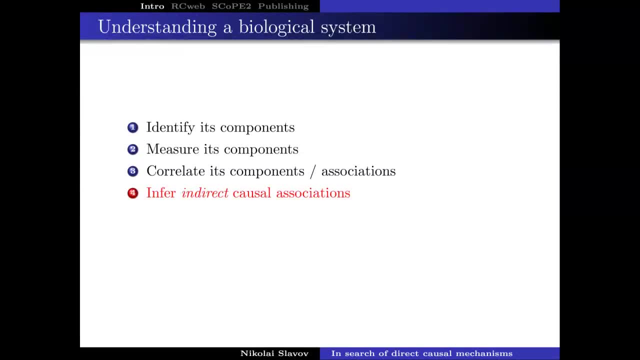 but they're also not very informative and not very useful. Now, direct causal interactions are much harder generally to identify and that will be the big emphasis in the presentation: How do we go from indirect to much more direct mechanisms And ultimately, the thing that happens? 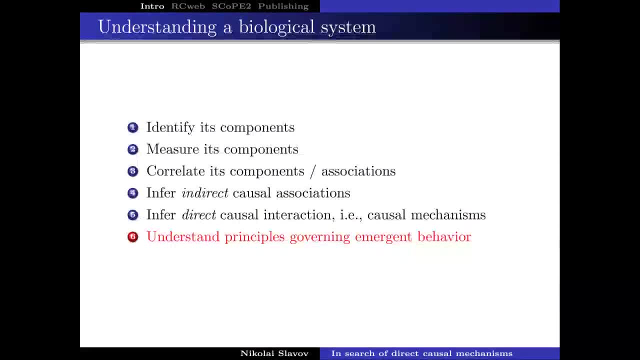 rather rarely and we celebrate is if from all of that we can distill common underlying principles that govern emergent behavior. most of biological functions are emergent behaviors. that's wonderful and happens rarely. Certainly, doing four and five is not equivalent to doing six, but to the extent that we can do five much better, I think we are also closer to 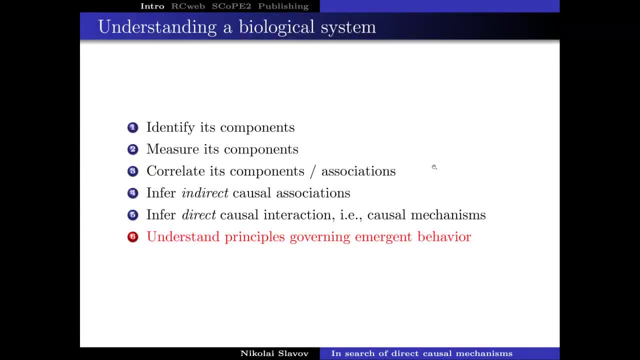 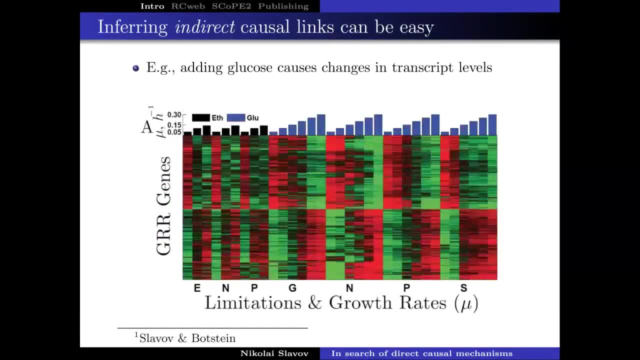 being able to identify principles governing biological behaviors. So let me start by giving you an example of how you might very easily infer indirect causality. This is a data set that they generated when I was a graduate student about your career stage. If you have any cell culture that you're growing, whether mammalian or yeast or any other condition, 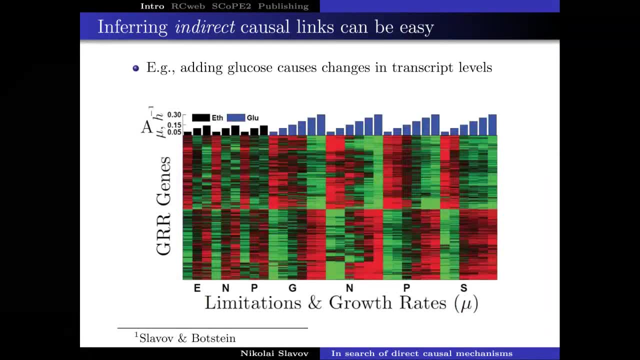 you can change one factor at a time and you can measure downstream results, such as the abundance of messenger RNAs. and what you measure, if you change only one factor in your system, is a direct result. It's causally generated by the factor that you change. So if you, if you put glucose to your culture of 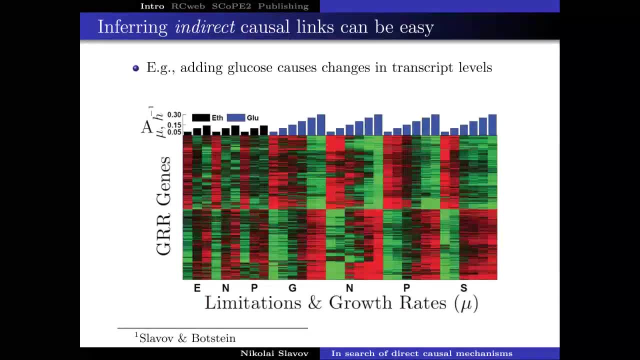 cells and then you measure messenger RNAs levels. you're going to find that glucose causes some messenger RNAs to increase in abundance and others to decrease, and in this case I was studying the growth rate of cells in and its association with the abundance of many transcripts in different 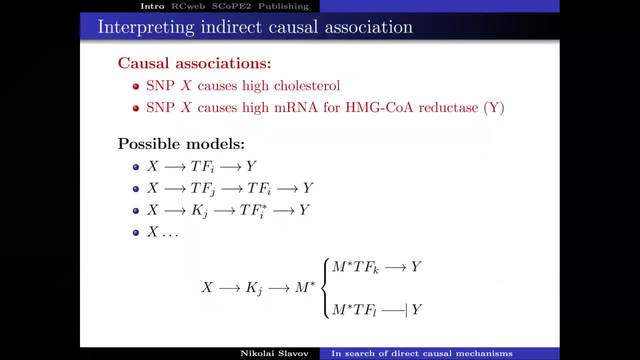 conditions. But I want to illustrate the limitation of this kind of indirect inferences with a case study of a very important biological system relevant to human health, and that is the regulation of cholesterol, which we all know is associated with atherosclerosis and multiple morbidity in the human population. 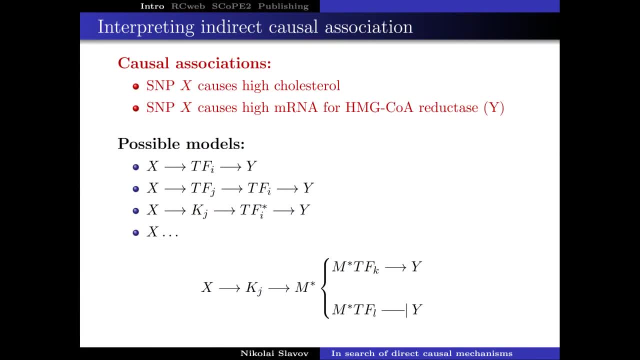 What is commonly done these days in the post-genomic era is to identify multiple SNPs or single nucleotide polymorphisms across population in many, many, many individuals, and then we can associate them, compute based on a model. we can compute some association between those and phenotypes of interest, various diseases they can. we can associate them with messenger. 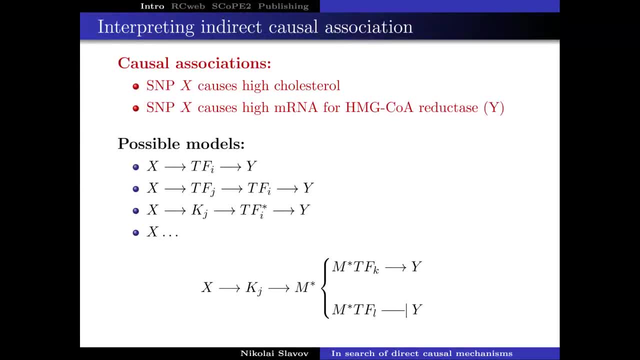 RNA levels and so on and so forth. So let's just assume that we have done one such study. there is a study called genome-wide association studies and that study resulted in two very confident conclusions that are. we are going to assume here, for the sake of argument, that they're bonafide. 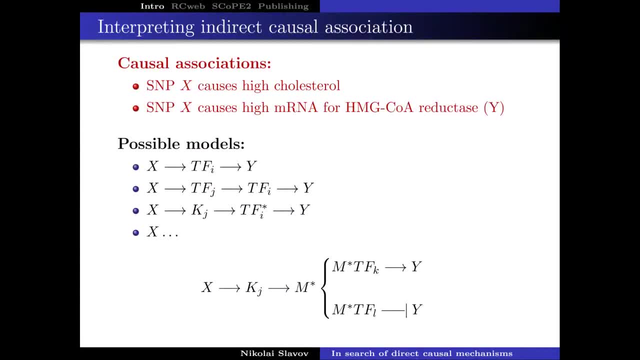 causal associations. we know- that's god-given truth- that SNPX is associated with high cholesterol, causes high cholesterol, and also we find that SNPX causes increased abundance of the messenger RNA for HMG-CoA reductase. HMG-CoA reductase is one of the key enzymes regulating 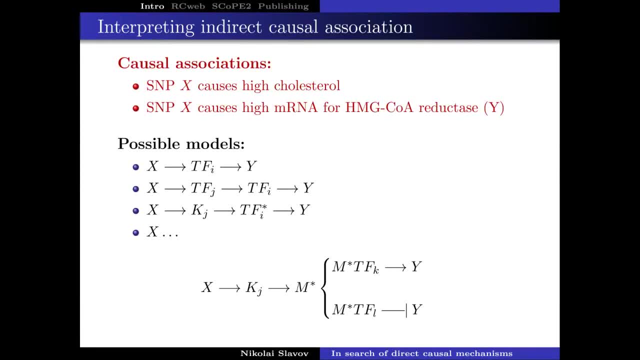 cholesterol biosynthesis and the enzyme is inhibited with multiple pharmaceuticals that are used to treat atherosclerosis and that for many, many years have been the most profitable pharmaceuticals on the market. It's a very important regulatory step in cholesterol biosynthesis, So my question for you is: 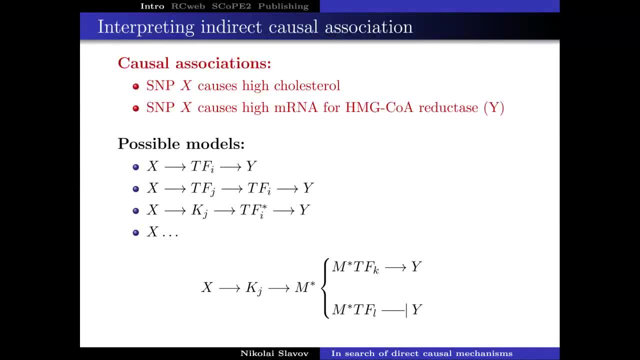 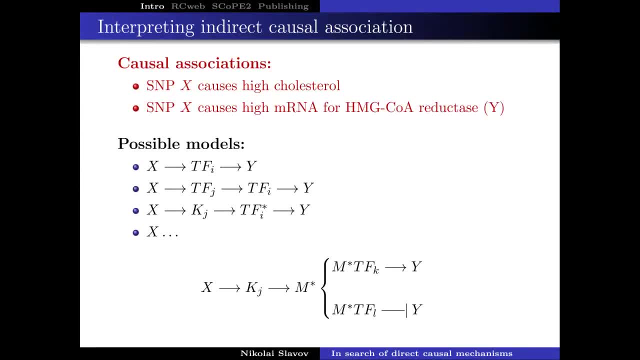 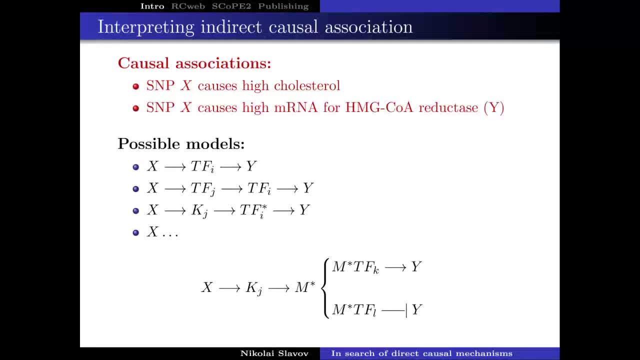 That's right. So it seems likely that this might be one possibility that this particular SNP, increasing the messenger RNA, might contribute to more cholesterol being synthesized. But that's certainly not the only possibility consistent with the data and in fact there. But that's certainly not the only possibility consistent with the data and in fact there. 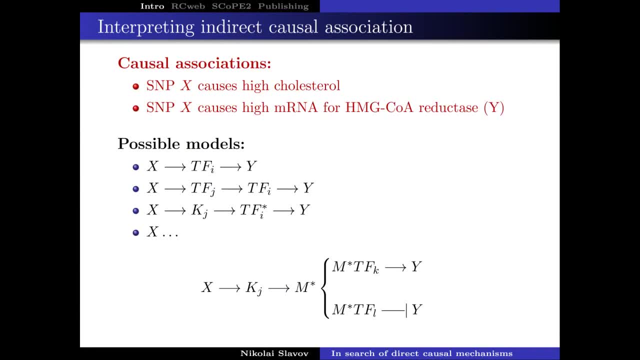 many, many possible models that one can write down, that they're all consistent with these observations. In particular, it could be that SNPX, which here I denote with X, causes the increased levels of transcription factor I. that then facilitates the synthesis of the messenger RNA Y. 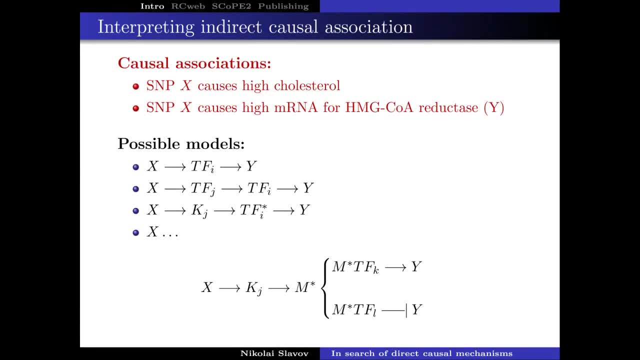 It could be that SNPX actually activates another transcription factor J. It could be that SNPX actually activates another transcription factor J. It could be that SNPX actually activates another transcription factor J that then activates a transcription factor I. that then causes the induction of the messenger RNA. 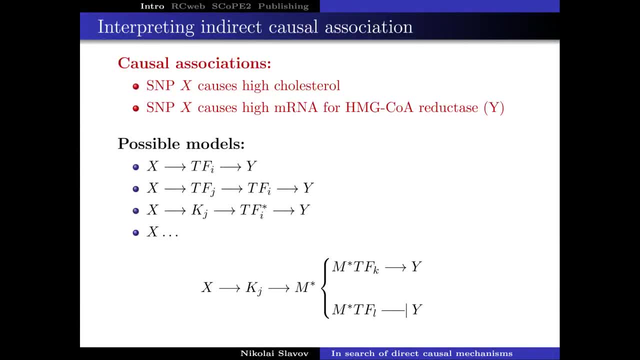 Or it could be that the SNP actually increases the activity of kinase J, that then phosphorylates transcription factor I, that then induces HMG-CoA reductase transcription, And could be a zillion other similar linear models. Or it could be also branched models, as I have indicated on the bottom, where you have SNPX. 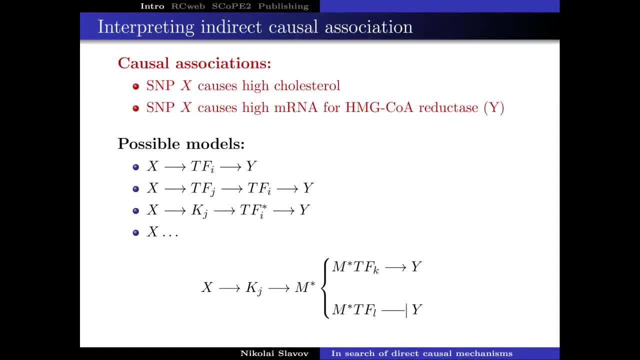 Or it could be also branched models, as I have indicated on the bottom, where you have SNPX causing increased activity of kinase J that then phosphorylates to the mediator complex And the mediator complex, if interacting with transcription, factor K induces the transcription. 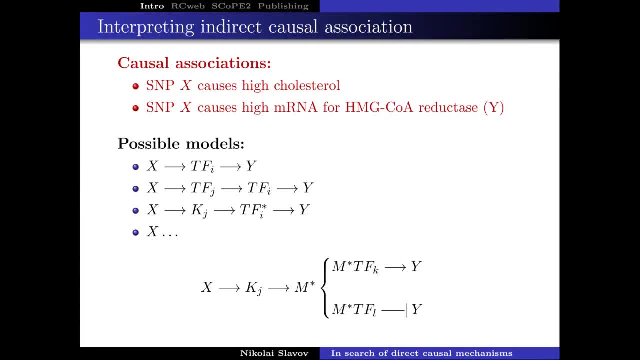 of HMG-CoA reductase. If, on the other hand, the phosphorylated mediator complex interacts with transcription factor L, it suppresses And could be that one team has more patients. one team of researchers analyzes more patients in which the first branch of the pathway is active and finds 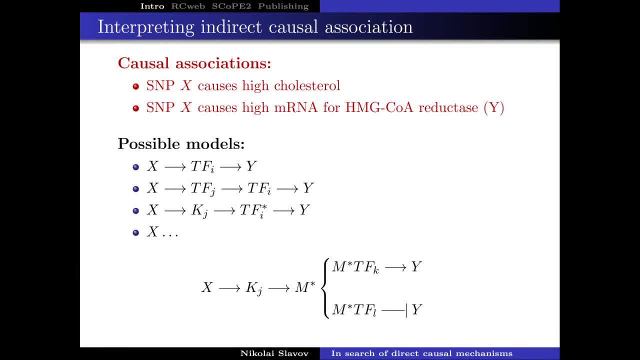 positive association. And another team activates another subgroup of patients in which the second interaction is happening and finds a negative association. And not only that, these things can be happening one at a time. all of these zillion models can happen simultaneously in principle, theoretically considering. So even if we have these bonafide very high 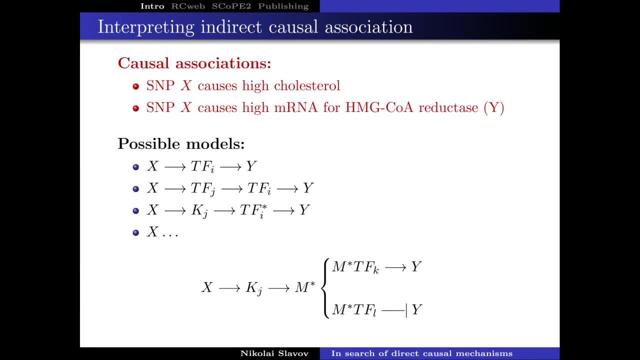 confidence-based patients, we can still get the same results. in the same way, If we have evidence-indirect causal associations, our ability to interpret them is quite limited because there are many, many, many possibilities consistent with them And we cannot rigorously exclude any of them without doing more experiments. We have to. 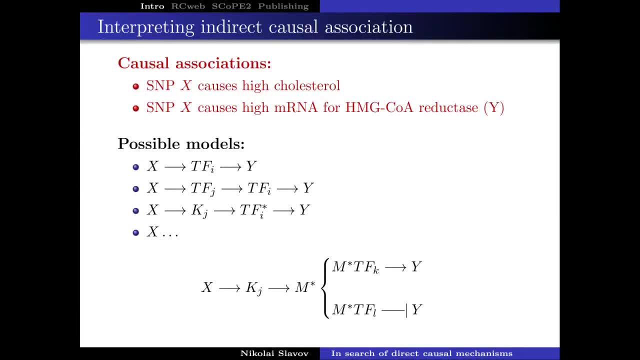 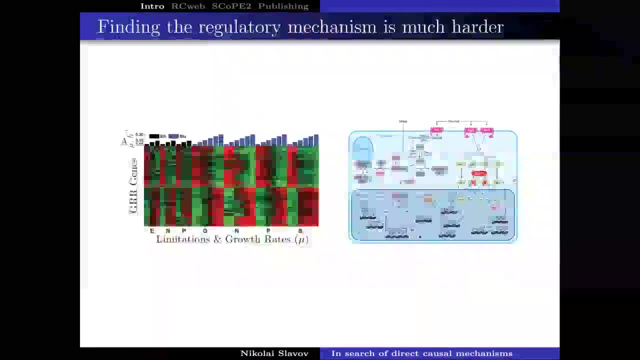 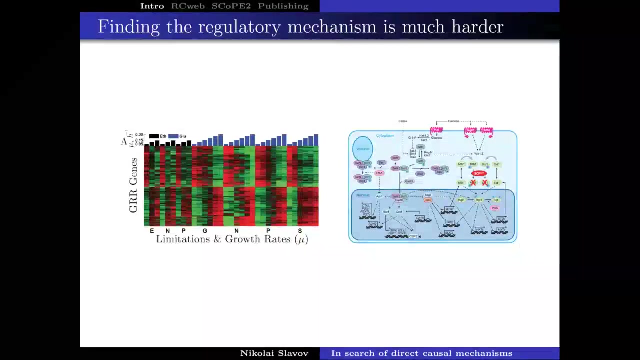 go to a more direct association. because if we actually had evidence that SNPX is directly regulating any of these components here on the slide, that will be much, much more straightforward. So we can interpret much more invariant. So while it might be easy to find the causal association of adding glucose and having induced 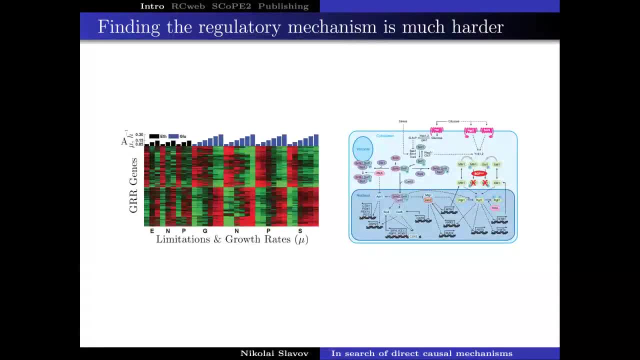 transcription of many genes. finding the mechanism that is causing that induced transcription is much harder Here. what I'm showing on the left- And this picture on the left- traditionally has been drawn based on literature analysis of lots, of, lots of individual low throughput experiments and has been generally lagging very much behind. 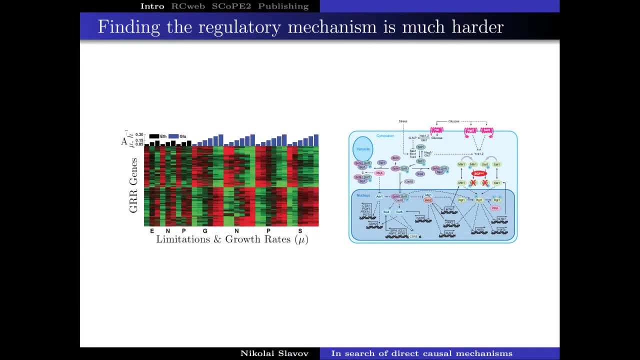 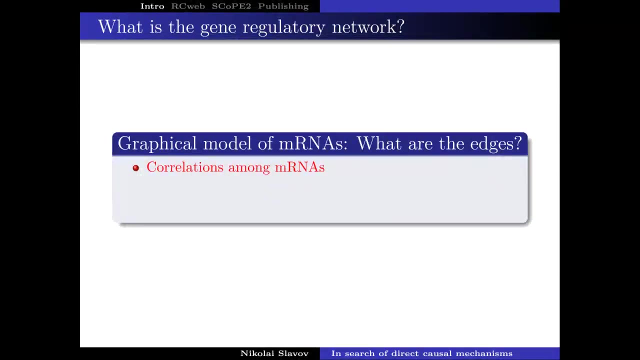 our ability to generate large scale data sets and just infer associations, including indirect causal associations. So one way to try to bridge the two worlds is to try to find out regulatory networks S, And here I want to discuss a little bit what regulatory networks might be and what they need. going back to the beginning of our class, when we discussed some 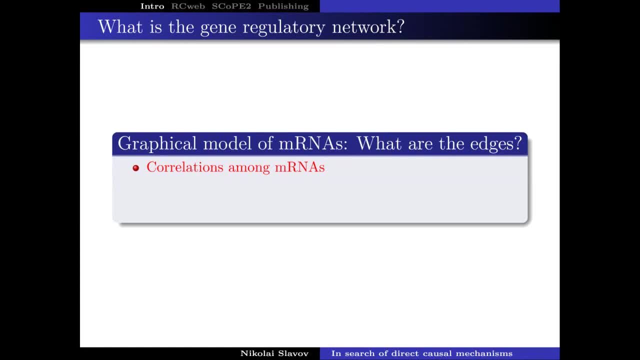 methods for inferring such networks. Now, the simplest type of network that we might build is simply by correlating messenger RNAs, their abundances, across multiple conditions, and say that the nodes are the messenger RNAs and the edges are their correlations. 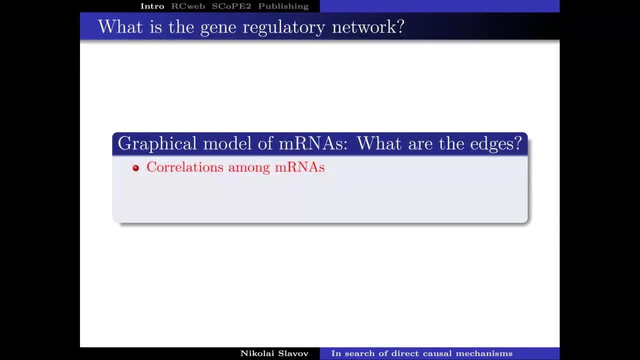 We may choose to threshold them. So if the correlation is above a threshold, a certain threshold, then we put an edge. If it's below that threshold we don't have an edge And obviously that's somewhat arbitrary And obviously that kind of network doesn't. 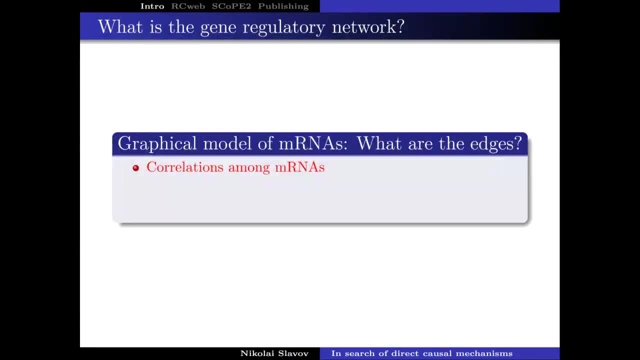 correspond to direct mechanisms or regulatory interactions, such as stelsis, which messenger RNAs tend to co-variate together, And many of these co-variations are going to be indirect. It is not going to be direct, It is going to be indirect. It is going to be indirect, It is going to be indirect. 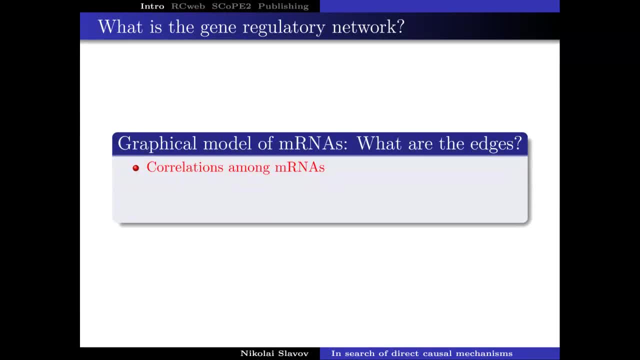 So we can say that messenger RNAi is causing the levels of messenger RNAj, but rather the two might be caused by another transcription factor And people. the first approach to try to distinguish a little bit with those direct and indirect associations is to make a model And based on that model we can say if we account for. 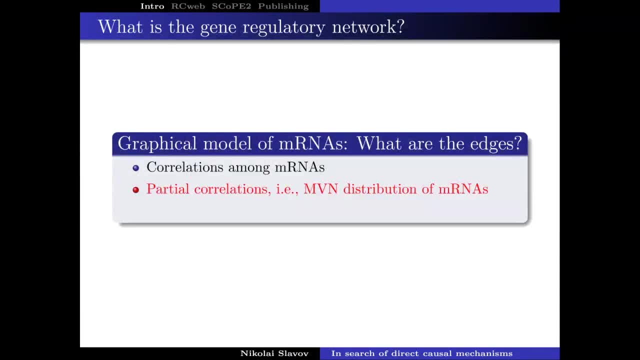 the interactions between this subset of messenger RNAs, we might be able to deconvolve and throw out these indirect associations. So what kind of model you're going to make if you don't know the underlying interactions and if you don't know the functional relationships between them? Well, the simplest thing is: 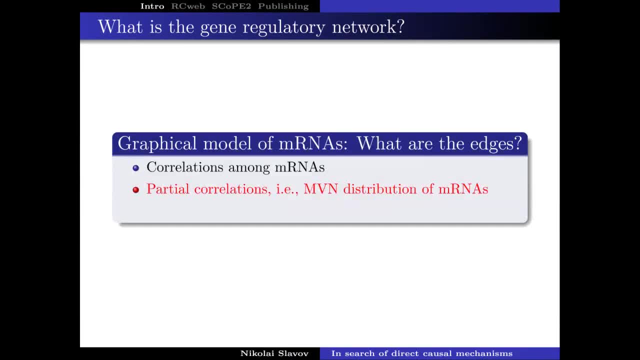 let's just model everything with lines, linear relationships, And it should be emphasized that this is done out of simplicity and convenience rather than because we think that this is really what's going on in the system And the corresponding associations. if you were to do it with a linear model, 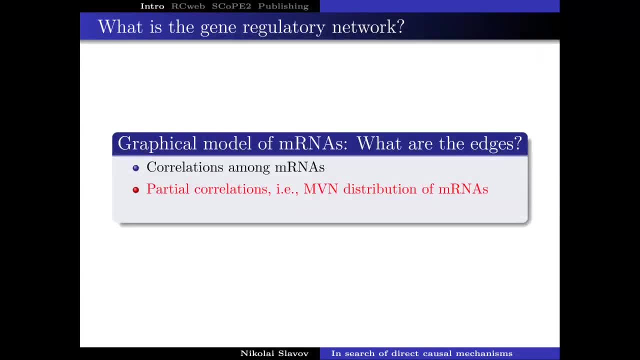 are called partial correlations, And that corresponds to essentially inferring a multivariate normal distribution over the messenger RNAs. There were many, many, many papers published on this variation in early 2000s And, as we have already discussed in class, we can do a little bit better than that. We can relax the 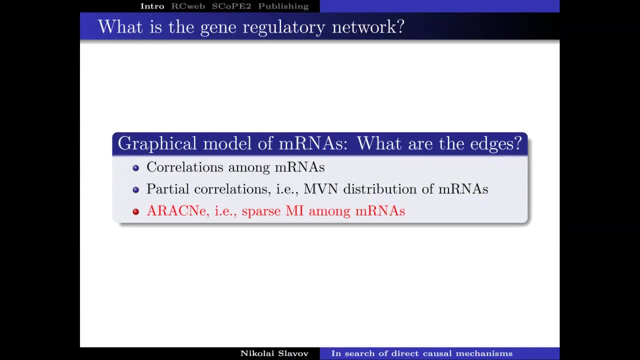 assumption of linearity. We can do a little bit better than that. We can relax the assumption of linearity, potentially by using mutual information, And that allows us to account for arbitrary nonlinear interactions in principle between the variables that you're analyzing, assuming that we can compute the mutual information which, as we have discussed in class, 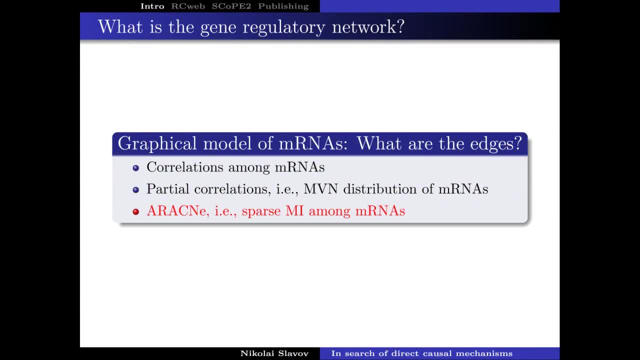 is not trivial. It's actually very difficult to reliably estimate joint distributions criterion in visible aftermath. Public Interrepresented Identitariness. Professor Sonar Thewa, Now let's say you do that, Let's say you've done arachne to the best data site you could generate. 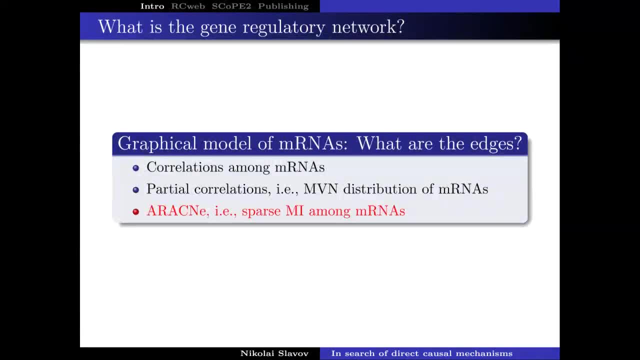 and to find that the mutual information between RNAi and RNAJ is very high. Why do you think that might be? Can you? – can you give me some possibilities as to why that mutual can be very high If the genes are co-regulated Exactly? so a very simple. 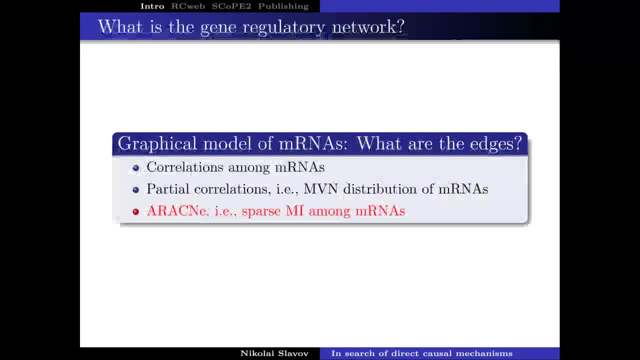 and realistic case when messenger RNAs co-variate very strongly is if they have the same transcript, if their synthesis and their degradation are regulated by the same molecules, if their transcription is induced by the same set of transcription factors, their degradation is mediated by the same set. 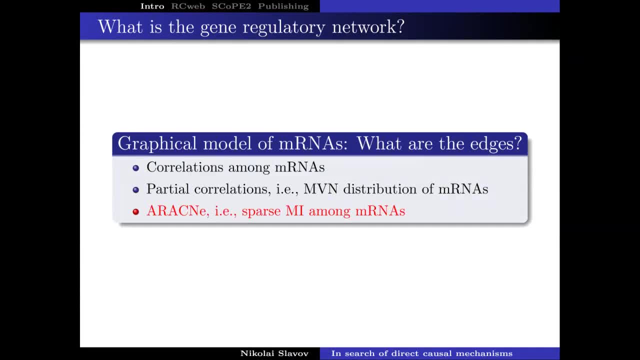 of regulators, then they're going to co-variate very strongly And finding such messenger RNAs doesn't quite correspond to our idea of finding regulators. because regulatory network? because we would like to know a molecule that is causing another molecule to do something, rather than two molecules that are both. 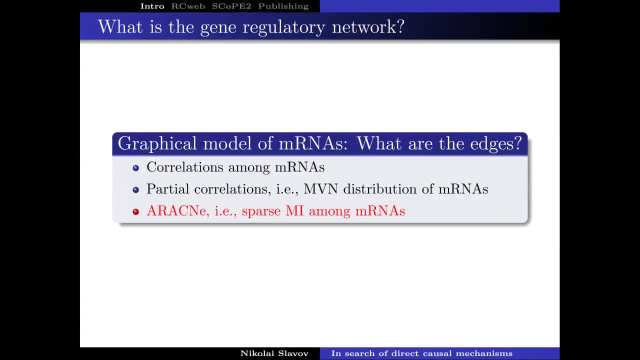 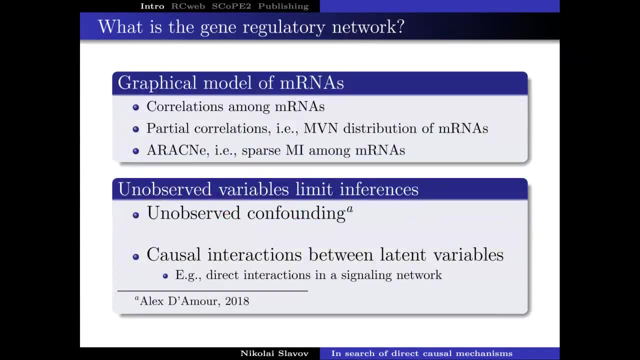 doing more or less the same, because they're listening to the same music, so to speak. And the really big elephant in the room here, when we try to infer gene regulatory networks, is that most of the really important regulators are rarely measured. They're unobserved variables, They're confounders. What do we mean by that? 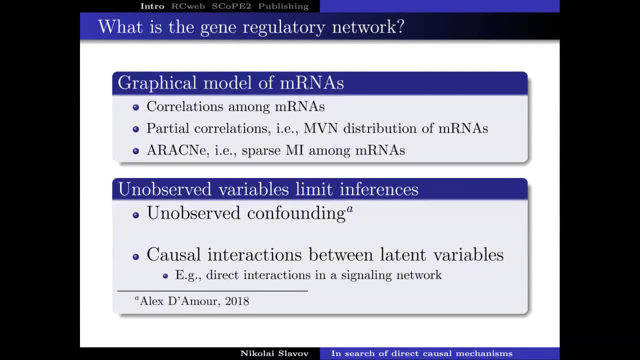 The regulation is usually not exerted directly by messenger RNAs, but by their protein. products would then get post-translationally modified and get localized to particular places. It's that active form of the regulator that is exerting the regulatory effect. So what can you do about that? My idea how to deal with it, and it's: 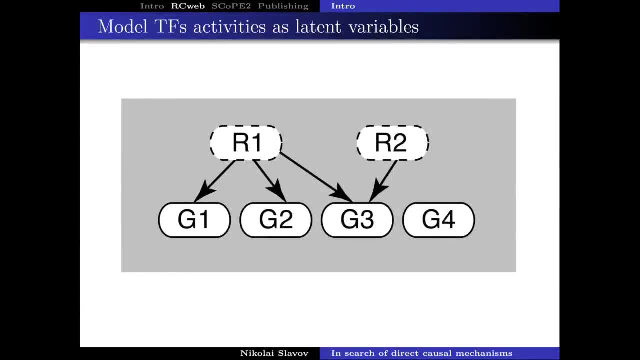 certainly not something that I invented. many, many people have worked on this problem, but the thing that really resonated with me when I was again a graduate student in your career stage, was that I'm just going to distinguish what they know from what they don't know, and I'm going to acknowledge 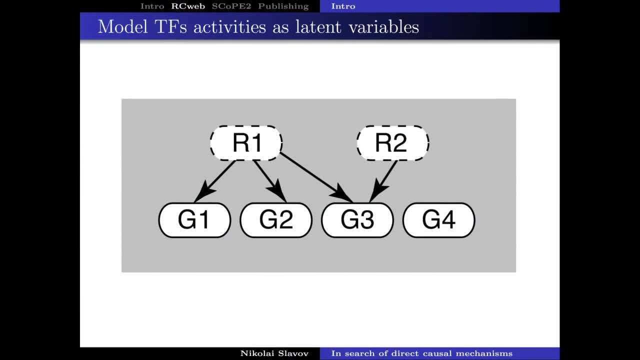 that the abundance of the messenger RNA for a transcription factor is different from the activity of that transcription factor being post-translationally modified and localized in the nucleus, which I did not know. So my idea was again- not just mine, many people's. 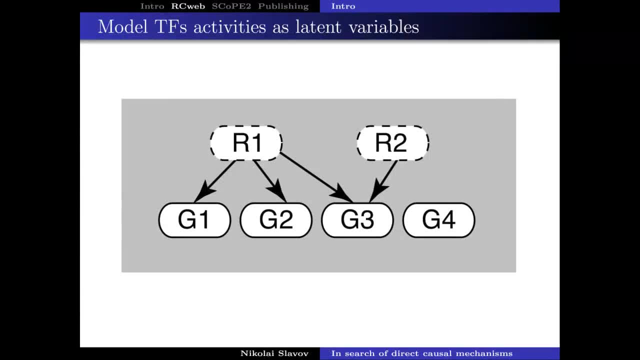 idea. the thing that I did was to model the activities of transcription factors as latent variables. So here I'm showing this very simple bipartite network where, with two layers, one layer- the bottom one- are the genes, and the top layer are 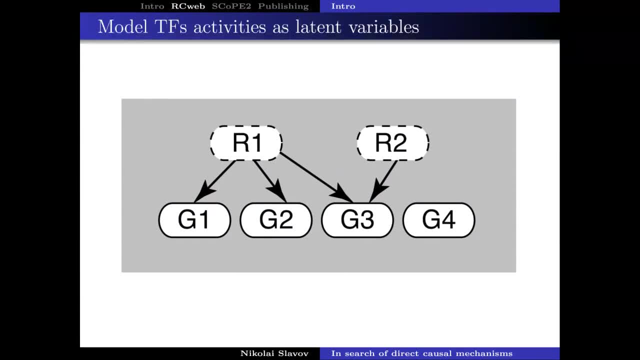 their regulators. they can be transcription factors. they can also be molecules that regulate their degradation, that regulate their abundances, and some transcription factors regulate subsets of messenger RNAs, and so on and so forth. So the idea of inferring such a network is 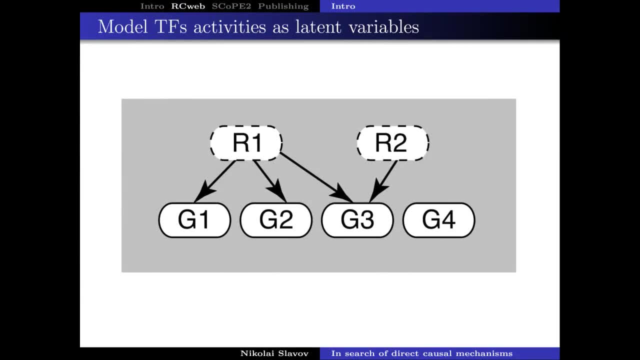 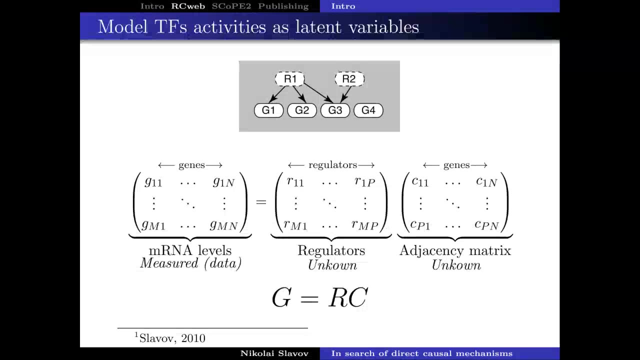 twofold: both to find which regulator regulates which subset of genes, and then to find what are the activities of that regulator. So how we might be able to do that. The thing that they did was to decompose the matrix of measured messenger RNA levels shown here. 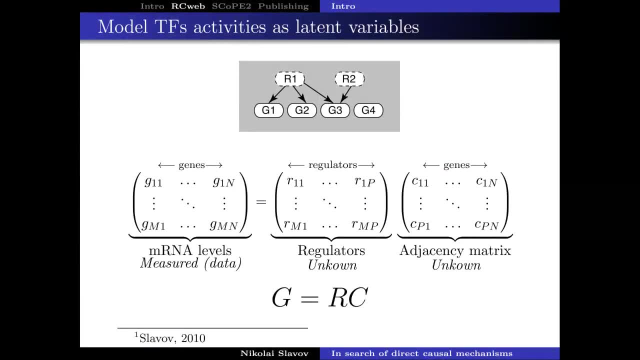 on the left, into a product of two matrices: one matrix containing the activities of the regulators- and these can be highly nonlinear functions of the actual abundances of the regulators- and to another matrix which describes the connectivity of the network, its adjacency matrix. that's the 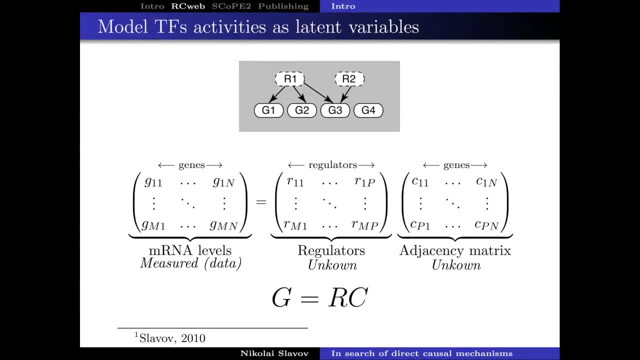 technical term used to describe the matrix that specifies the edges between the nodes of a network, And this boils down to a matrix decomposition problem. as I have written here at the bottom, G, the matrix G will be decomposed into the product of two matrices, R and C. What do 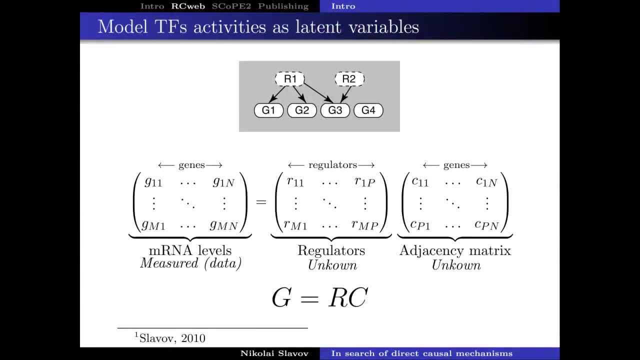 you think: does this problem have a solution, a unique solution, First, does it have a solution? and B? does it have a unique solution or does it have many solutions? What do you think? Many solutions, Exactly So this is ill-posed problem. there would be infinite number of solutions. 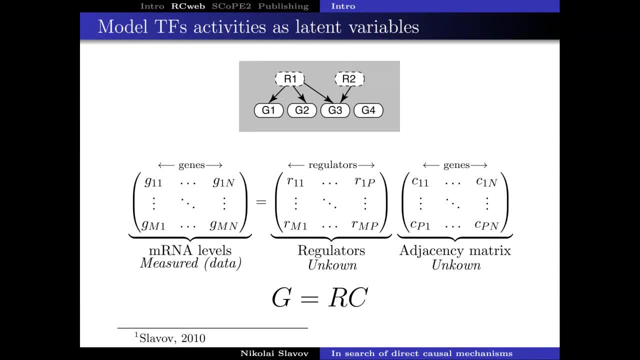 with it without knowing something more about it to constrain it. Now, what do we know about the system that we can assume because it's true rather than because it's computationally convenient to assume it. So in this case, the assumption that I felt very comfortable making is that the network is relatively 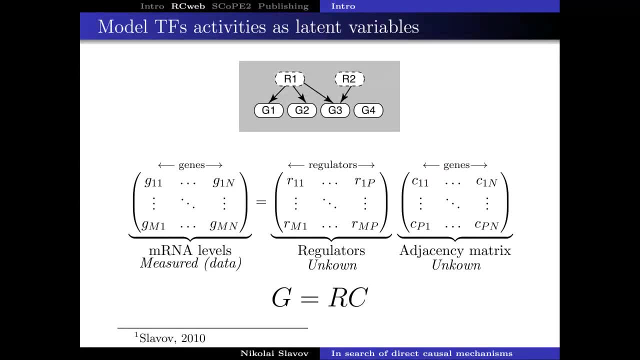 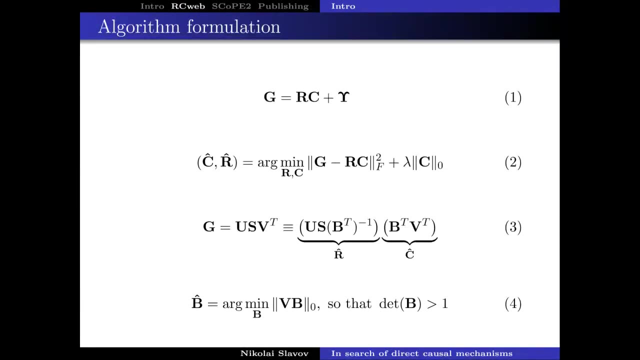 sparse, meaning that not every transcription factor regulates every messenger RNA, and we know that's generally the case. So if you make that assumption, you can. you can formulate the problem mathematically so that it becomes solvable In this particular case I 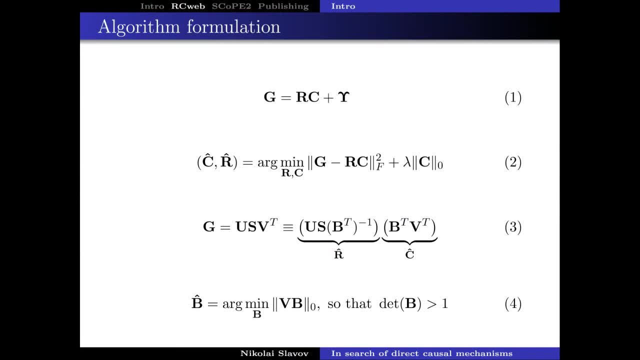 reduced the problem to finding a rotation matrix that rotates the singular value decomposition of the data in such a way that we can find both the adjacency matrix and the value decomposition of the data in such a way that we can find both the adjacency matrix and the single value decomposition. in such a way that we can find both the adjacency matrix. 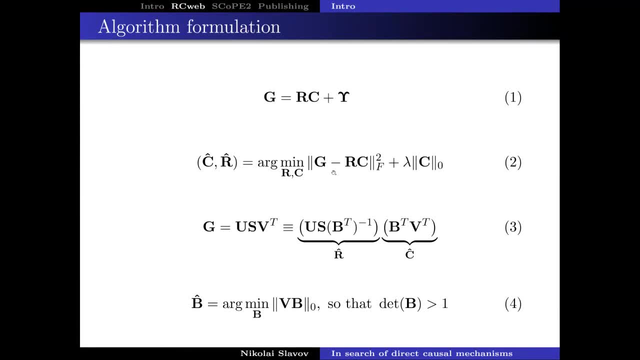 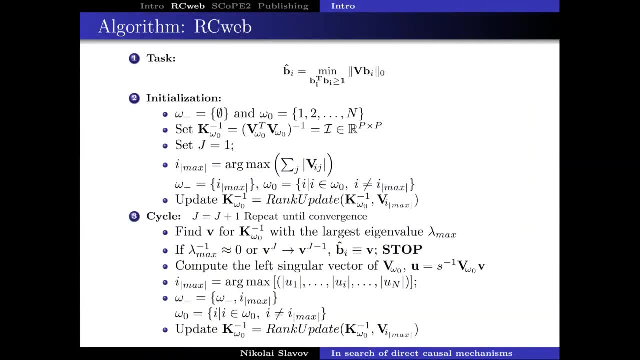 and the activities of the various regulators. This is the actual algorithm that implements it. I will not attempt to describe it for the sake of time, because it will become a little bit too technical beyond the scope of this class, but it's certainly something that is published, implemented. 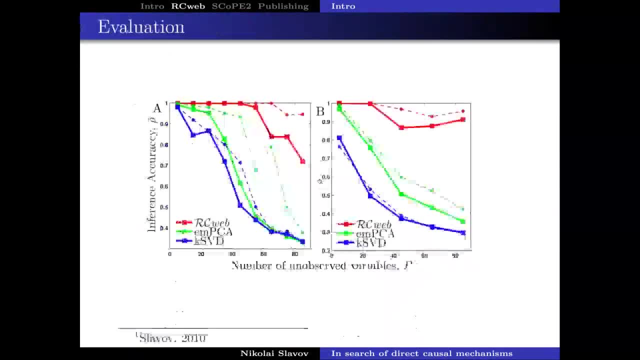 and you can read more about it if you're interested in how it works. I'm just going to show you a couple of plots of how it works. This is a demonstration of how you might be able to validate something like this. In this case, I simulated data from in-silico networks. 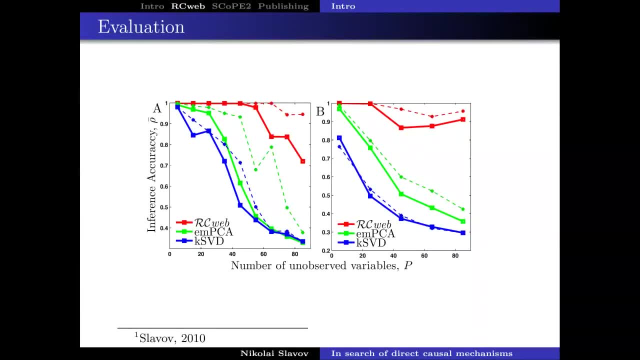 not unlike what was done in the Arachne paper. And then I used various algorithms, including this one that I developed as a graduate student- It's called RCWeb- to infer the topology of these networks, and then I correlated the inferred topology of the network. 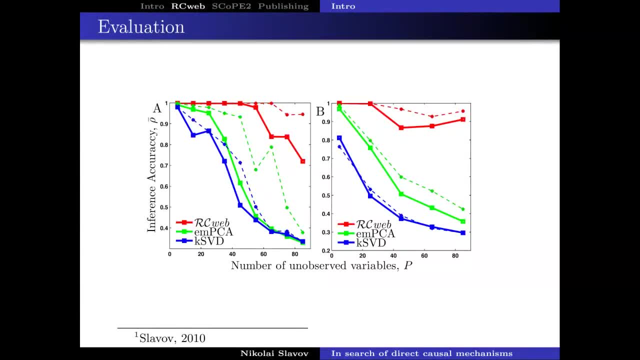 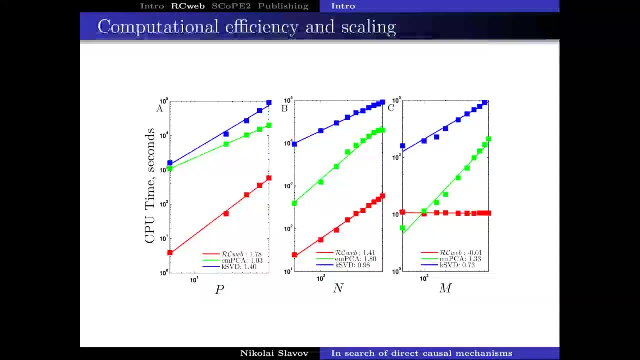 to or the actual topology that produced the data, And I found that generally, RCWeb performed better than other computing methods in terms of the accuracy of the inference and also had very favorable scaling with the complexity of the problem. So when you're developing algorithms for large-scale data, 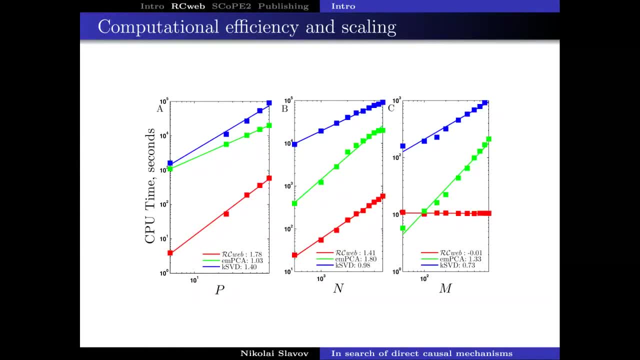 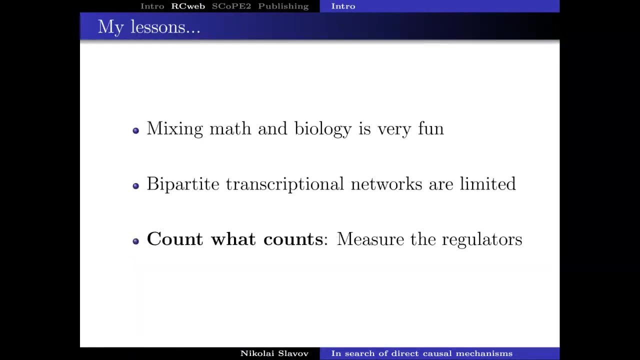 you always have to be concerned not only with their accuracy but with the ability to compute something practical with given finite computing resources, And certainly the scalability was very favorable here. So towards the end of my PhD I had concluded that quantitative approaches can be fruitful. 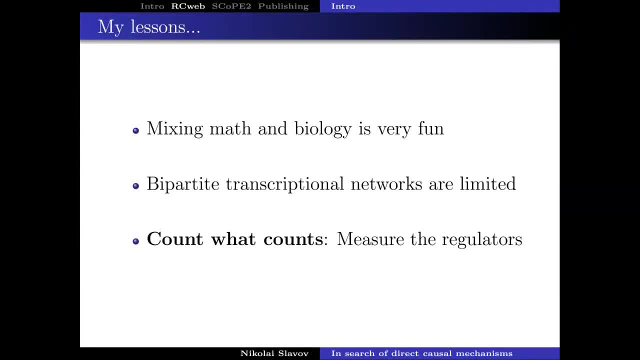 and quite fun when applied to biological systems. I was also somewhat disappointed with the limitations of bipartite transcriptional networks, And I was very interested, among other things, in measuring what's important, not just what's really convenient to measure. but can we also begin to characterize the regulators? 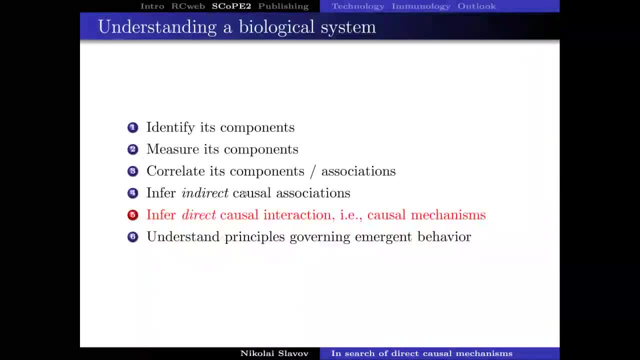 And I'm going to suggest here one of the possible ways, very difficult but perhaps possible way, how we might directly, We might just use this example as the one for causal interactions, direct causality in biological systems, And the idea is kind of simple. 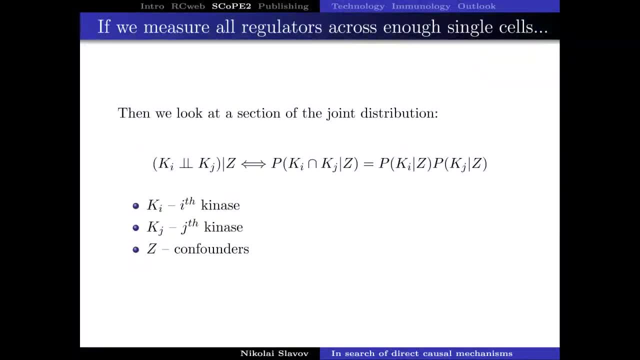 If we can observe the biological systems of interest under enough number of configurations, we might simply take the subset of cases where the only things that change are the molecules of interest. In other ways, this is subsetting the data in such a way that we have to convert the data into data. 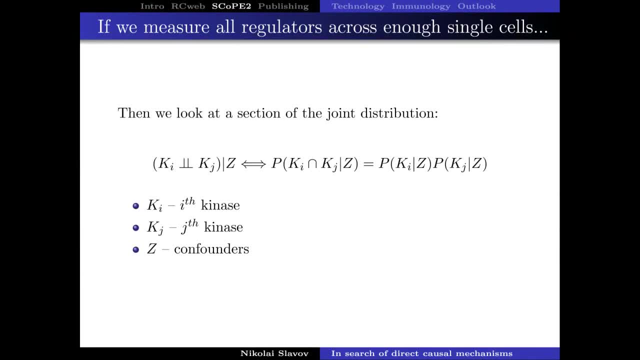 Subsetting the data into data, have the ideal controlled experiment. what do we normally do? let's say when, when, when stakes are very high and we really want to know the truth, we randomize our subjects or our samples into groups and between those those groups, we want to have only one factor that is varying, because in that 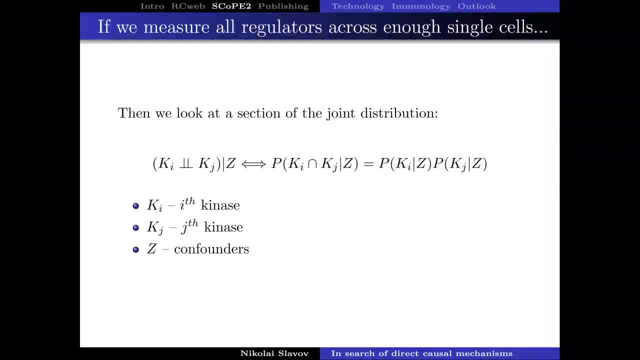 case, it is relatively simple to assign whatever differences between that we see between groups to that one factor that is different. so in this case, if we had, uh, millions of observations of the, the molecules in in cells across different configurations, we can just take the subset of those observations in which, um, everything except for the, the levels of kinase, i and j, is the same. 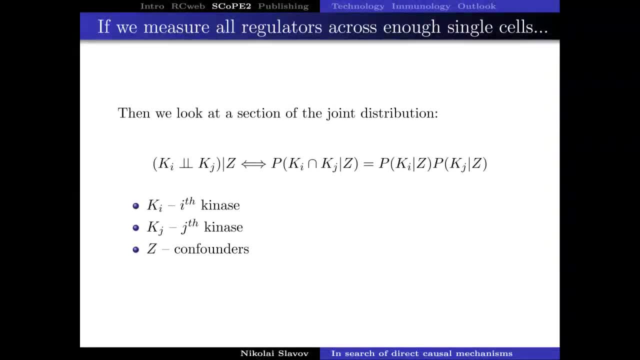 so that means that we effectively control for our confoundings, so that whatever effect they're having, that effect is going to be the same in all of the samples that you are considering, except for the sample for for the activities of kinase i and j, and then we can ask whether the joint distribution 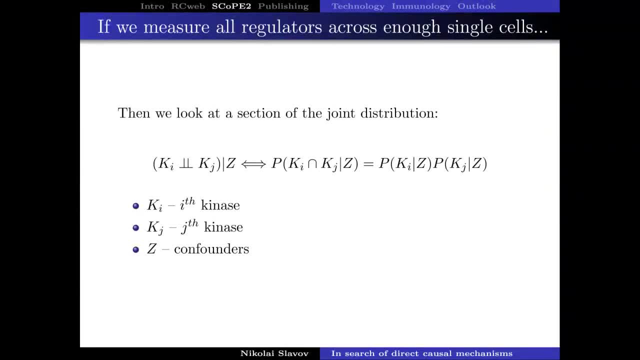 of the activities of these two kinases, i and j, is simply product of their marginal distributions, and if we could do that, then we can rigorously determine whether the kinases are actively, are directly activating, phosphorylating each other or not, without making any assumptions. so this is what the fancy math here is is describing. i try to describe. 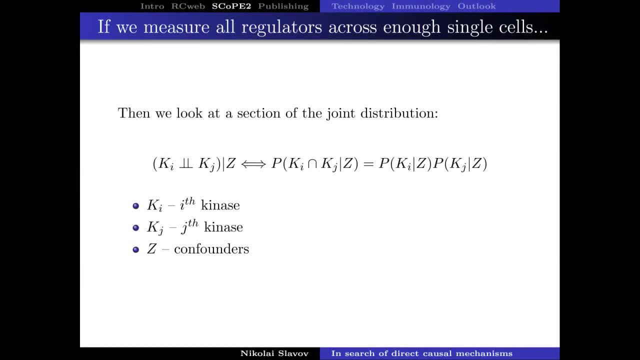 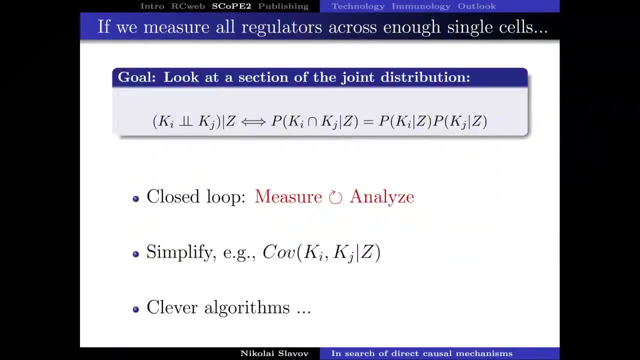 it in in plain english: uh, it's hard to do. you, you really need to have a lot of data and you need to have data that can be subsided. in that way, and instead of just taking the, the joint distributions, you may want to look at the conditions of the distribution and you may want to look at the. 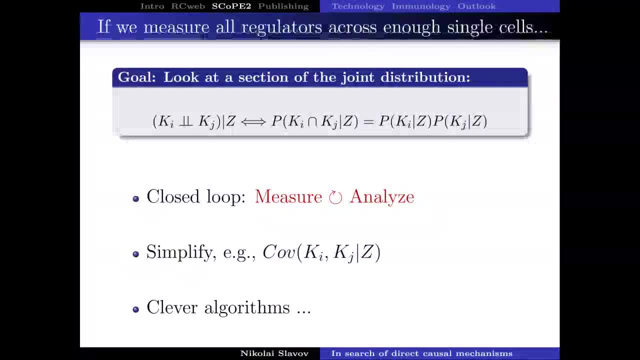 distribution of this information, and it's not just one and one-dimensional distributions, but there are additional covariances or other measures of association that might be more tractable, uh, and that to to make it more tractable again, one needs to to derive algorithms so it can be able to make this inference with limited data without uh making. 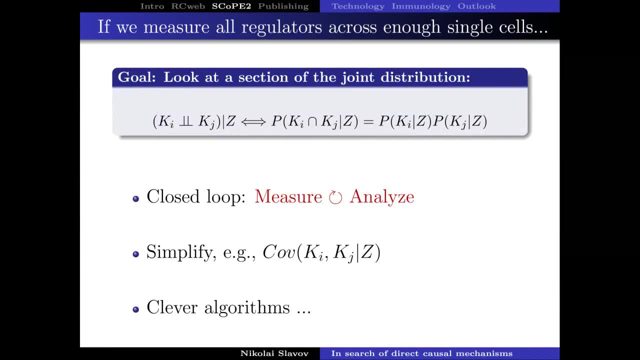 any assumptions and ideally, all of that should be done within a closed cycle where, uh, after we have done some measurements and we have learned something about the system, we have always listened to the data and we are also practicing the data in this way because we have used it a lot, but it's almost impossible to actually do the same thing we have to do in the samsung. that's the way we do it in the traditional covariance and there is number of covariants that are in the traditional covariance and there's, for instance, equivalent data, and there are also covariants that are in the traditional covariance. 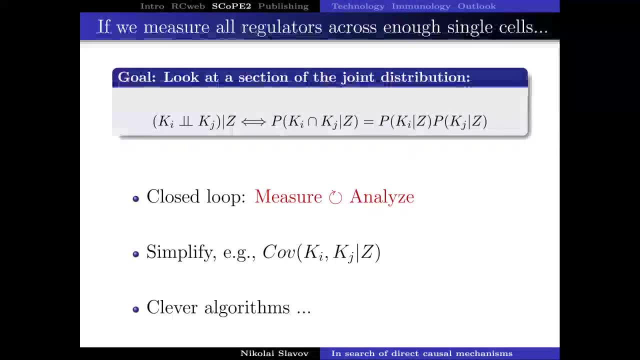 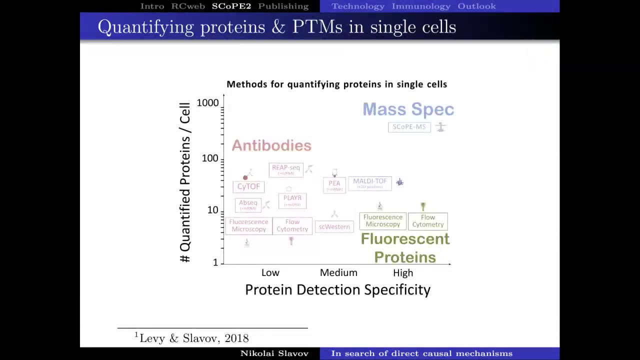 can use that knowledge to better design our next set of experiments and keep iterating until we reduce the uncertainty. So let me see how we're doing in terms of time. I think quite well. Maybe it's a good time to pause here and ask if you have questions. 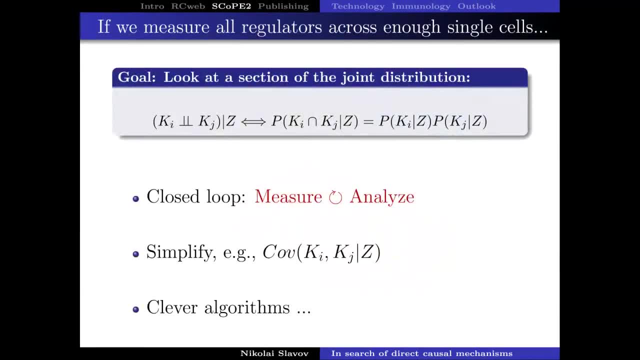 Yes, on the plot that you showed, comparing your model to other models for, I guess, inferring the connections between those different genes. the solid lines were labeled, but what were the dotted lines in that figure? The dotted lines corresponded to- let me go here. corresponded to: 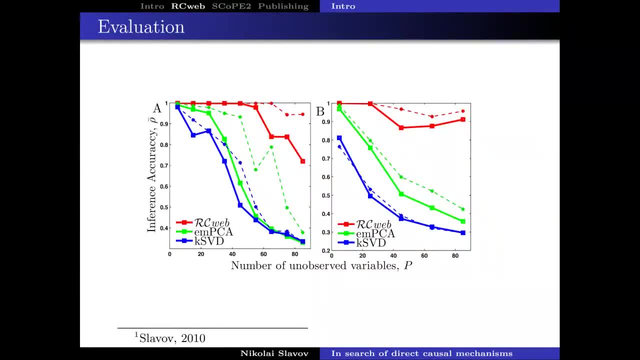 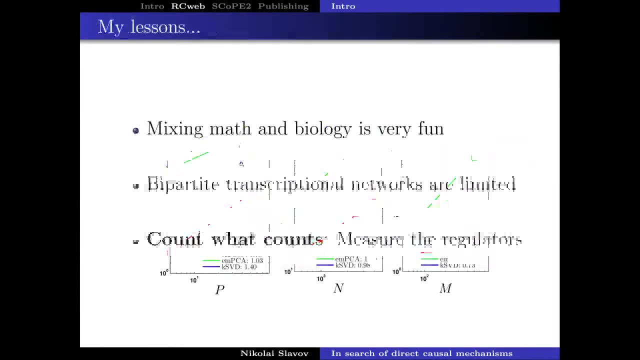 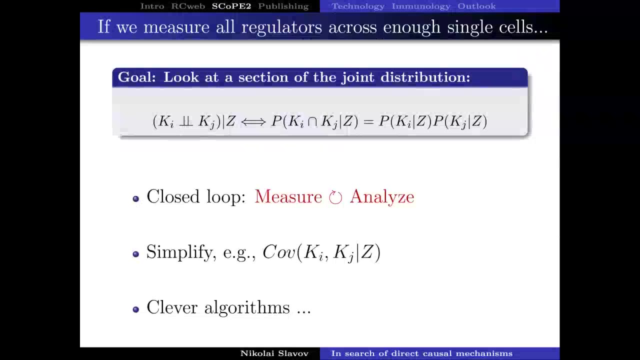 to different number of observed configurations of the data. Okay, thanks. I was wondering what kinds of computer programs are suitable for this level of analysis. You can write the code in any language that you choose, whether Python or R, or MATLAB or C. 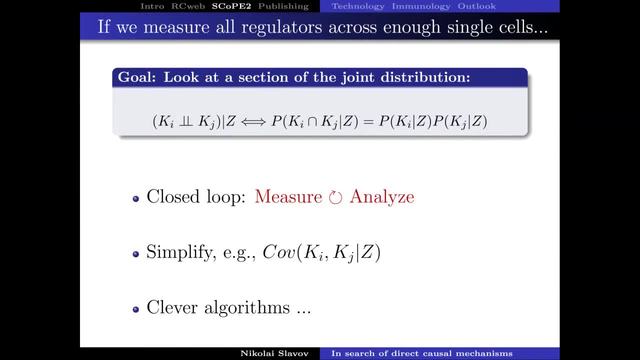 The language. it's not so important In terms of the more important thing is the algorithm. and then that algorithm can be implemented in various languages, but almost any modern language will have the capability of doing that. And then, in terms of algorithms, 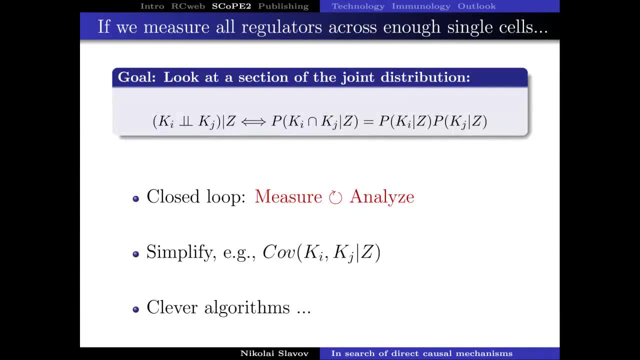 I don't think that this kind of analysis that I'm discussing here has been implemented on biological data in a particularly convincing, high-scale way, In large part, I would say, because the required data, both in terms of what is being measured and the accuracy of those measurements, have been lacking. 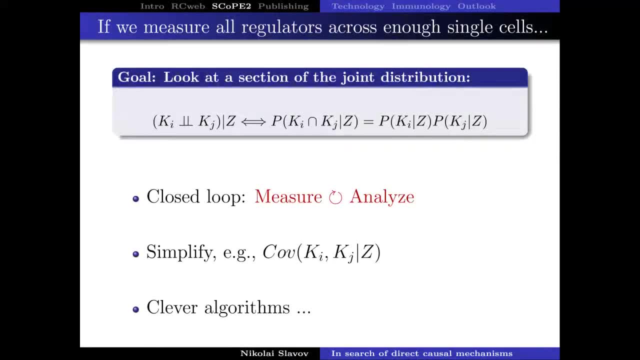 Hello Dr Slavov. I have a question. I'm just wondering. These experiments are done in cultures of cells. I wonder if the messenger RNA or the genes or whatever get affected in the body like. do people mitigate these differences? 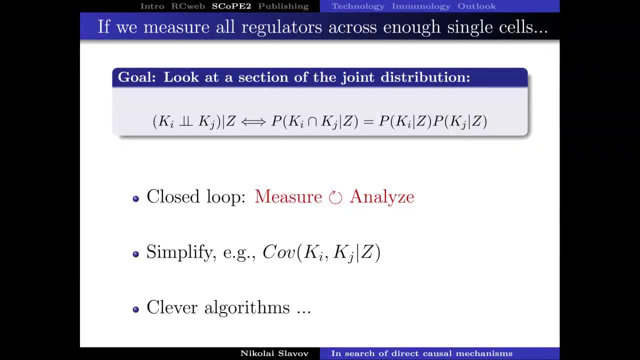 The experiments don't have to be done in cell culture. They certainly can be done with human cells extracted from humans, from patients. There is- that's not a limitation- Many oftentimes the study is easier and cheaper to do with cell culture. but none of the things. 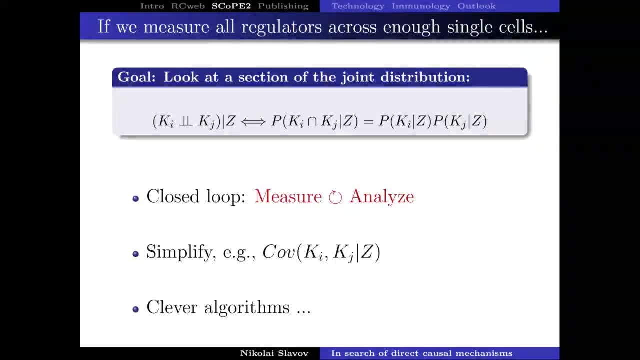 that they have said so far, or that they will say in the second part of my presentation, is limited to cell cultures. Everything can be done with human patient samples, But you still take out the cells from the human and you culture them ex vivo, right? 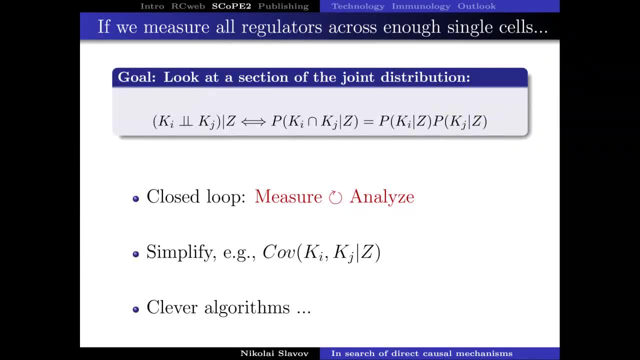 No, You don't need to culture them. Oh, okay, You just do So. the idea here will be so if you take cells, assuming here we're doing single cell analysis. so let's say you take a small biopsy from a patient. 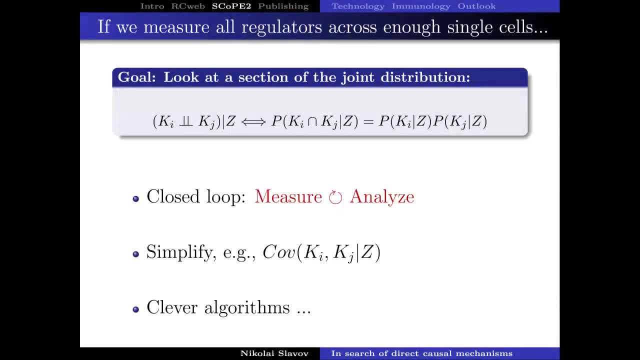 that corresponds to 10 million cells. 10 million cells is actually a tiny, tiny biopsy. If you analyze these 10 million cells at the single cell level, what you're gonna find is that each and every cell is different in some ways. 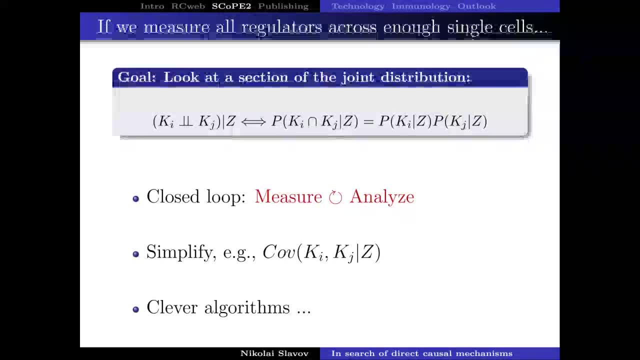 sometimes because of systematic factors. There are local environment, different signals that they receive. There would be different states and different types of cells, sometimes because of perhaps more stochastic fluctuations within these cells. But that will give you a lot of diversity and you can think of each cell being subjected. 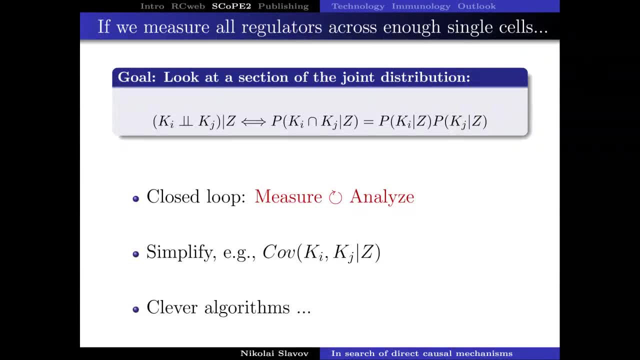 to a different kind of perturbation. You can sort of think of that heterogeneity that normally, normally exists in the human body, that exists right now in each part of my body, as a form of perturbation. And then, when the analysis that I'm describing- 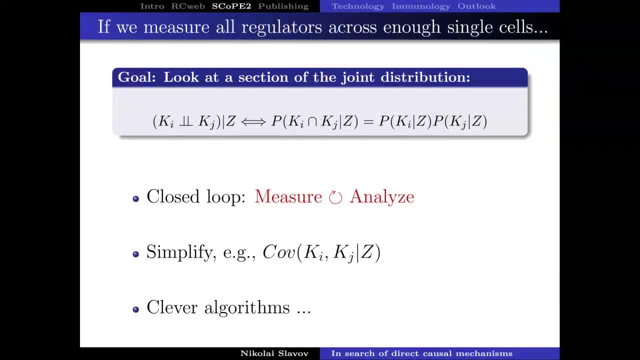 is conceptually equivalent to choosing the subset of perturbations in which the molecules under study are varying and they're changing but the other ones are not, And that gives you the ideal controlled experiment. if you could find that subset Now, that's not easy to do. 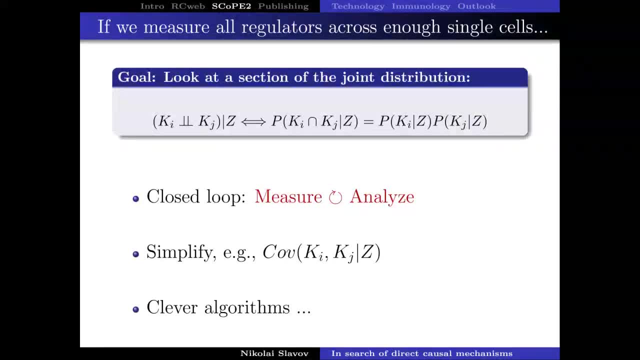 And that's not easy to do, And that's why one might have to mitigate, one might have to relax a little bit the constraints on this analysis, and there's need for very clever algorithms that can do this efficiently, But in its purest form. 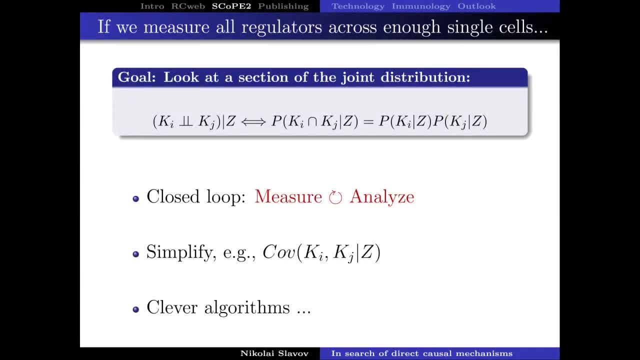 this analysis is very simple conceptually, just hard to implement, both in terms of the quality of the measurements required and the scale of those measurements. Okay, I was just wondering if just the act of taking a biopsy does that affect the cells Like I would imagine that not being like in the host. 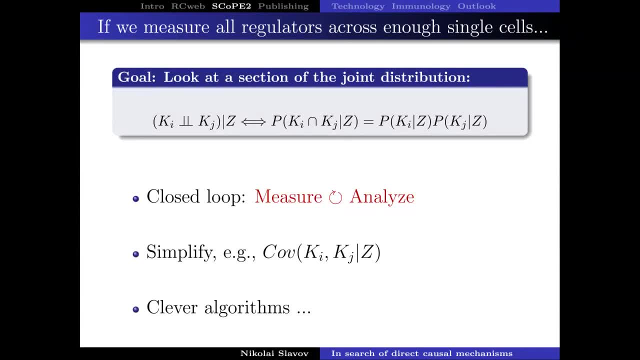 like being just grown outside of the body. that would mess up the actual representation of what happens in the body. Absolutely So if you take them out of the body and you grow them, yes, but you don't have to grow them. So what I'm suggesting is that you take a biopsy. 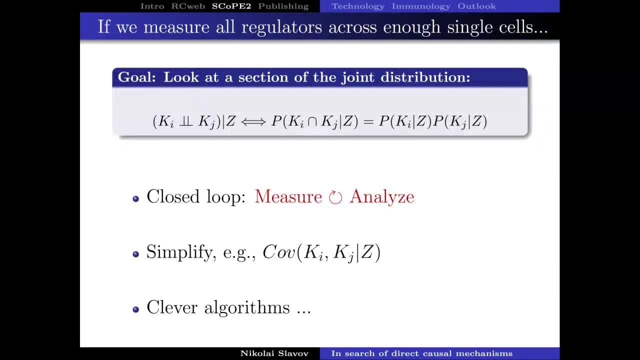 in principle, that's one of the possibilities, certainly not the only one. but you take a biopsy and then you freeze the cells for negative 80 Celsius before they have had any chance to change. That would be one approach, And now can you do that practically? 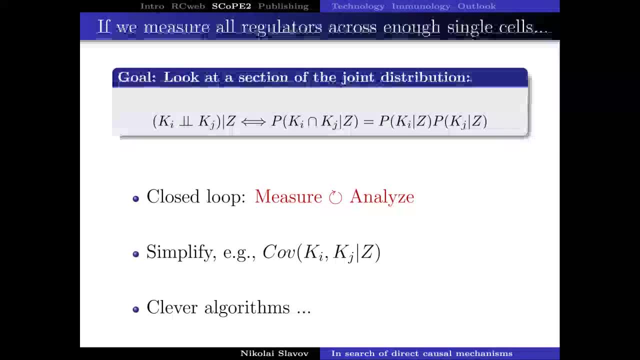 so that nothing changes. You can do your best, And will the cells change during that period? Perhaps, but the aspiration is always to decrease the magnitude of those changes, And some things may change more than other things. It is highly unlikely that the cells are going to have 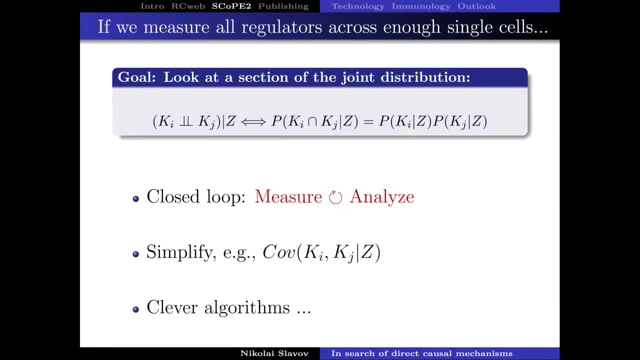 enough time and energy to degrade proteins. Protein degradation requires a substantial amount of energy and takes time to do so. Proteins are highly unlikely to change, at least in abundance, during sample collection. Their localization might change much faster. Messenger RNAs might be more susceptible. 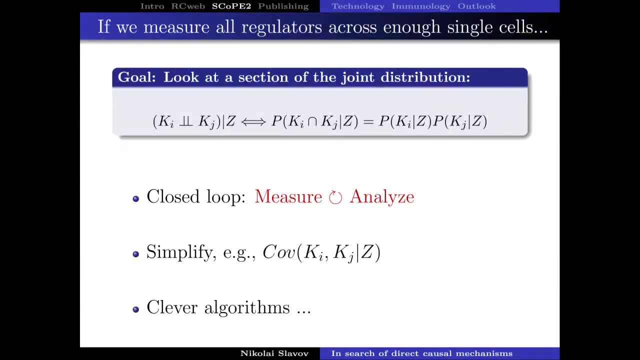 to change more quickly. But again, that's a well appreciated problem of how do you collect the samples with the least amount of artifacts- And there always are artifacts to some degree or another- But there are many clever approaches and many people who have devoted their careers and efforts. 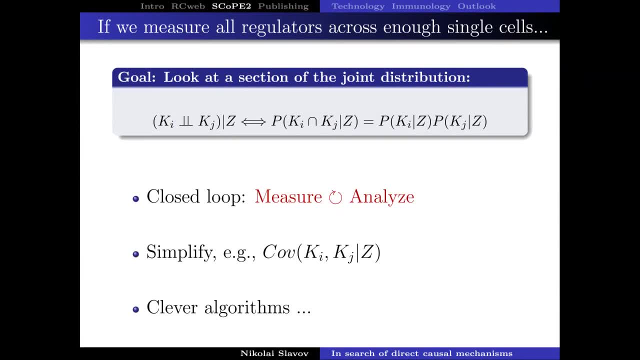 in trying to come up with ways to minimize those changes And I would say that there are good options out there, that that's not a huge problem In many cases. of course it is a problem, but it's not precluding the feasibility of fixed-tracking. useful information. 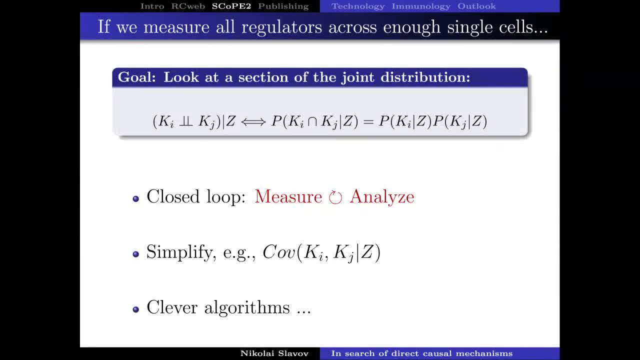 from such samples. Thank you, Hi Dr Sala. Other questions: Yeah, You mentioned that you're gonna need a very large data set for this algorithm to be effective. Is all that data collected from your lab, or are there collaborators that are also collecting that data? 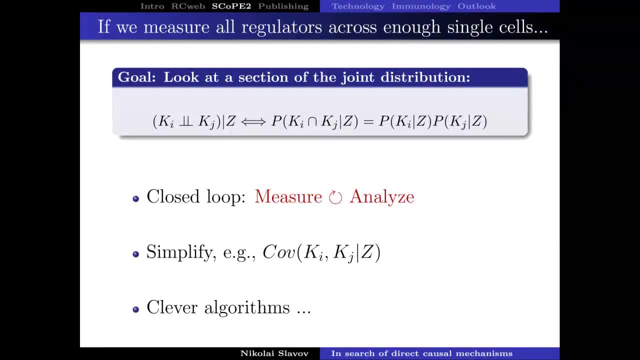 Anybody can do that. Ideally, we have that being organized. This is a global collaborative effort. I'm going to talk during the second part of my talk, my presentation about methods that we have developed to collect this data, but who uses these methods? 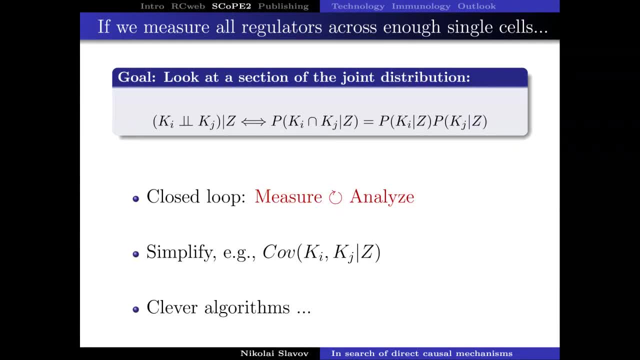 and what experimental designs, in what shape and fashion. that very much depends on resources and interest and availability And ideally, if this kind of proposal is to be successful, to be successful at a large scale, that would require that it's adopted by many groups. It's 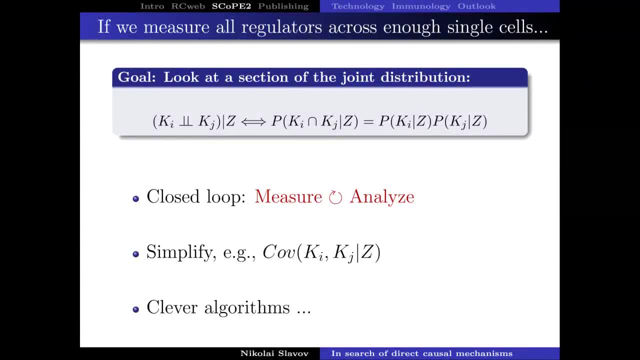 very hard to claim that somebody is successful if they're the only ones doing it. It's when you're a pioneer and you begin doing something. at the beginning, you and your group tend to be among the first doing it, But ultimately, if the thing is to become really influential, you need to be. 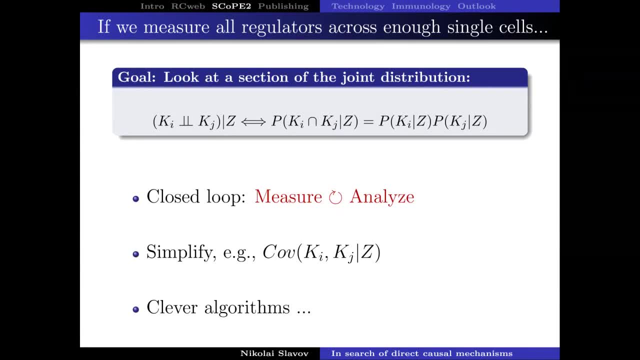 able to engage many other smart people, many other good groups in doing that, Especially if it involves large-scale data generation. that would certainly require many collaborators and lots of resources. In this case, I aim my presentation not specifically to things that we're doing in. 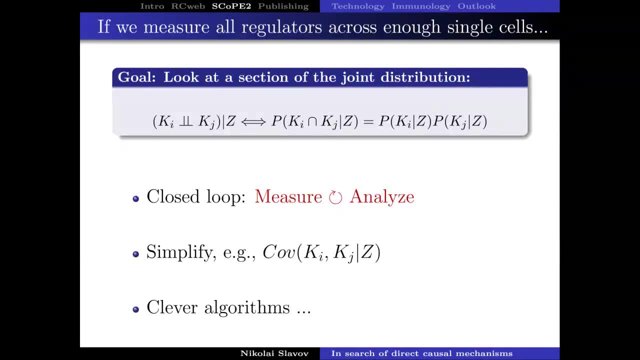 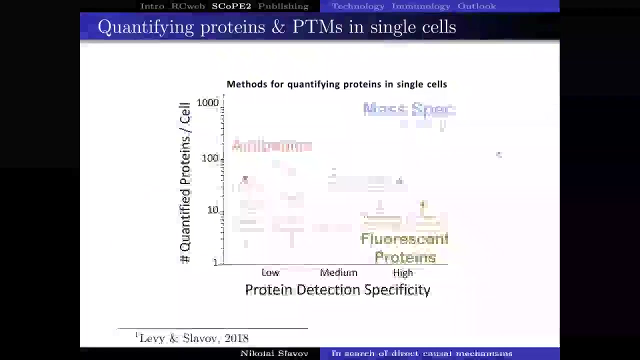 my lab, but more generally as a presentation with pedagogical purpose, to illustrate some ideas and to discuss concepts that we already covered in class. Other questions, All right. so I'm going to talk a little bit about how we might be able to measure. 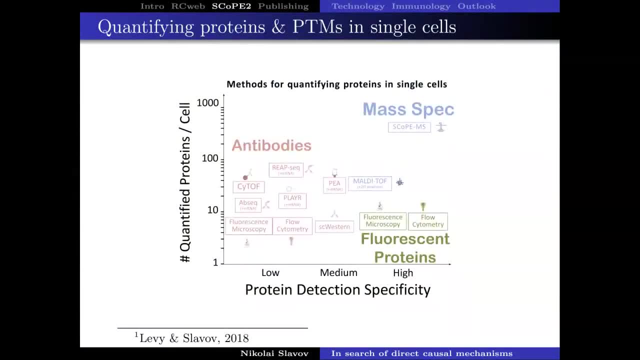 more of the variables that are usually unobserved, Specifically when it comes to measuring them in tiny samples taken from patients, such as single cells, And many of the regulators in the cell tend to be proteins, and particularly their post-translationally modified forms. So it's worthwhile considering what are the options of. 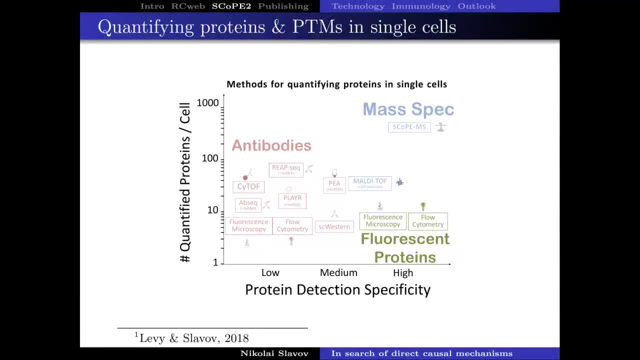 measuring them. For many decades, the only methods that could measure proteins in single cells, in the main methods relied on antibodies, But antibodies tend to have- many of them tend to have- limited specificity, in the sense that antibody recognizes a particular epitope and that epitope might be. 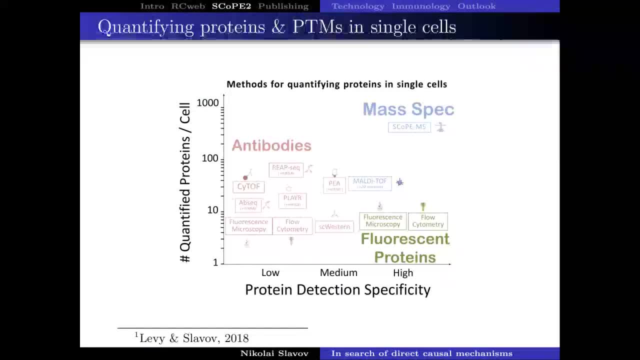 present in other proteins as well. Or it could be that the antibody recognizes other epitopes as well, and especially if these other epitopes are present in very abundant proteins, the specificity of that antibody can be compromised. So what's the best way to measure the number of antibodies? 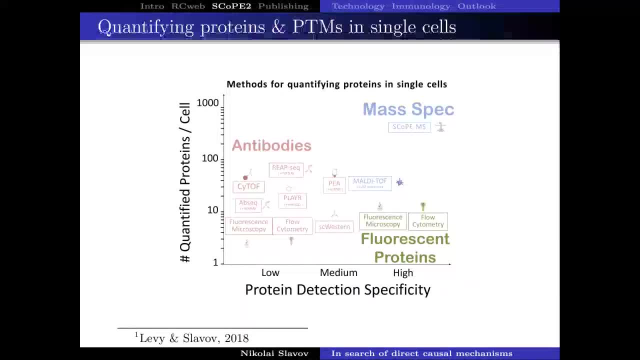 The other weaknesses. the other major weakness of antibody-based methods is that they have failed to scale to analyzing multiple proteins per sample. After decades of work, we can still measure a few dozens, maybe up to 100 proteins per sample, but not more than that, And I was 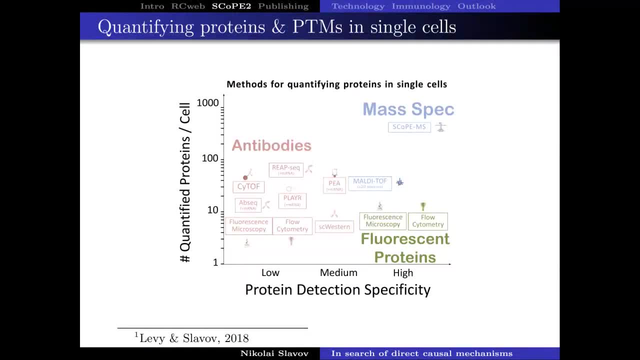 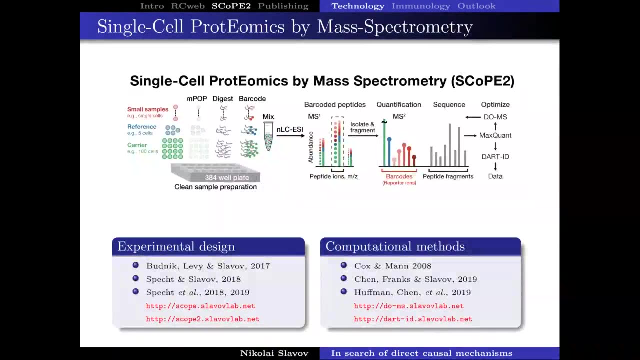 interested when I started my group at Northeastern 2015 in developing mass spec approaches to be able to make such measurements in single cells, And here I summarize the methods that we have developed in a single slide that they can usually spend an hour explaining, But I'll summarize. 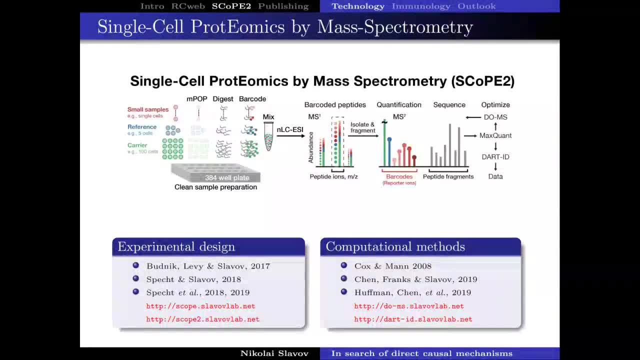 in very conceptual terms. First, we need to somehow isolate the single cells, and this isolation can be done by a variety of methods. The one that is most practical in most cases is by fact sorting them. In fact, it's really hard to imagine how a single cell would be able to do it, And in fact, 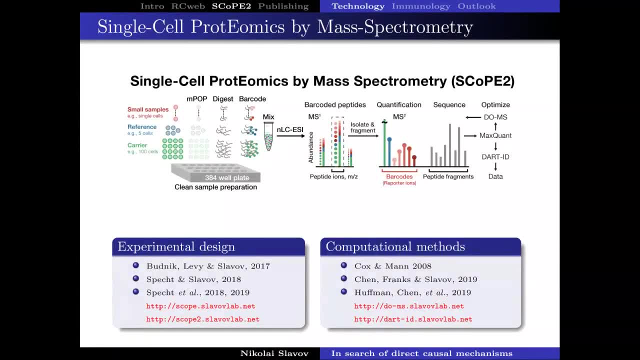 it's hard to imagine how a single cell would be able to do it, And in fact it's really hard to imagine how. into a multi-well plate again. there are many, many other possibilities. and then we needed to develop methods for preparing the samples in tiny volumes, conventionally samples for mass spectrometry. 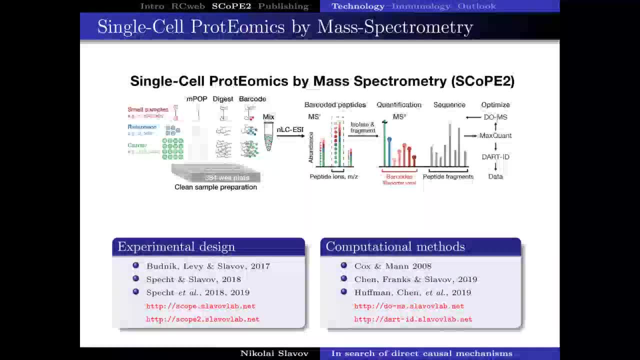 analysis are lies using chemicals that are incompatible with the mass spec analysis itself. so they have to be removed, and if you try to remove chemicals from tiny samples, you tend to lose the, the proteins from these tiny samples. so we came up with methods that don't require. 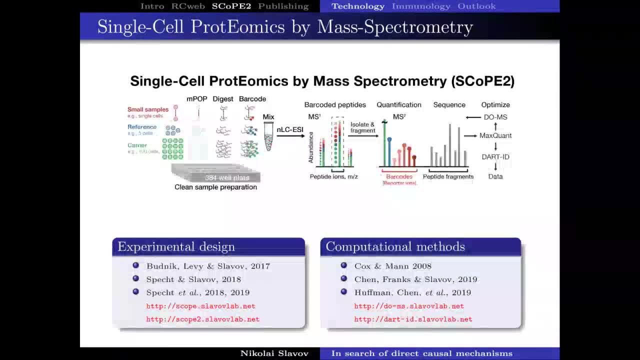 these samples to be cleaned up and whose volume can be miniaturized. and then the proteins are usually digested to peptides, because peptides are easier to analyze by mass spectrometry. then the peptides are labeled with barcodes, and these barcodes covalently label each peptide and 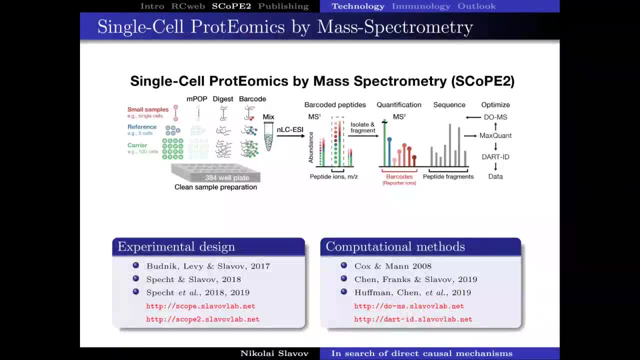 if we use one barcode per single cell, then every peptide from that single cell gets the same barcode. once they're labeled, they can be mixed, and we also mix them with sample that is comprised of larger number of cells, because that helps to reduce losses from proteins adhering on various surfaces. after that, the mixed barcode samples are separated. 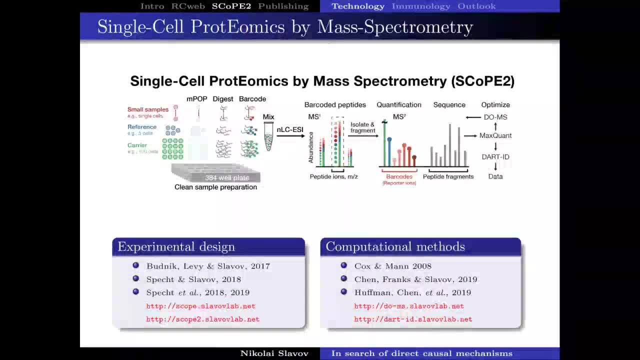 on chromatography. the reason why we do that is because if we inject the peptides from a group, from mammalian samples, from mammalian cells into a mass spec instrument, there will be millions of ions detected and we, the instrument, will not be fast enough to analyze these ions and determine what are the peptide sequences, what do they correspond to, and so on. 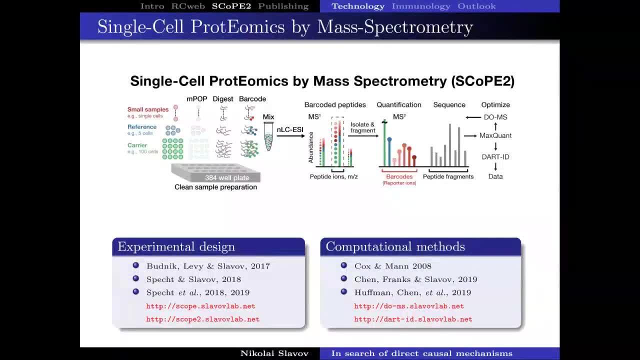 so to reduce the complexity of what the instrument says, we have to use various methods to separate the peptides so that we have fewer peptides entering the instrument. at the same time made our machines worse, and so on. and of course, what actually enters the instrument are ions, because mass spectrometry works with ions rather than molecules. 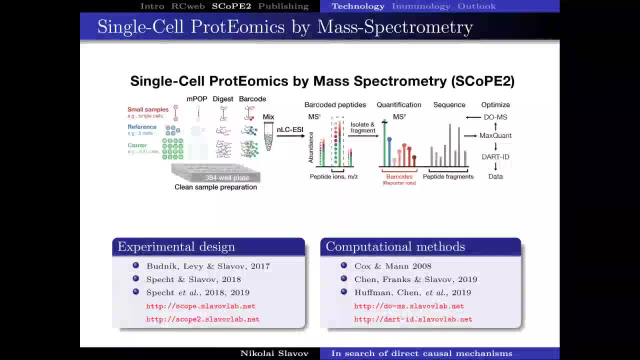 and then the technology allows to see all of the peptides that have the same sequence- and i've received those barcodes- the peptides with the same sequence that come from different single cells who correspond to a particular iod cluster that then can be isolated in such a way that the barcodes become distinguishable and can be used to quantify. 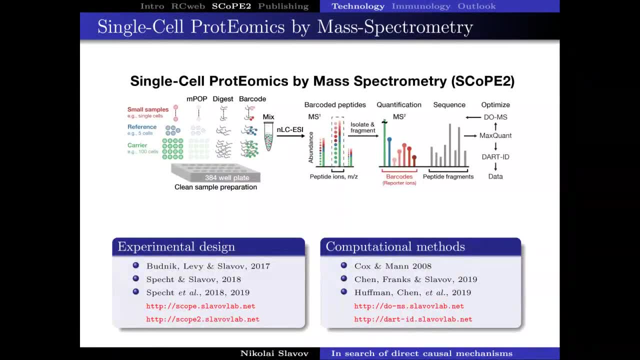 the abundance of that particular peptide across all of the single cells analyzed and the peptide fragments can be used to determine what is the sequence of the peptide. so that's the the big picture, how the experimental design works, and there have been essential computational aspects to optimizing both the the many parameters that go into. 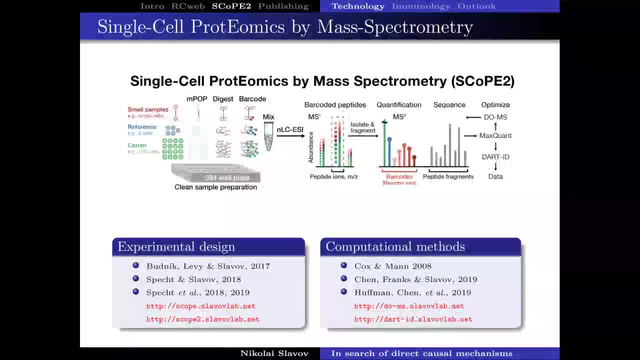 controlling the acquisition of these data, and also computational methods to enhance our ability to identify the peptide sequences by using additional information such as the retention time of the peptides, and to further be able to interpret the data. are there any questions? on the big picture, this is, ashley. what exactly do you mean by like? what is? what does barcoding the 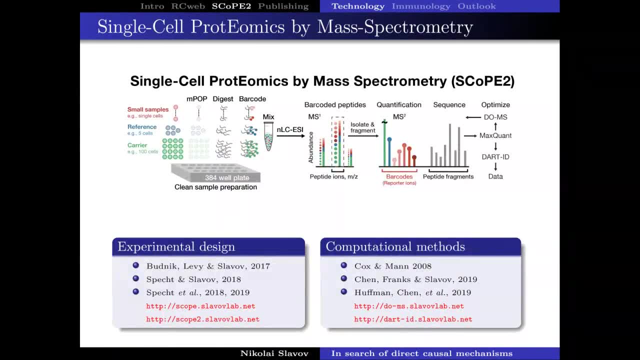 sample mean. so the barcoding is done by uh molecules that are known as isobaric mass tags and- and just for everybody else to explain this, isobaric. isobaric meaning they have the same mass. so even though we have different tags, all of these tags have the same molecular weight. 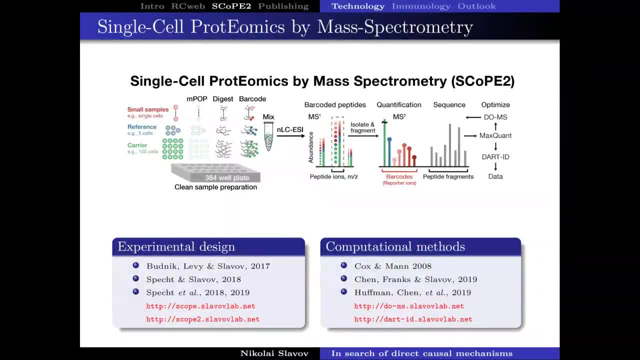 and because they have the same molecular weight. when we attach the different tags to the same peptide sequence, we end up with molecules having the same mass. therefore they appear as a single cluster during as they enter the mass spec instrument during the first scan, but when broken they break in distinct ways the different tags and then we can distinguish. 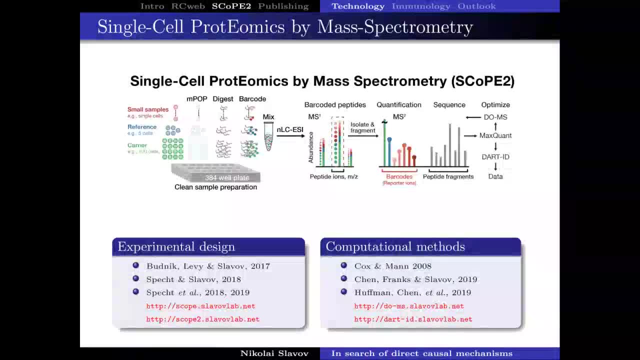 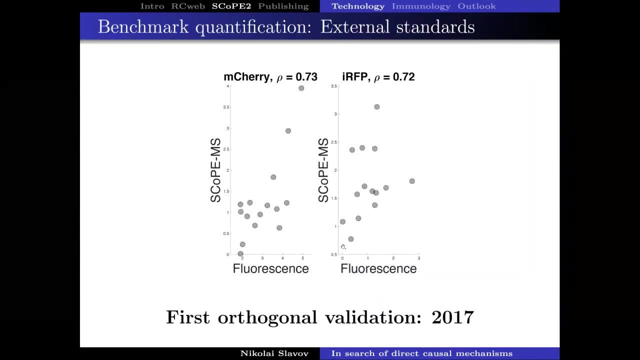 them and quantify them separately. yeah, that helps. thank you, other questions? all right, so does it work? all of this is, uh, the beginning. the beginning efforts were actually done by co-op students at northeastern- undergraduate students, and these data are produced by undergraduate co-ops students at northeastern. so if you have something new, 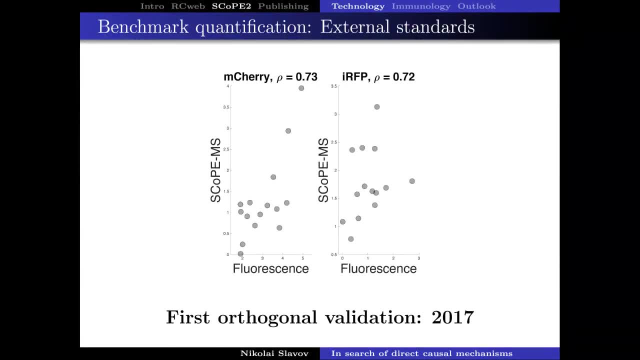 you always want to test it and see whether it makes sense or not, and ideally you don't test it by seeing how reproducible it is, because you can have perfectly reproducible artifacts. reproducibility and accuracy are very different things. it's good to have reproducible things, but 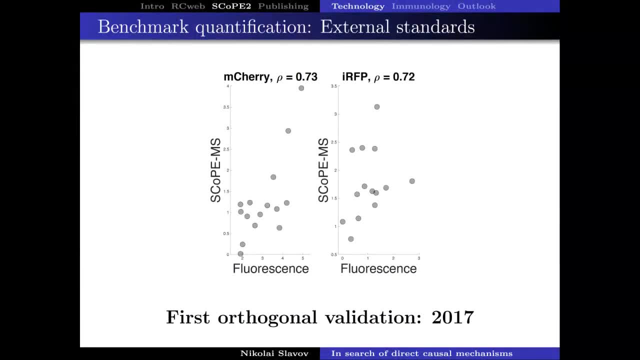 reproducible. things can be wrong. so in this case we wanted to test it with something orthogonal and something orthogonal as a method to measure proteins in single cells reliably, without the issue of low specificity and so on and so forth, is to measure fluorescence from fluorescent proteins. so in this case we had m cherry and irfp infrared fluorescent protein being expressed in. 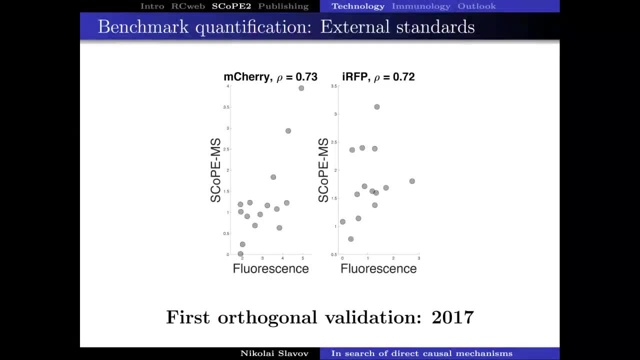 mammalian cell line. these were breast cancer cells. so uh, we could measure the fluorescence on a fax sorter. and then the sorted cells were also analyzed by uh scope ms at the time a few years ago, and we found that the two measurements correlated. so that gave us confidence that we might be able to further improve the method and get quantitative. 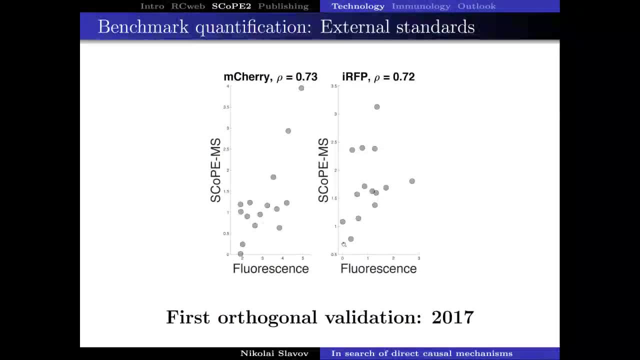 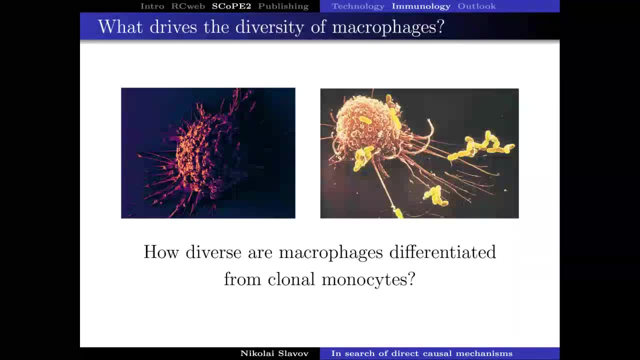 data from it. um, and i'm going to tell you about um more about the application of this method in the context of a study that i'm going to be doing in the next couple of years, and i'm going to tell you about um more about the application of this method in the context of a study that 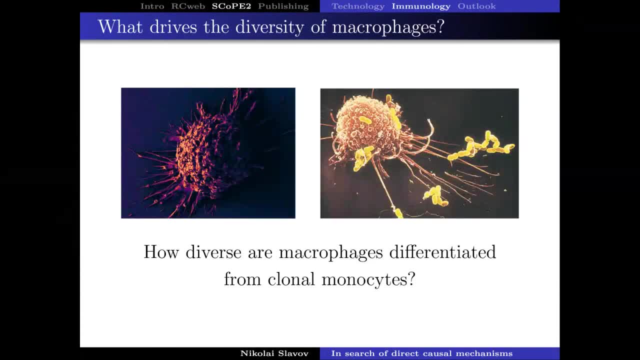 uh, a graduate student in my group led harrison speck, and that study started with a very simple question as to the determinants of macrophage polarization. macrophages are cells of the innate immune system, as we have actually discussed a number of times during our class that they're 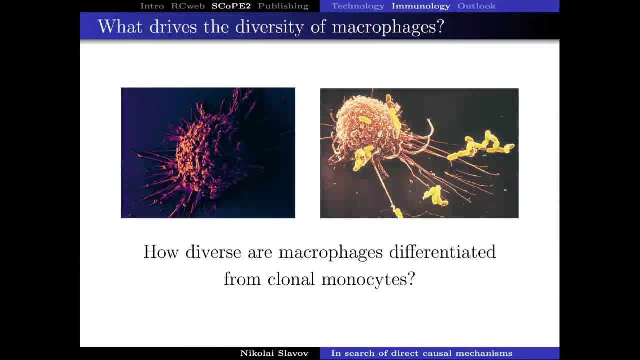 present in most tissues in your bodies, and what is remarkable about macrophages is that they tend to have many different types of macrophages. they tend to have many different types of macrophages. they tend to have many different guises. uh, what do we mean by that? they can, depending on various cytokines present and 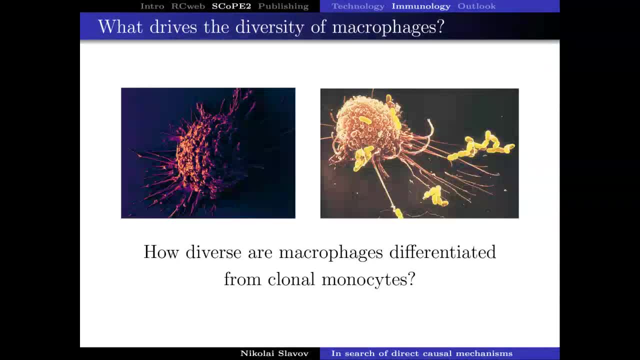 the extracellular matrix and other cues from the environment. they can have different phenotypes, molecular and functional properties. for example, some macrophages can be pro-inflammatory- they stimulate the immune system, they attack and eat bacteria, while other macrophages are exactly the opposite: they tend to be anti-inflammatory and they might repress the 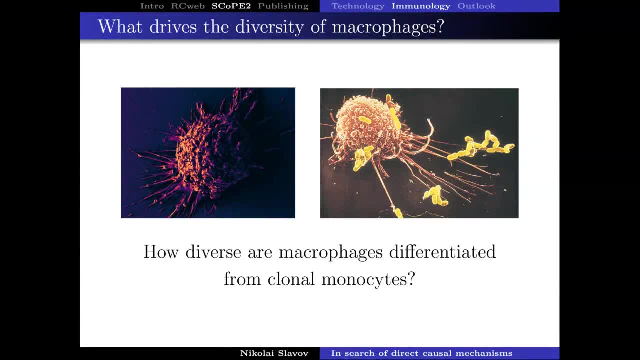 immune response, and both of these functions can be very functional in the context of of of health and macrophages performing their functions in the organism. the pro-inflammatory one is obviously associated with the immune response and responding to various types of infections. it's performed by macrophages that are classically called m1 macrophages, for m1- polarized macrophages. 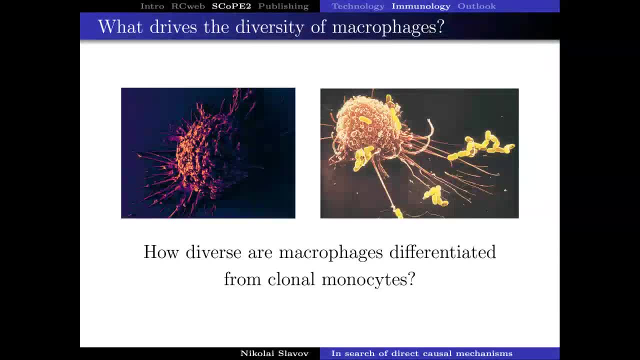 and the other function can be very important in preventing autoimmune diseases such as arthritis. macrophages can prevent the immune system from inappropriately attacking the cells of the host, your own organism. but of course that function, the immunosuppressive function, can be uh usurped by cancer cells and it is commonly one of the mechanisms that cancer uses to evade. 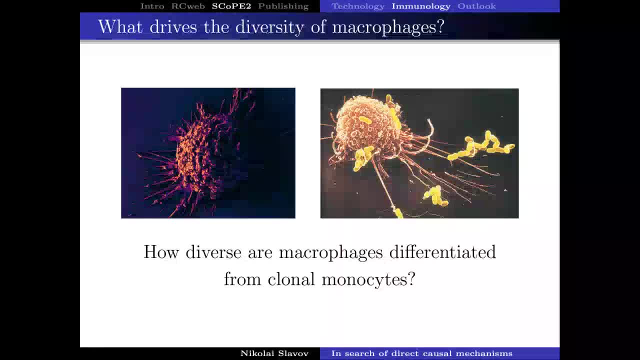 the immune system by surrounding itself with such inhibitory macrophages that help suppress the immune response and prevent immune cells from reading the body from the cancer. so the question that we wanted to answer is whether macrophages um have the inherent propensity to become polarized. 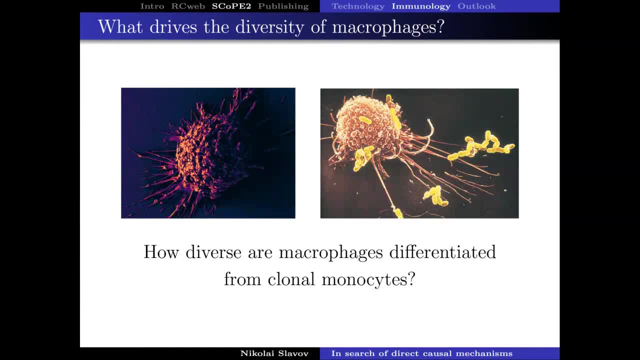 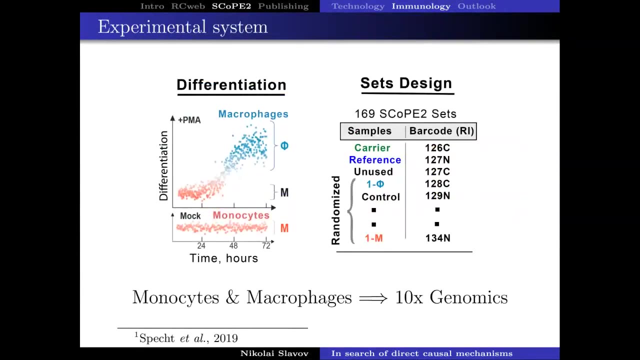 whether they can get polarized if we don't provide cytokines or if we differentiate them in vitro. in the absence of cytokines, they might still show a degree of polarization. so to address this question, we did an inventory differentiation experiment from a cell line by adding a chemical pma in this. 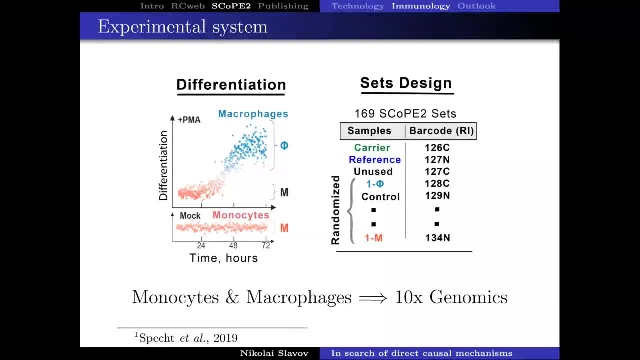 case uh, the mono to a monocytic cell line. the monocytes differentiated in the course of 72 hours, and then these macrophage-like cells were analyzed both by single cell mass spectrometry and by 10x genomics, which is one of the very powerful high throughput methods for single cell rna. 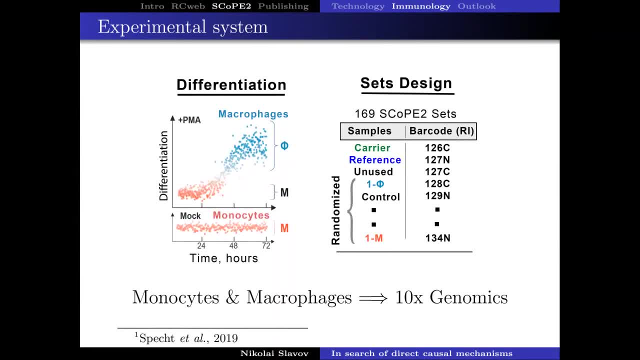 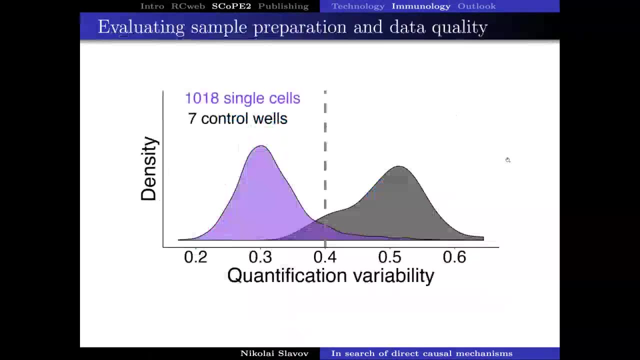 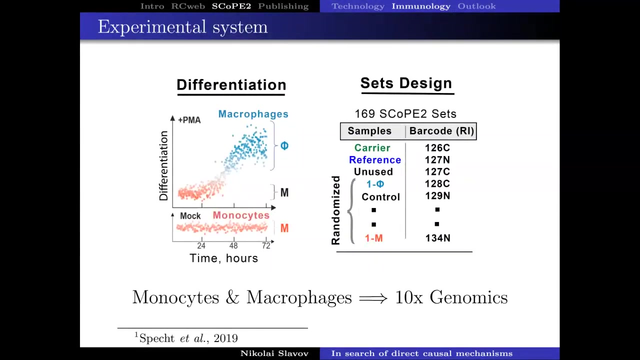 sequencing. it's a commercialized version of of dropsyc that was developed by the Harvard Medical School and the Broad Institute a few years ago. um, i'm going to let me see how are we doing in terms of time. we have time so we can explain the design. so, as i say previously mentioned, each single cell will get its own barcode. 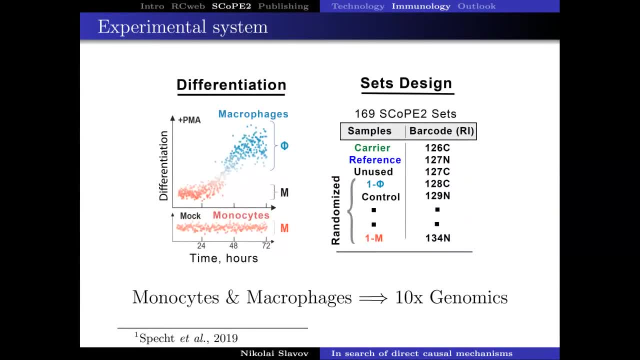 that then can be used to quantify independently the, the protein abundances, the- the sorted single cells were labeled with these barcodes, as shown here in the table, and, in addition, each set contained the reference sample that was used to to be able to integrate data from multiple scope to sets into into the same matrix and contain the- the carrier. 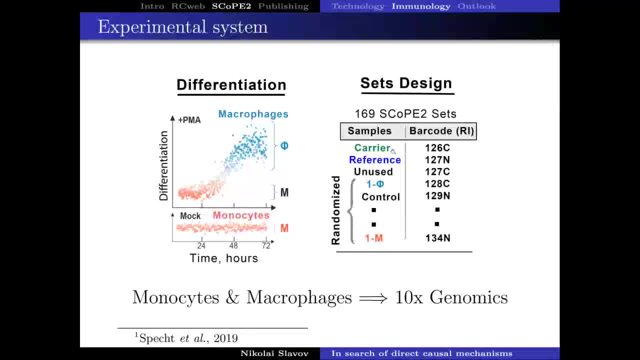 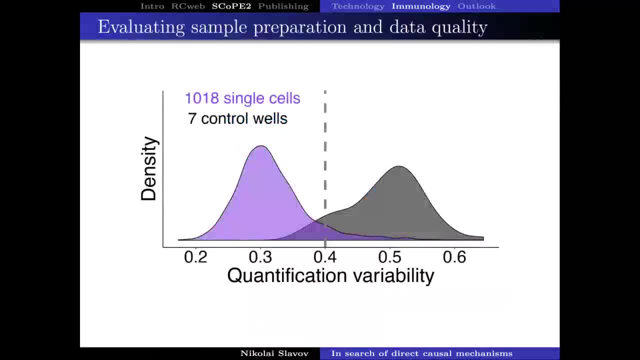 sample comprised of 200 mixed cells, monocytes and macrophages. that facilitates the analysis by mass, and the first time you get data you should always question the quality of that data. so we spent much time thinking about metrics that might indicate whether the data are useful for analysis and indicate possible problems in the data and 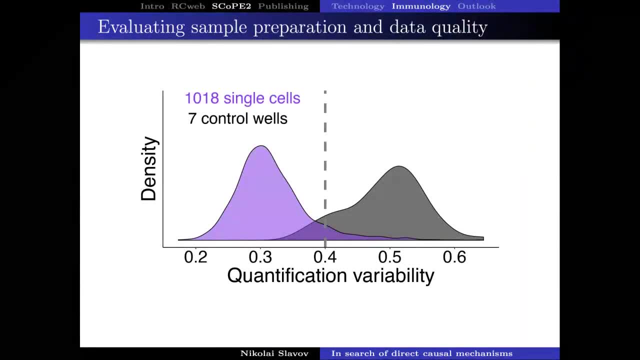 one well well validated and widely used method to evaluate protein measurements by mass spectrometry is the degree to which different peptides originating from the same protein provide consistent quantitation. so if we have different peptides that originate from the same protein, they should change in a similar way between different single cells. 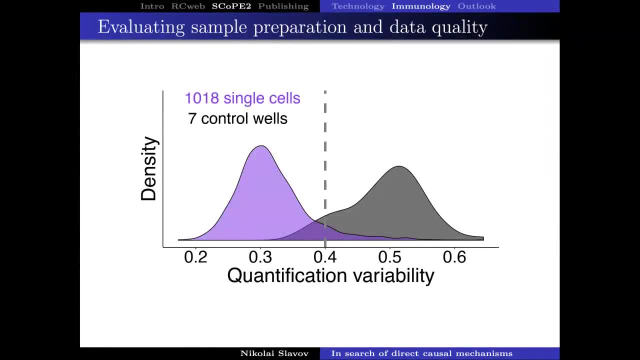 and we can quantify that variability by computing a coefficient of variation. that's a normalized measure of their variability and what we can see here is the quantification: variability tends to be lower for the single cells compared to control wells, and the control wells are wells that received all experimental treatment that single cells did. but 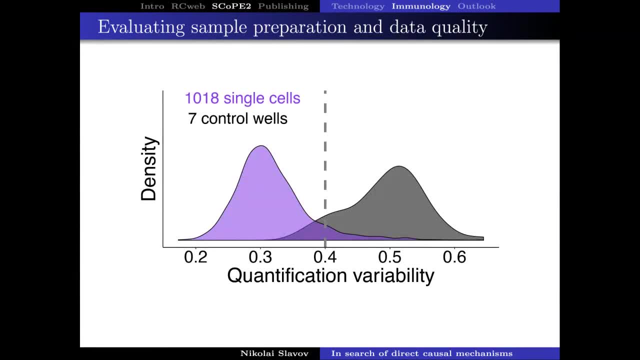 they did not receive a single cell and, based on this analysis and other types of quality control analysis, we were able to establish that most of the single cells processed through the pipeline were suitable for further analysis, while a few of them appeared to to have too noisy data or to have failed for whatever reason. and that's the 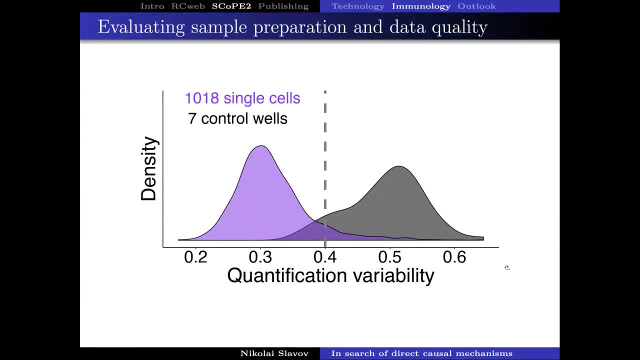 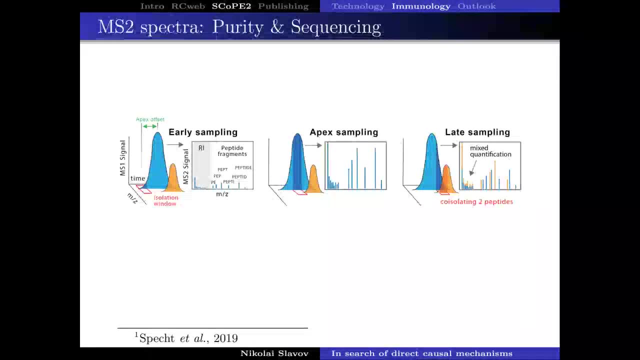 magenta tail of the distribution and they were discarded from further analysis. one very important aspect that we had to improve in this analysis will be illustrated here with with these cartoons, and that has to do with the efficiency of sampling peptides by mass spectrometry. so i already mentioned in the in in the introductory slide that the barcoded peptides 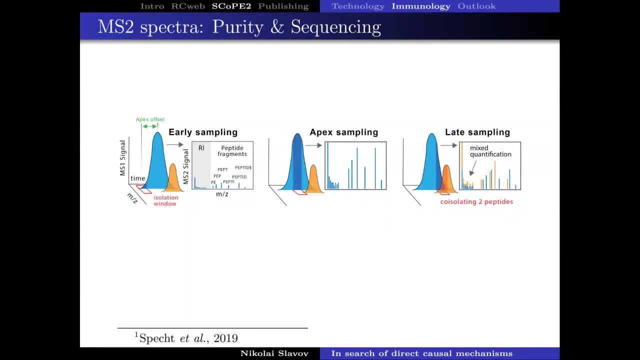 are separated by chromatography before they're analyzed from by mass, by mass spec, and each peptide elutes from the chromatographic column over a period of at least a few seconds, and that elution peak here is being drawn as this, um uh, as these curves colored in in blue or orange. 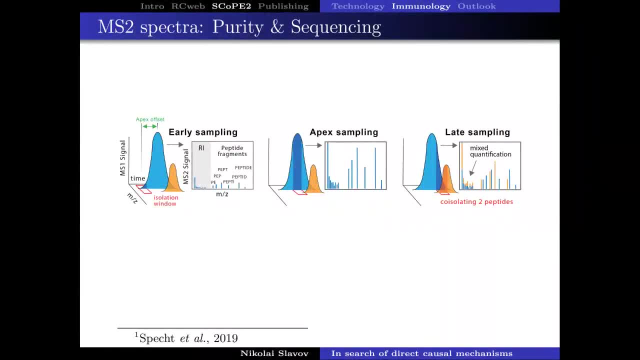 the blue corresponds to one peptide, the orange corresponds to another peptide and then, during a particular period of time, the instrument is going to select that peptide for further analysis, for fragmentation and determining its structure by tandem mass spectrometry and, as you can see from the graph, from the panel on the left, 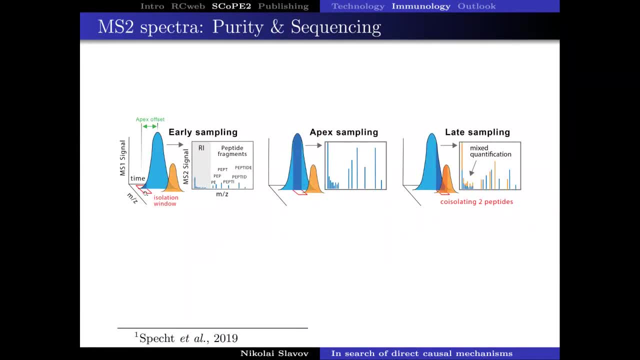 if the selection happens very early, then you are going to sample very small amount of that peptide and therefore we might not have enough material to determine the composition of that peptide, what the sequence is, and to quantify it. if it's a sample put in the middle, while 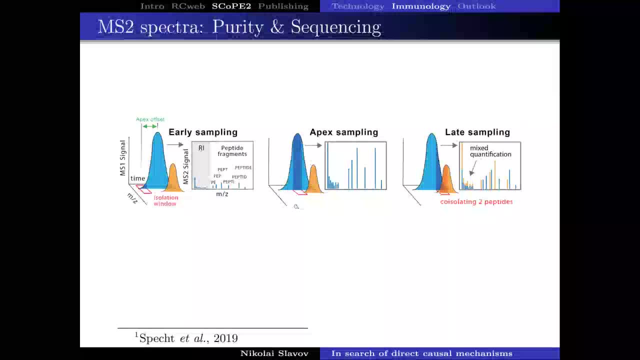 avoiding sampling any other peptides. that can result in optimal sampling that maximizes the copy numbers of that particular peptide that are analyzed and the purity of the ms2 spectrum. and then another problem that might happen is if at the time when you're sampling the blue peptide, the 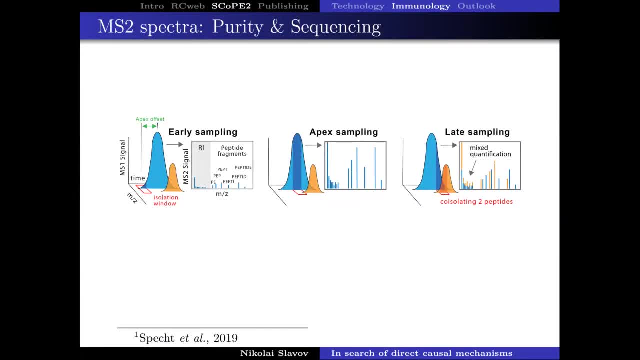 orange one is co-eluting and falls within the sampling window. we might co-isolate both the blue and the orange peptide, and that results in hybrid spectra that undermine the quantification and also undermine the ability to identify the sequence of the peptide. so these things are. 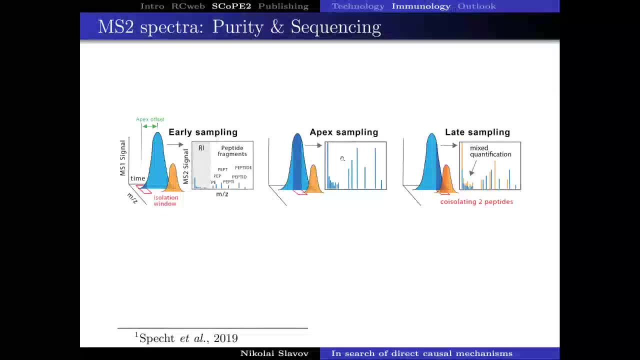 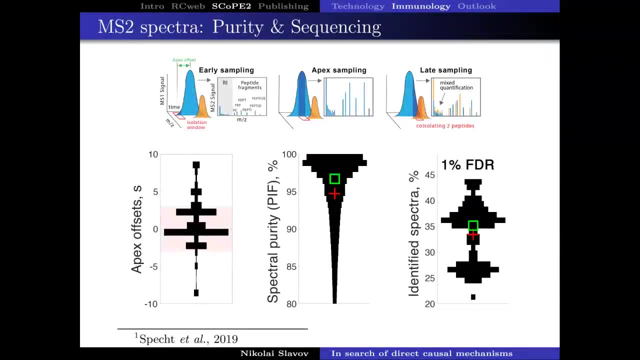 desirable to minimize, and they were an important part of what we had to optimize in the experiments that i described. so here i'm showing some graphics summarizing the extent to which we were able to optimize it. the first one, with the apex offsets, shows the time away from the apex of the elution. 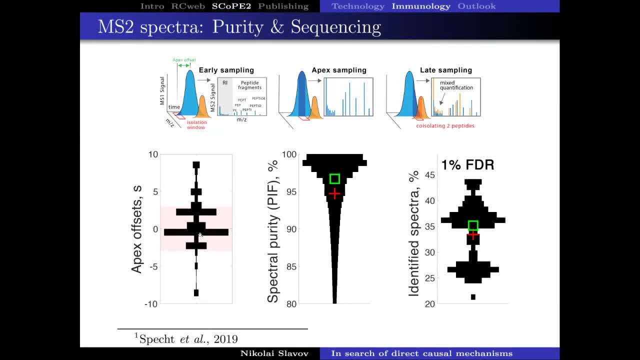 peak that the peptide is being sampled. the majority of the peptides here shaded- the shaded part of the distribution- elute within three seconds or less, and that corresponds to something very close to the apex. these peaks are about 20 seconds wide at the base. so that's and because the sampling is so close to. 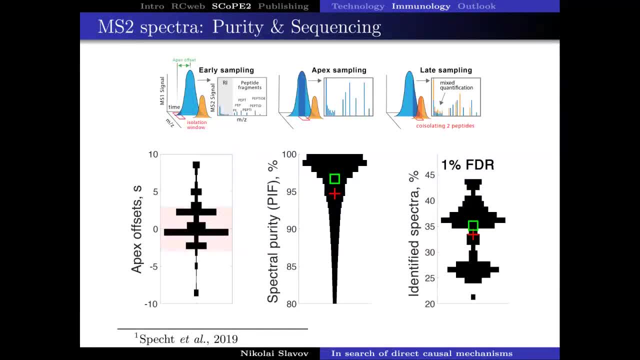 the apex, the spectra are about 95 percent or more pure, which helps with the identification. in this case we are able to assign confident peptide sequences to about 35 percent of the analyzed peptides by by ms2 analysis and of course, a high spectral purity helps improve the quality of quantification. 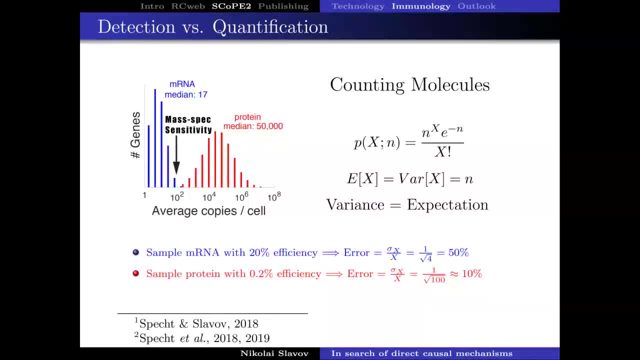 now, one thing to worry about when doing single cell measurements or measurements of tiny amounts of material, is that if you detect very few molecules you may not be able to and you perfectly detect them. you count them, you may not be able to detect. uh, use this detection to quantify their abundance in your sample. 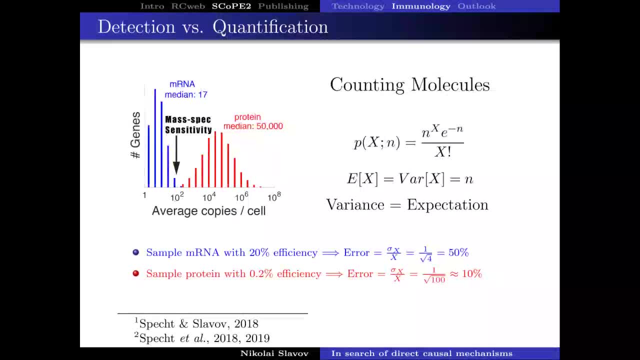 and to illustrate that, i'll use the analogy of sampling red and blue balls from a bucket. if i have a bucket full of friend blue balls and i ask you to sample three bowls, you can pick them and find two blue balls and one red. now from if? even though you can ascertain where the 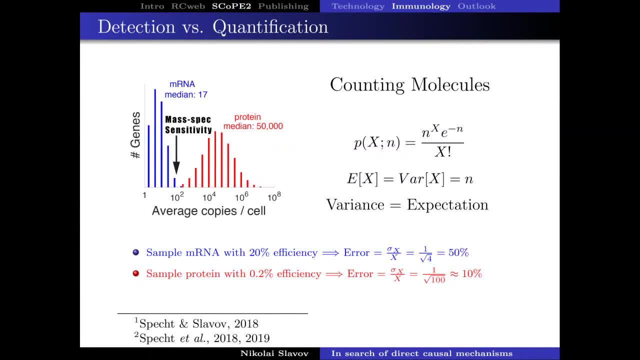 to ascertain with absolute certainty what are the colors of these bowls. you cannot use that information to accurately infer what was the ratio between blue and red bowls, because if that ratio is 84 to 5, you cannot approximate 84 to 5 with any ratio of numbers between 1 and 3.. 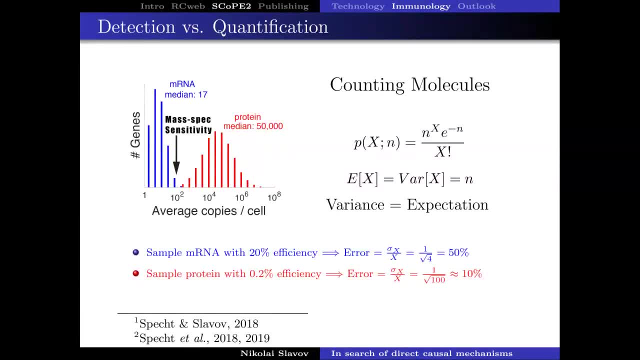 And more fundamentally, we can describe this problem of sampling very, very few observations from a distribution with a pulse on distribution. In fact it maps perfectly to the pulse on distribution And that represents a major hurdle for most types of single cell analysis, because we rarely sample all of the molecules. If we sample only a subset, that subset should be large enough to result in representative estimate of the abundances. 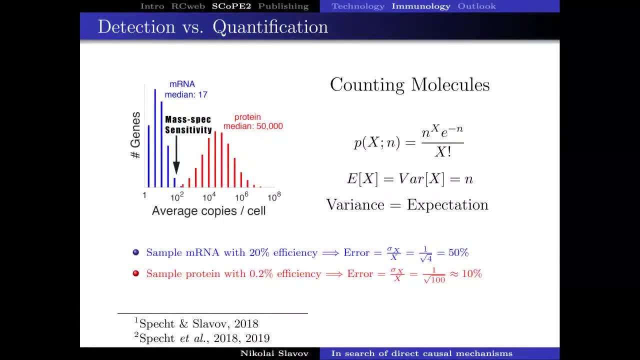 Currently for single cell RNA sequencing. that is one of the major bottlenecks for their accuracy. Even the most efficient methods sample about 20% efficiency messenger RNAs And because messenger RNAs tend to be lowly abundant- on average 17 copies per cell or fewer- that low sampling efficiency results in fairly large counting errors. 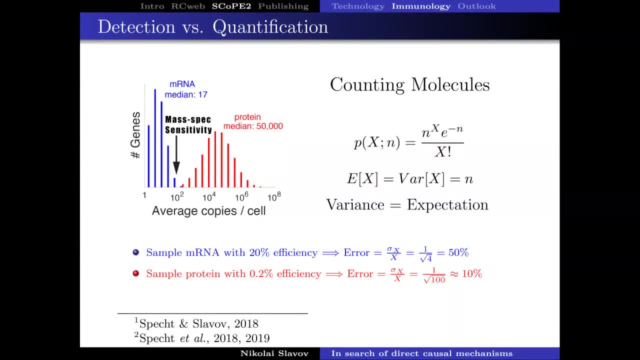 And this is even in the case when the rest of sample proteins. The thing that is quite helpful with analyzing proteins is that proteins are much more abundant And even if we have a hundred fold lower efficiency in sampling them, we might still sample more copies per protein, which might result in having less counting noise in estimating their abundance. 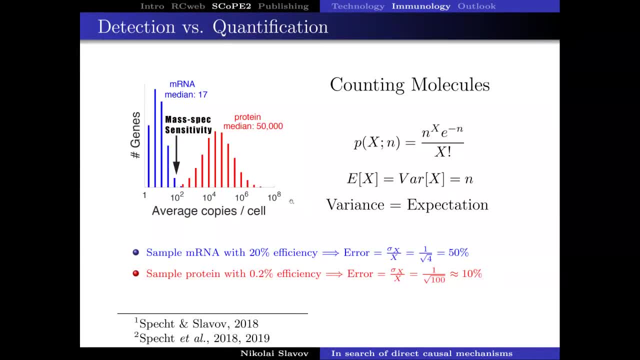 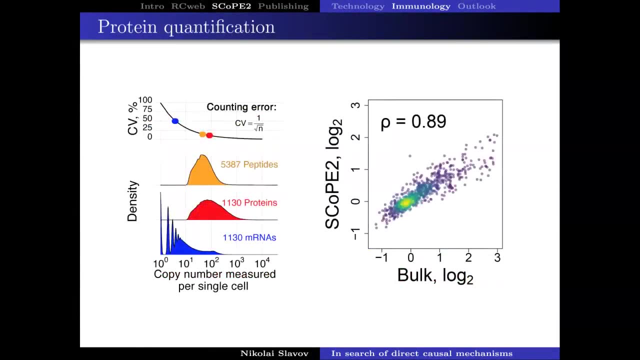 So that was the theory. That's something that we proposed Long before we could actually estimate what the sampling efficiency is, And the gratifying part is that when we get around to estimate the copy numbers that are being sampled- per protein, per single cell- 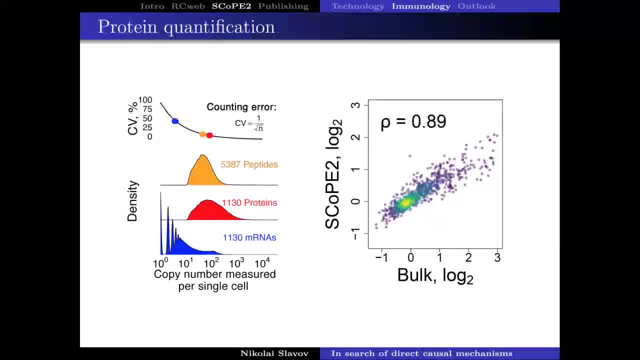 By the described methods we found that that corresponds to about 100 copies per single cell, which corresponds to relatively small counting error- Not negligible, But relatively small- and compares very favorably to the copy number is sampled by 10X genomics with state-of-the-art single-cell RNA sequencing method that, even when implemented optimally, has about 50% counting error in our case. 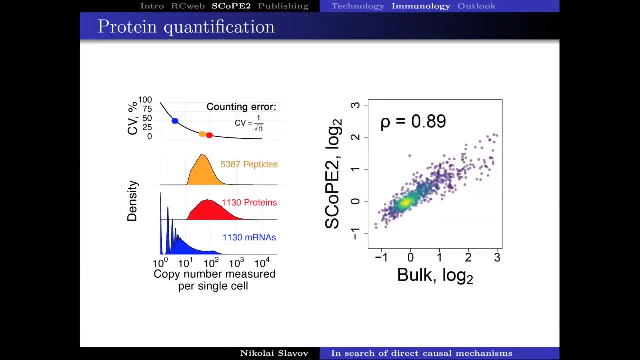 So the ability to sample multiple copies per protein results in about 50% counting error in our case. So the ability to sample multiple copies per protein results in about 50% counting error in our case. So the ability to sample multiple copies per protein results in about 50% counting error in our case. 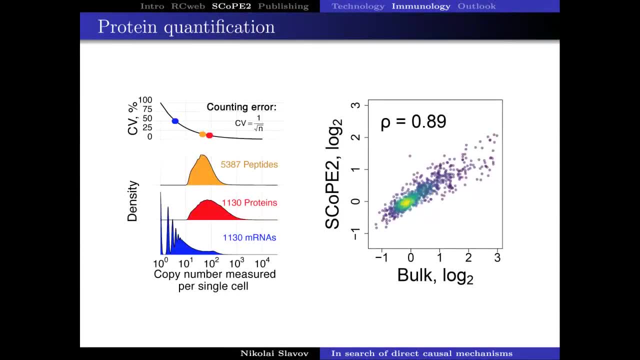 And then we had this relatively good quantification shown here to the right. The way we are benchmarking quantification here is by estimating the relative protein levels. The way we are benchmarking quantification here is by estimating the relative protein levels For proteins between monocytes and macrophages. Estimated by conventional, well validated bulk methods And then doing the same relative protein estimates by in silico averaging out protein abundance, Which means we now do some more sampling with the specific protein that she was trying to get away with, which is higher protein. Norther than just pick some Enlightness, which is the same model. it's actually musclesright. So without the Dropbox column, both of these methods were poor, But for proteins that are saying low fr, Integration of protein, it's also very important. 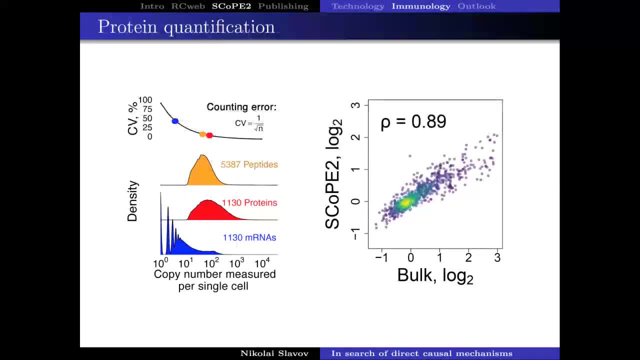 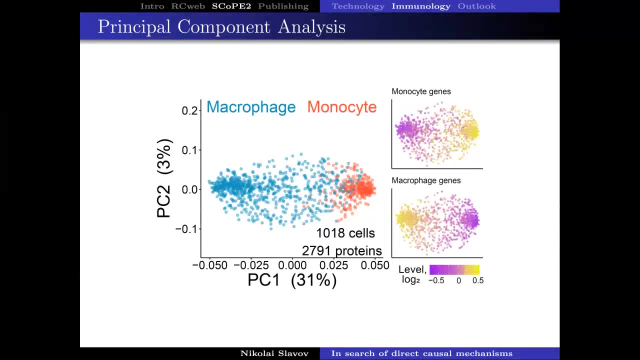 averaging out protein abundances within monocytes, averaging out the same abundances within macrophages and then taking the ratio, And these data allowed us to quantify about 3,000 proteins- a little bit fewer than that- across over a thousand cells. and if we just project these data into the axis of their 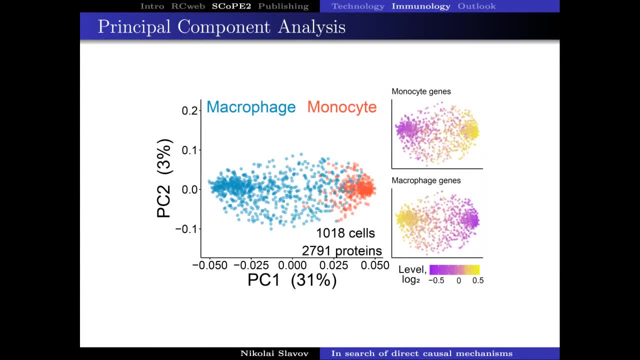 principal components. we see two clusters because during the sorting process we knew whether a single cell was monocyte or macrophage. we can color code each cell by its identity and we see that the clusters correspond to the different cell types, as one would have hoped. Similarly, we can color code now each single. 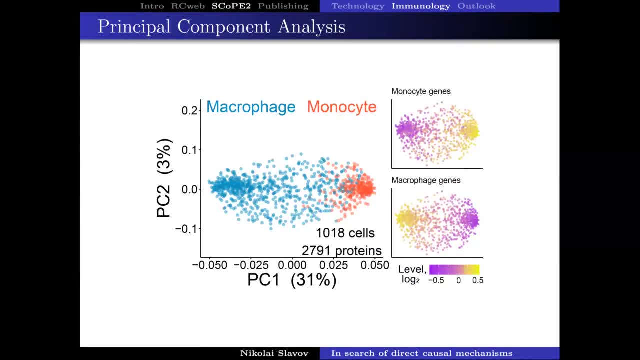 cell based on the abundance of proteins that are either monocyte or macrophage markers, and we see that this coloring scheme shown to the right again indicates that the two clusters correspond to the two different cell types. Now, one reaction that the reviewers had on seeing this was that 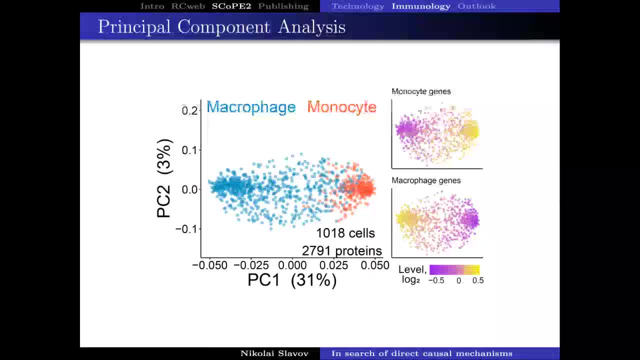 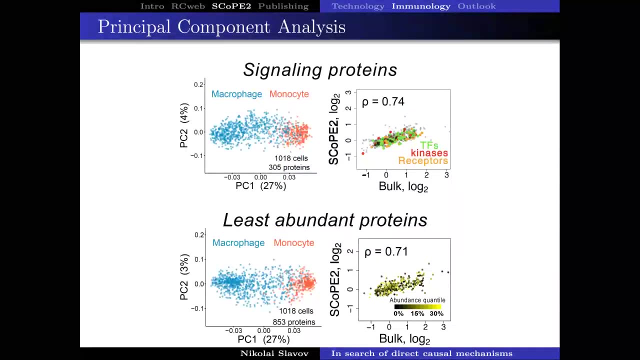 perhaps the separation is being driven mostly by some highly abundant proteins, while the proteins that correspond to regulatory functions are not well quantified, and we could very easily evaluate this concern quite directly by limiting our analysis just to proteins such as macrophages. 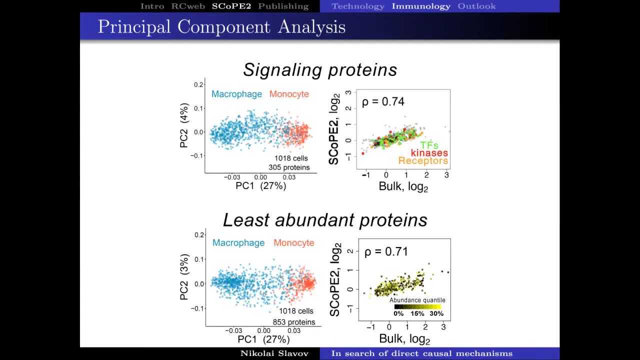 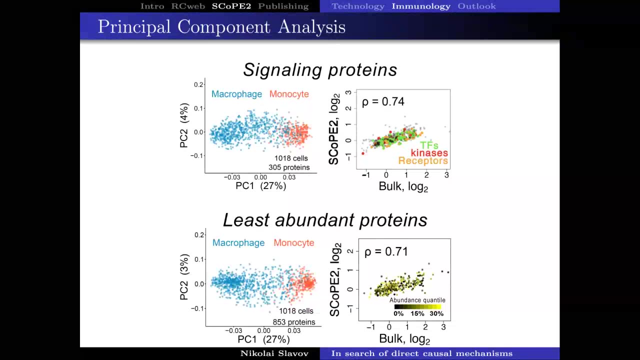 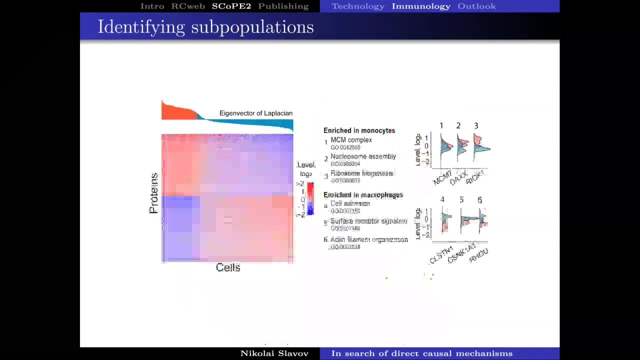 transcription factors, kinase and receptors and see whether we can still identify the clusters and what is the accuracy of their quantification. specifically, and as shown here, both such regulatory proteins as well as the least abundant proteins in our data set tend to be quantified reasonably well and allow separating the different cell types. the next thing that we did was to use 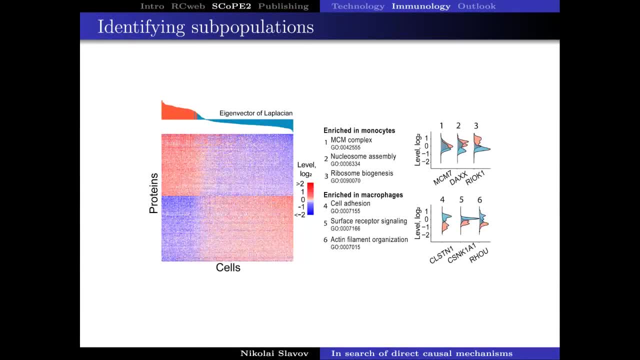 spectral clustering, which is a method that allows to identify structure within the data sub-clustering, without assuming that they're distinct clusters. essentially, the way this works is that we we can use the similarity- pairwise similarity- between different single cells to build a graph, and then the eigenvector of the lapletion of that graph is being used to sort out single. 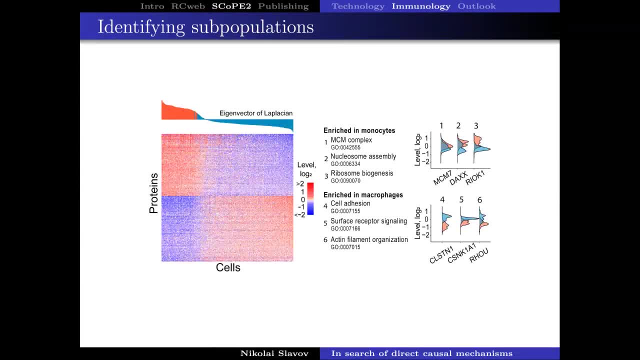 cells basically permute their orders. here each column corresponds to a single cell and when we do this analysis, we see that the distribution of the elements of the eigenvector is mostly bimodal and the clusters fall into and the the continuum, while not being entirely discrete, falls within. 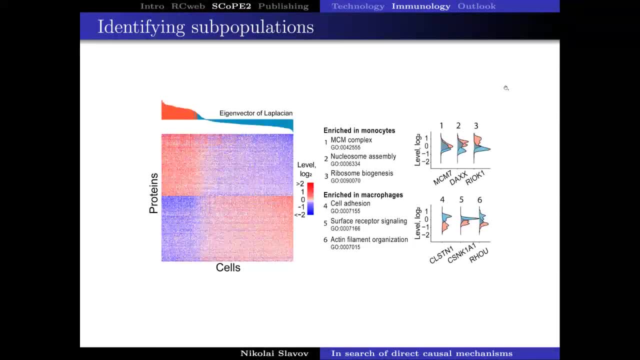 two in within two modes, with the proteins being enriched in each cell type. in this case here, within the monocytes, we can see what proteins are more abundant and these proteins tend to function within ribosome biogenesis and cell division, which makes sense because monocytes are actively. 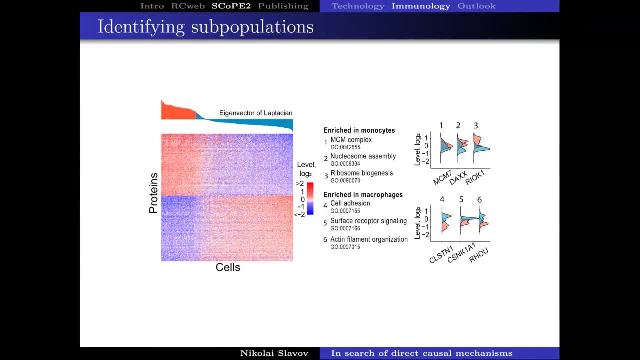 dividing, proliferating, while macrophages are post-metodic, mostly they they don't divide as actively. while in the case of macrophage cells, we see enrichment for proteins with immune functions and particularly proteins participating in cell adhesion, which makes sense because macrophage is 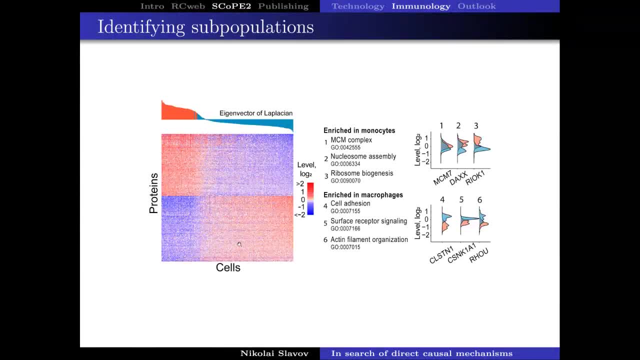 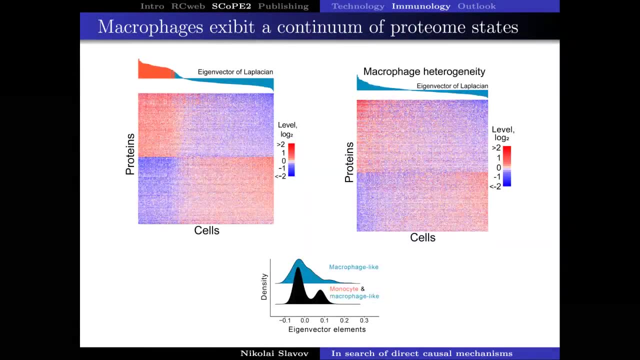 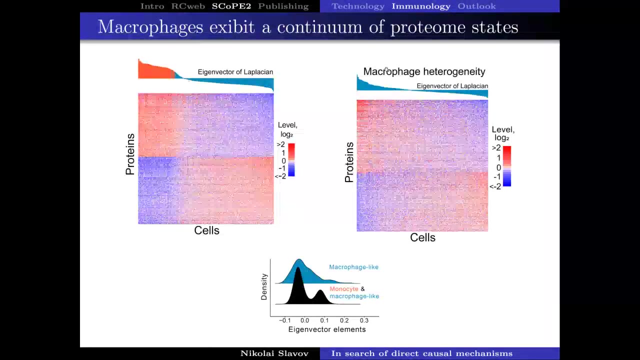 an adhesion cell, so they adhere. and, interestingly, when we apply this exact same analysis just to the macrophages, we see that there is a continuum of heterogeneity between the single cells, with much, much less bimodal distribution of the elements of the eigenvector, of the, of the 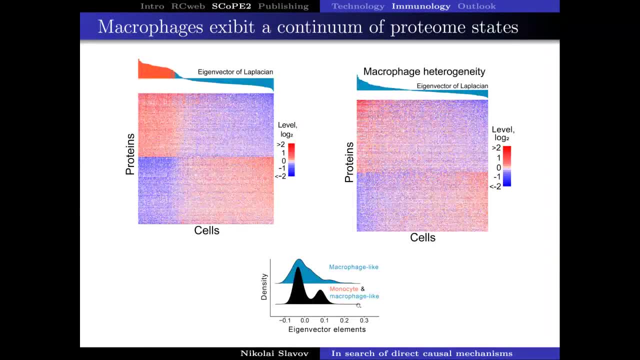 lapletion matrix. so you can see this more quantitatively here, with the distributions plotted at the bottom, with the eigenvector corresponding to the whole population being clearly bimodal, one mode corresponding to monocytes together to macrophages, while the macrophage-like cells 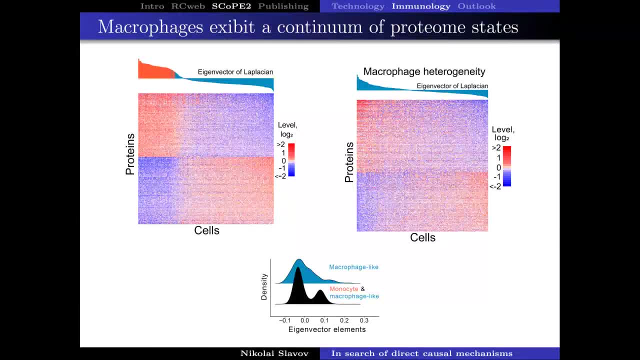 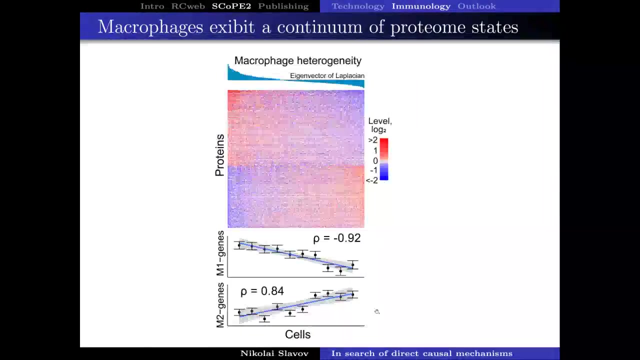 show, have a unimodal distribution. now what? what's this heterogeneity that we still observe within the macrophages? of course, one possibility would be that it's just noise. even though it doesn't look as a noisy pattern, it looks more like, more like a general trend within the different single cells. so one way to begin to ask and 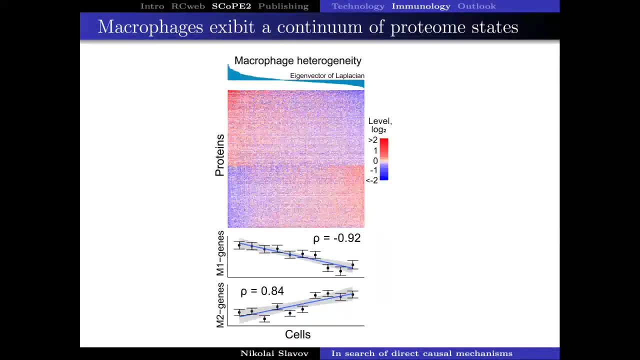 learn about what it might correspond to is by looking at the functions of the proteins enriched in each end of the spectrum and throughout the continuum. so to do that, we looked at genes that had been previously as annotated to either m1 or m2. polarization of macrophages. 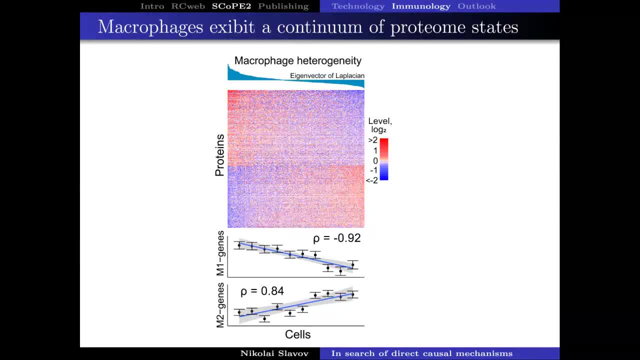 and we found that the abundance of the proteins corresponding to these genes is very, very strongly correlated to the gradient of polarization, with m1 genes being strongly enriched in the left continuum, in the left end of the spectrum, and their abundance gradually decreasing and the opposite trend being 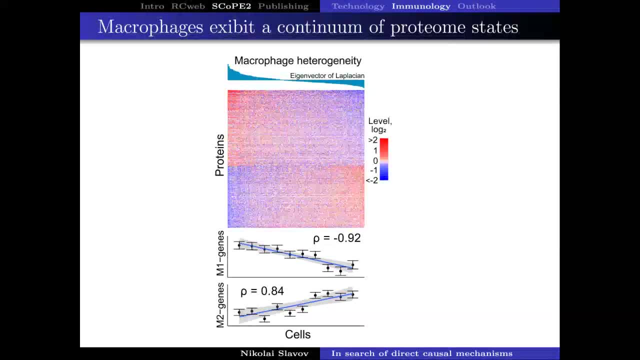 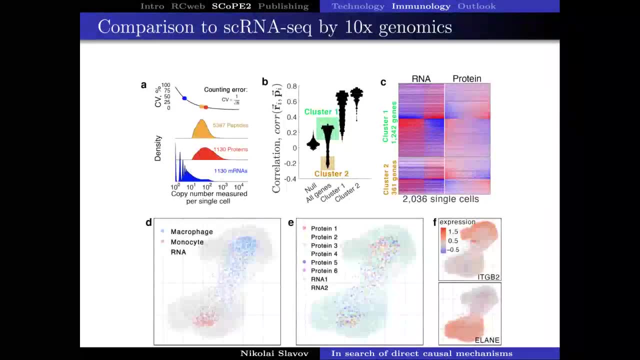 observed for the m2 or the anti-inflammatory macrophages. and then, of course, we wanted to compare the protein measurements to the rna measurements and evaluate the degree to which they're similar or different and what we can learn from one and the other. so, to this end, we performed correlation vector analysis to compare. 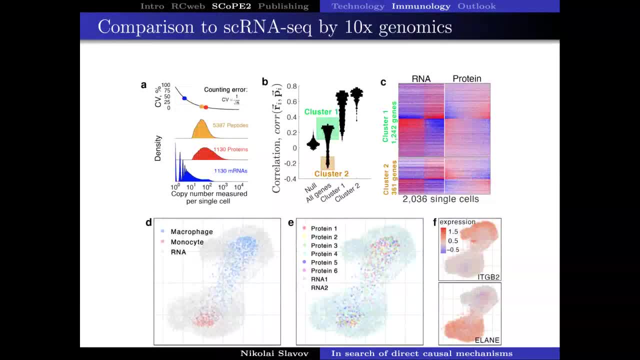 to identify genes that have similar responses at both the protein and the rna level and genes that differ in their response and protein and the rna level. based on this analysis, we see that the majority of genes- over a thousand genes- have qualitatively is not, if not quantitatively, at 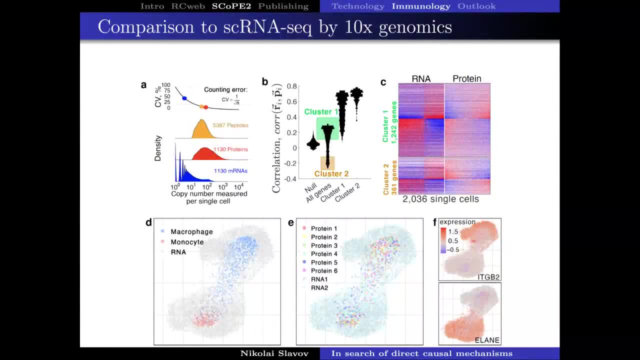 least qualitatively similar responses between the monocytes and the macrophages, as shown here in panel c, while a smaller group of genes, a bit over 300 genes, show the opposite response at the rna and the protein level, with many genes not being not changing the response to the macrophages and the 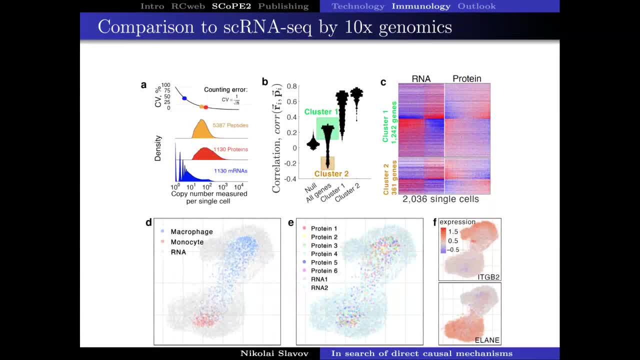 not changing significantly between the monocytes and the macrophages. Now, considering the different copy numbers being counted for the proteins and for the RNAs, we were particularly interested to see what is the overall variability in the data. So to do that, we projected the data into a joint low-dimensional 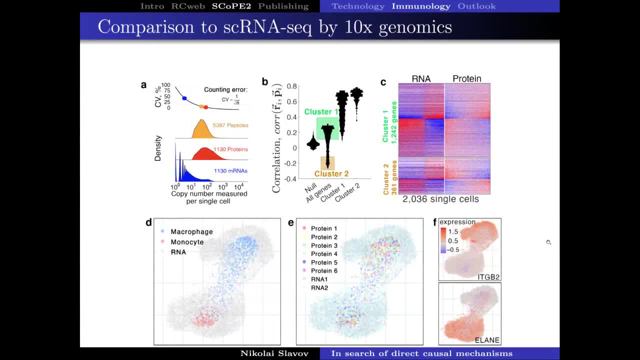 manifold using CONUS, an algorithm recently developed for projecting different single-cell RNA datasets into the same low-dimensional manifold, but could be easily generalized to work with protein data as well. And as you can see here in panel D, the joint projection is still composed of two. 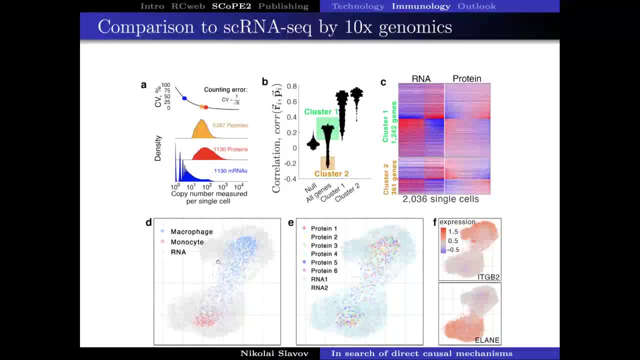 clusters, but the protein data form the cores of these clusters, while the RNA data is more diffused around them, seeming to have more variability. Quite importantly, we could see that this projection has been able to eliminate batch effects between the different clusters for purposes of 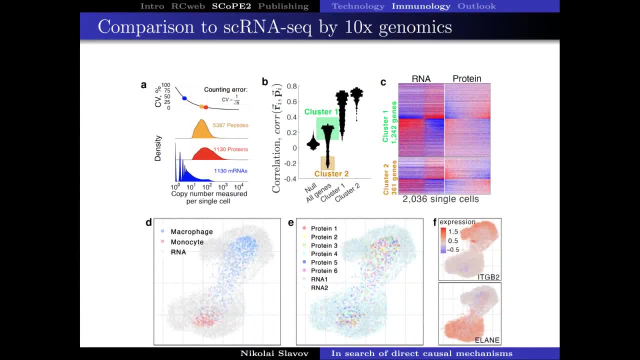 benchmarking and validation. We had both multiple biological and technical replicates within the data and we can see that these biological and technical replicates were uniformly dispersed within the clusters, showing that batch effects and biases, whatever they were, could be easily, could be easily analyzed. So we can see that the batch effects and biases, whatever they were, could be easily, could be easily. 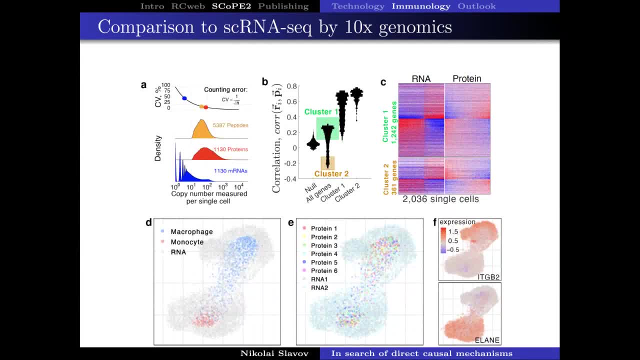 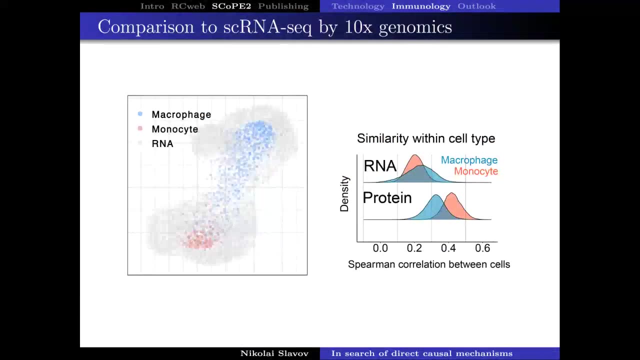 corrected for And again using marker genes, we can easily identify the two different cell types in our data. Now I want to come back to this observation of having observed more variability in the RNA data compared to the protein data, because it's potentially important. We don't fully understand it, we don't know. 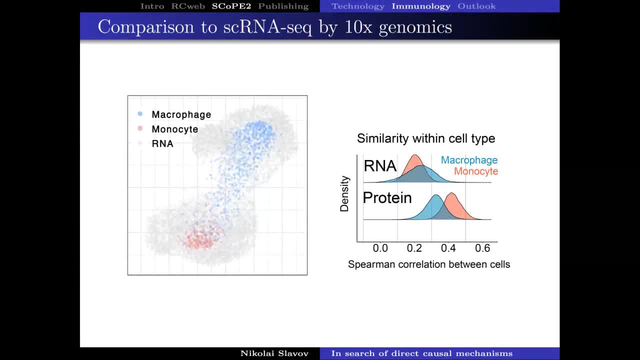 what's contributing to it? entirely, It could be. it could be driven by having more technical noise because of counting small copy number of RNA molecules in the RNA data. It could be related to having more biological variability among messenger RNAs because of stochastic transcription. It is known. 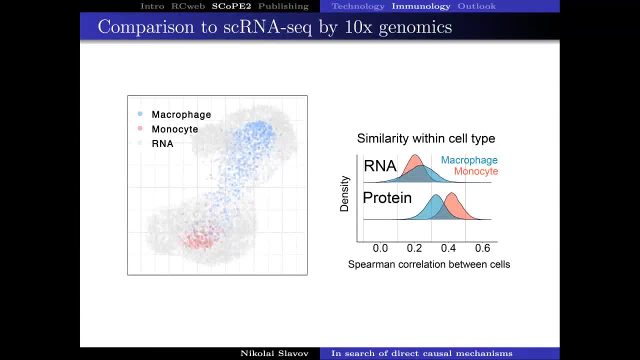 that many messenger RNAs get transcribed in bursts and proteins, being much longer lived, tend to average out that variability and there might be less biological variability at the level of the proteins, But we couldn't infer just from the low dimensional joint projection that there is less. 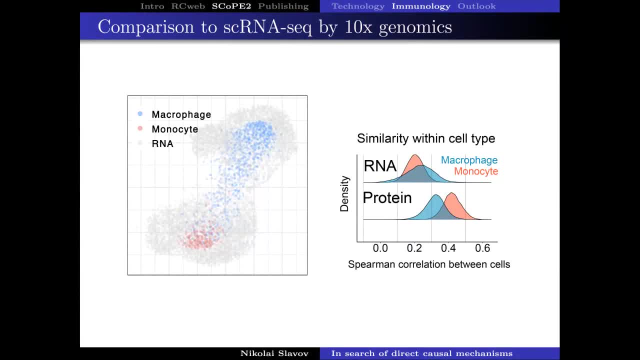 variability, because that captures only a fraction of the variance in the total data set and can be misleading. And that's an important thing for you to learn and transfer to your work: that low dimensional projections, visualizations, manifolds, can be very useful for depicting data and for 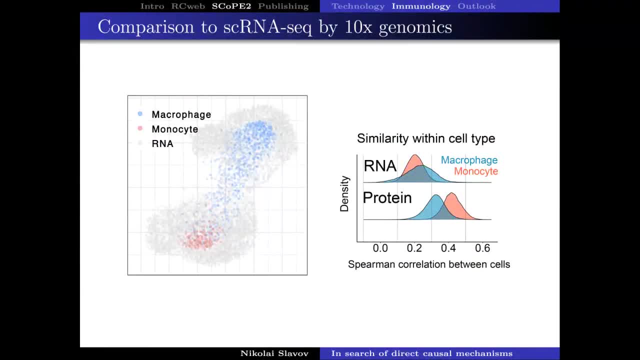 visualization, But they can be also highly misleading. so it's important to conduct different types of analysis that can independently confirm or invalidate the observation without making some of the approximations of the low dimensional projections. So in this case we simply used pairwise similarity between the. 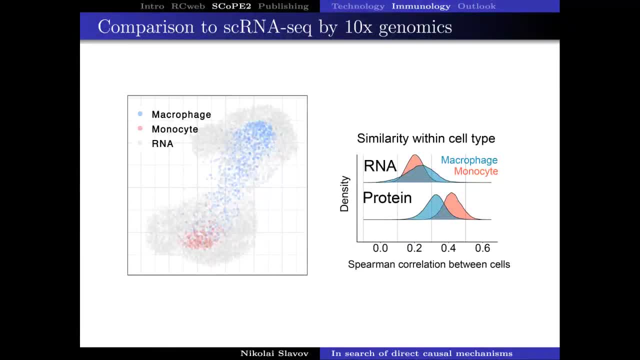 proteomes of single cells and the transcriptomes of single cells to measure their similarity or differences. So we computed all pairwise correlations between all single cells at either RNA or protein level and plot these distributions for both the monocytes and the macrophages, And what you can see here. 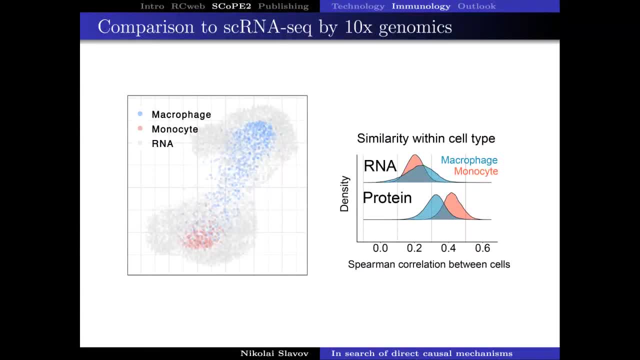 is that the correlations among the proteins are indeed higher, which is consistent in this case with the low dimensional projection, that we see less variability between the proteins of the proteomes of single cells compared to the transcriptomes. You can also see the difference between monocytes and 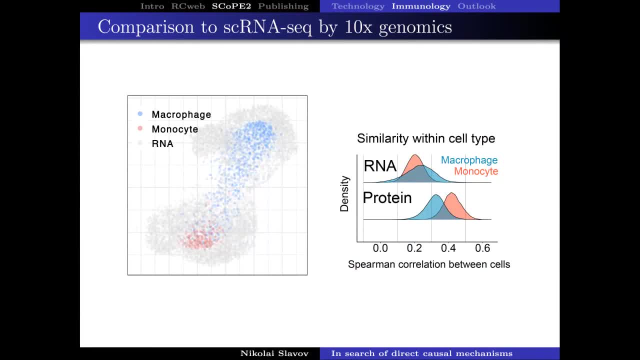 macrophages, The monocytes, have high correlation, which makes sense considering that monocytes are much more homogeneous- They're more or less clonal cell line- while the macrophages, as they differentiated, became more heterogeneous, and that's what our previous analysis identified as well. It's 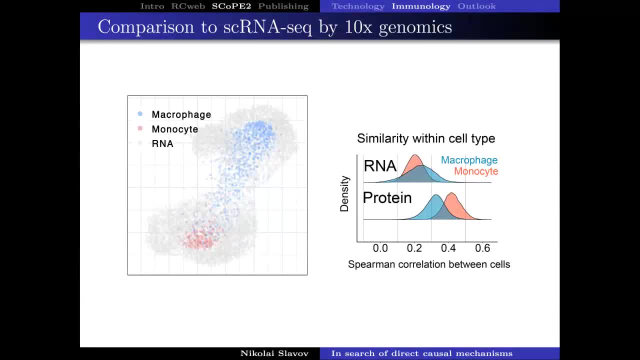 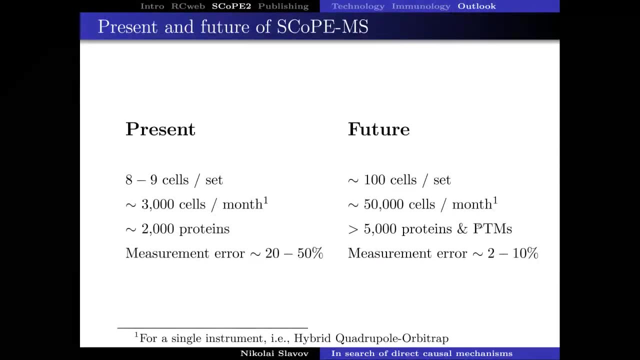 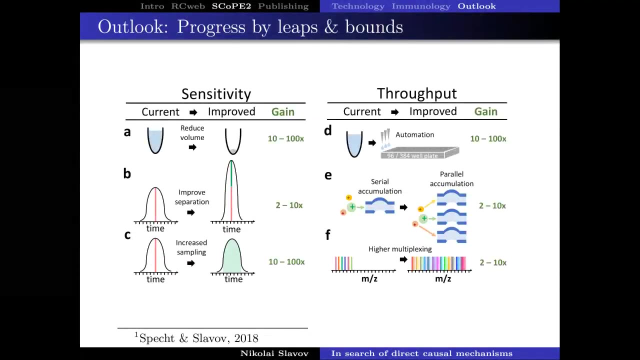 just nice to see that being reflected in this type of analysis as well. So what I have shown you so far is just a small vignette, a particular application and a short description of the methods that we have started developing, but I don't want to give you the impression that this is a mature field and we have 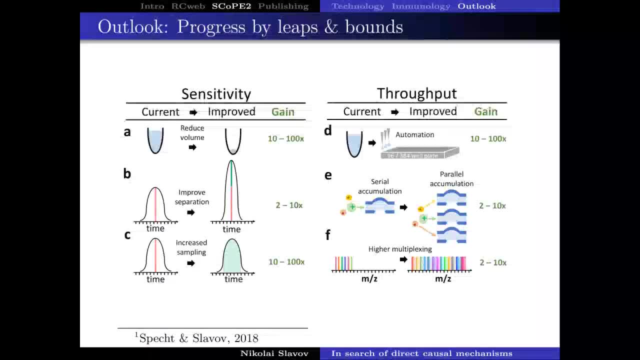 done everything that can be done. In fact, there is a lot of opportunity for a further advancement of these methods, both on the side of sample preparation, and in fact Andrew LeDuc is working on one of your classmates and colleague is working in my group trying to improve sample. 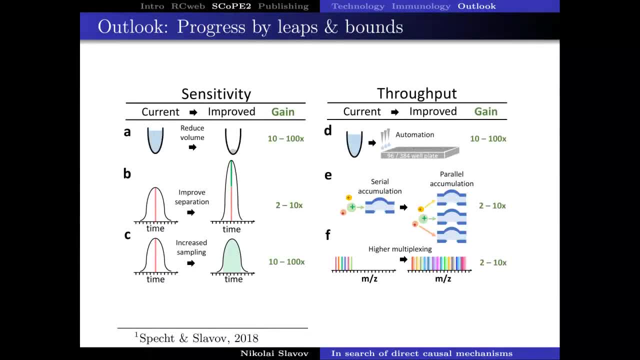 preparation, increasing its throughput, increasing the number of isobaric mass tags that we have to increase, multiplexing, improving chromatography, improving instrumentation. There are very many aspects that can be improved in this type of analysis. These are just early days. 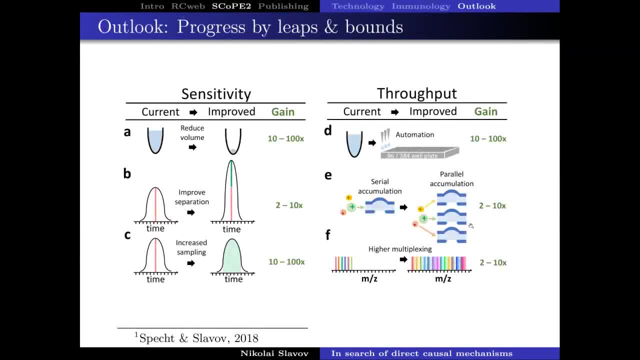 Now I want to pause here for some questions because, if we have time, I would like to spend the remaining 10-15 minutes discussing something very different and again going back to one of the themes in the class of learning: how the scientific enterprise works and what are. 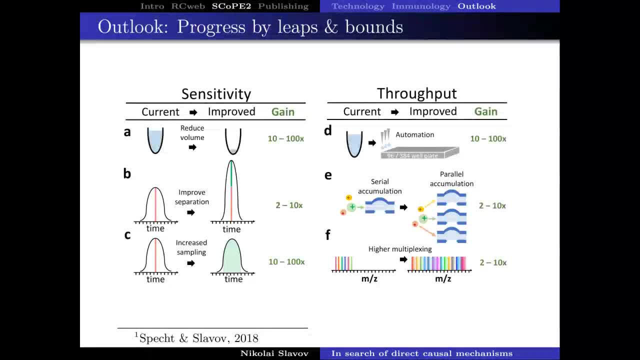 some of the weaknesses and strengths of the current publishing environment. So do you have questions for this part of my presentation? Hi, Oh, sorry, You go first. Okay, So I was thinking, when you were showing the original mass spec data, that you could. 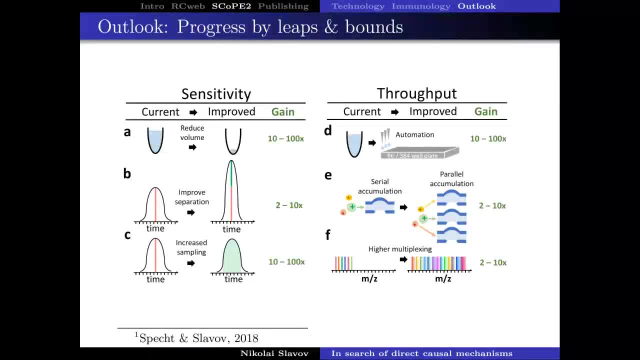 improve separation and sampling time, but I guess are there any kind of co-sensitivities that you need to be aware of as you're trying to improve one of these factors like separation or sampling, reduced volume et cetera. I'm not entirely sure what you mean by co-sensitivity, but there's no downside. 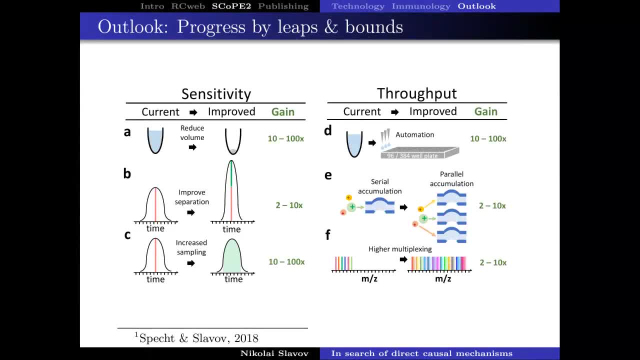 If you improve separation, for example, or ionization, there's no downside associated with that. but it's quite hard to improve it because the factors that tend to improve separation also make the chromatography less reliable and harder. so it's fairly hard to. 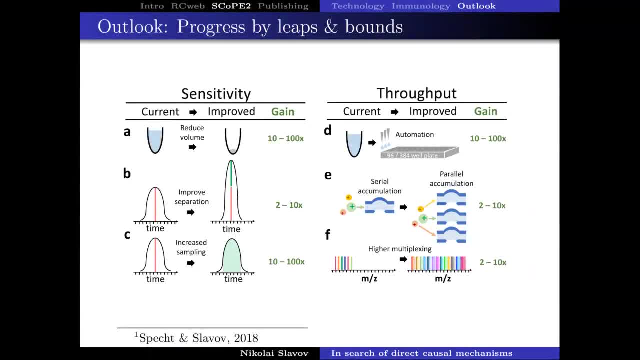 improve that. Similarly, there are no substantial downsides If we increase one of the factors multiplexing by a factor of 10, which is going to decrease cost by a factor of 10, it's going to be a huge benefit, but it's not so easy to synthesize 10 times more isobaric. 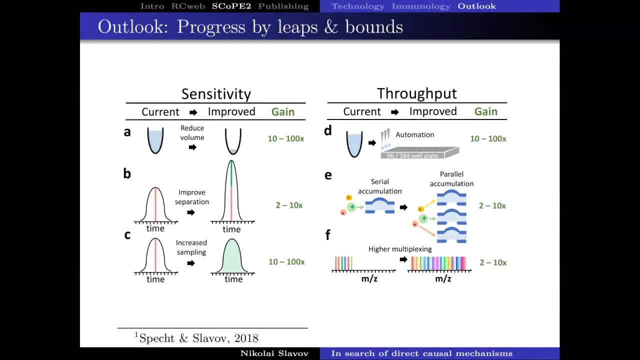 mass stacks. So it is not so much that there are downsides that you're facing these tradeoffs. It is more that some of these technical improvements are not so easy to accomplish, but nonetheless they're quite feasible and doable, which is what makes it exciting to try to push the 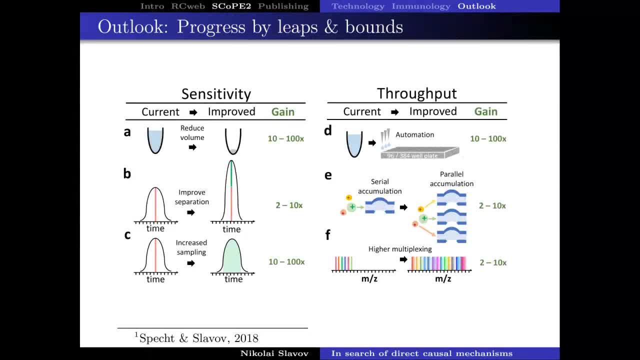 technology further. Hi Professor, It depends on the flow cytometry technique I'm thinking. if that's possible, based on the different proteins, like the surface protein extraction on the manual set or the macrophage, we can use the flow cytometry cell sorting to separate them. 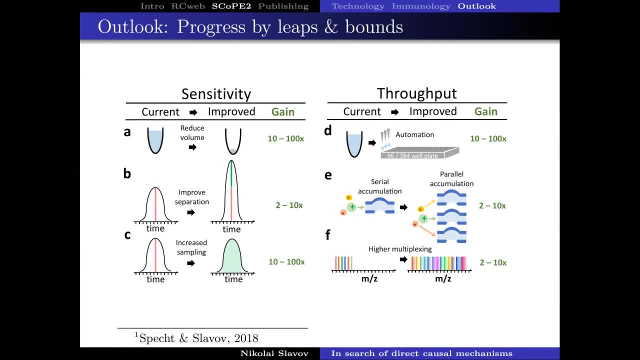 Certainly you can use flow cytometry. It's one of the best and only slightly moreогоful processes in a cell to establish longest standing methods for a single cell analysis. The issue with flow cytometry is that it mostly has to rely on antibodies to have molecular specificity, and there are 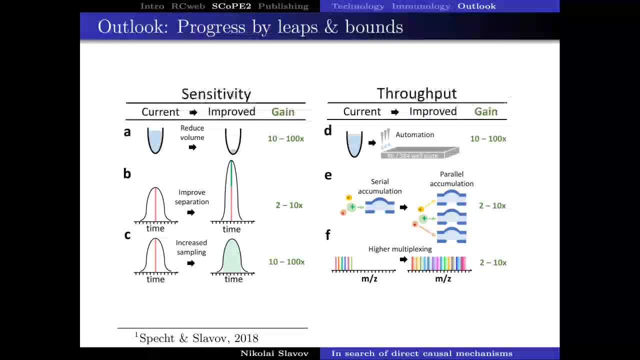 limited number of antibodies that can be labeled optically without having intolerable overlap between the emission spectra of the fluorophores. And then there is the whole issue with the low specificity of antibodies, And also the issue that we discussed of perturbing the cells as we take them for analysis, when 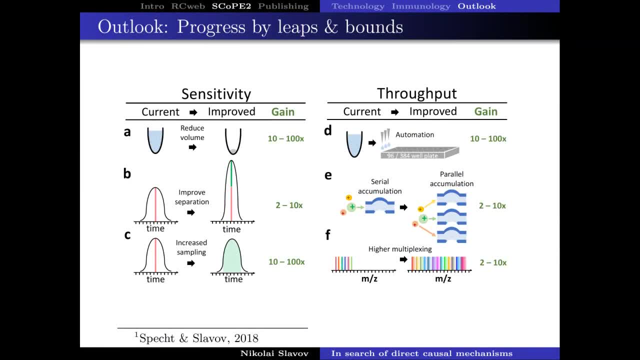 antibodies bind receptors, they can actually stimulate those receptors, which is oftentimes used for biological experiments. Now, if we're using the antibodies just as a way to detect these proteins, we might also inadvertently be causing stimulation of these cells, which results in downstream changes. 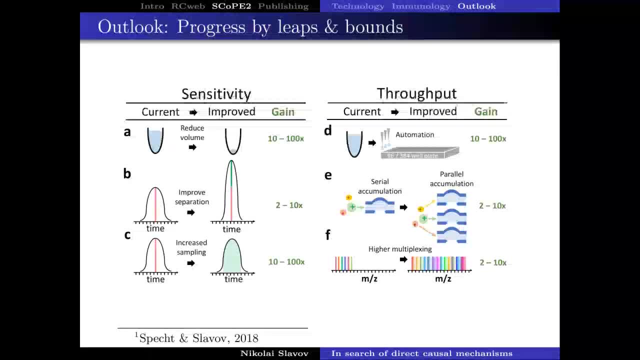 in their proteomes. But there are certainly many ways to combine these technologies that I'm describing with flow cytometry and use it as another dimension that is useful. It is just that flow cytometry itself cannot really at present give us quantification. 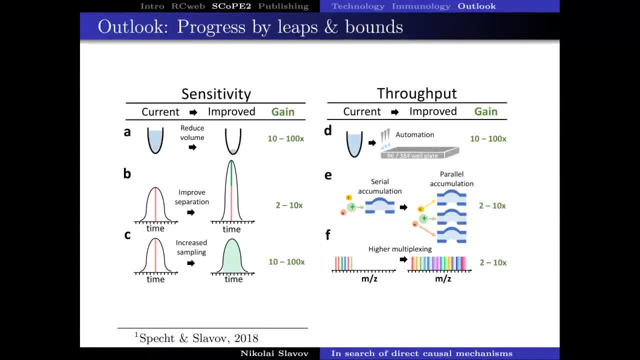 of a large number of proteins with good specificity. Okay, Professor Schlebel. Yeah, This is Kanika. I have a question. Can you please repeat the question? Yeah, I have a question regarding so with your research right now, you showed that there. 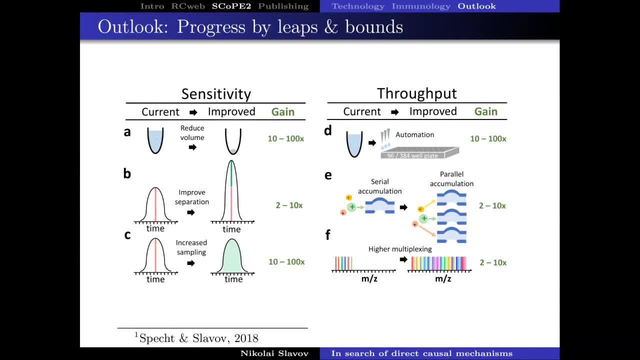 was heterogeneity in macrophages themselves. but would you be able to also show that various cytokines can really induce the change of its phenotype from M1 to M2 or vice versa, Like, for instance, subjecting them with IL-10 to change M1 phenotype to M2 phenotype and 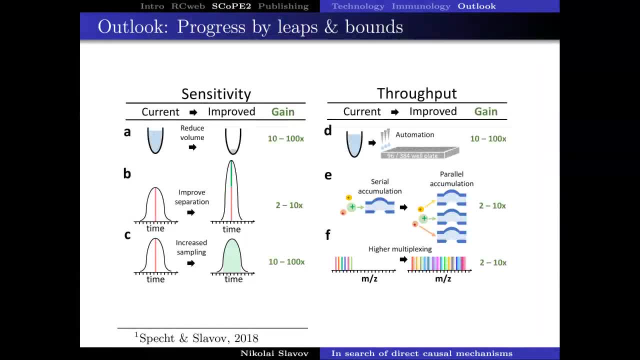 then screen a variety of them to just understand which one really works in modulating. You know, modulating that phenotypic change. So this is very clear that we can influence polarization of the macrophages by using cytokines. It's interferon gamma, for example, classically is known to induce M1 polarization and IL-4. 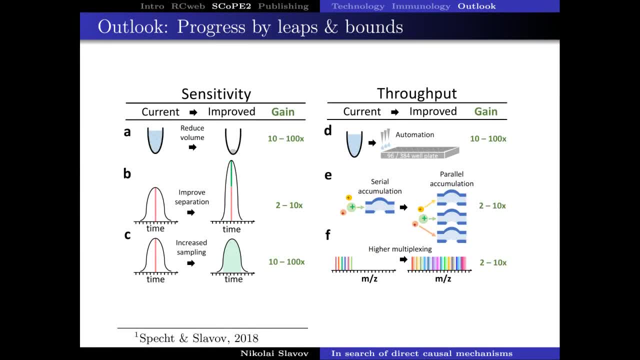 induces M2 polarization, So one can certainly alter that polarization. The question is also: when you alter that, it's actually interesting to what extent you still have heterogeneity When this is being done, and this has been done hundreds and hundreds of times. people 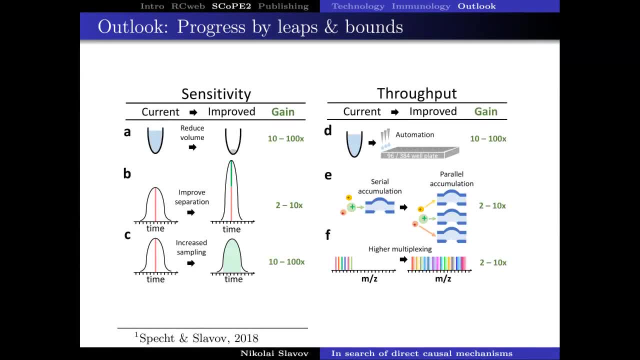 normally would do a bulk measurement within the cells and establish that there are certain markers that are increased for each cytokine and associate these with a particular polarization. I think the whole paradigm of M1, M2 polarization is really grossly oversimplified and it's 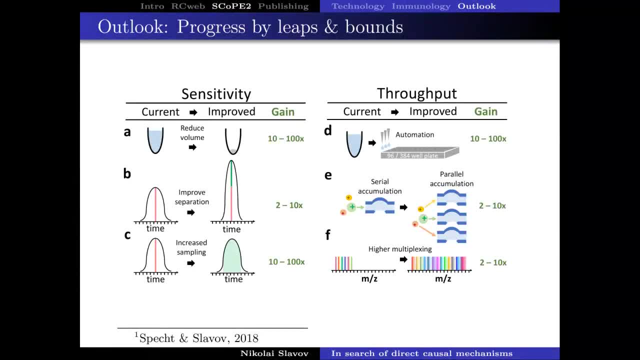 not just a single axis of polarization. There is a lot more heterogeneity being present, Mm-hmm, And it is very clear that that heterogeneity will be strongly influenced if we add cytokines. So in this case, the model system is just used specifically to look whether there is 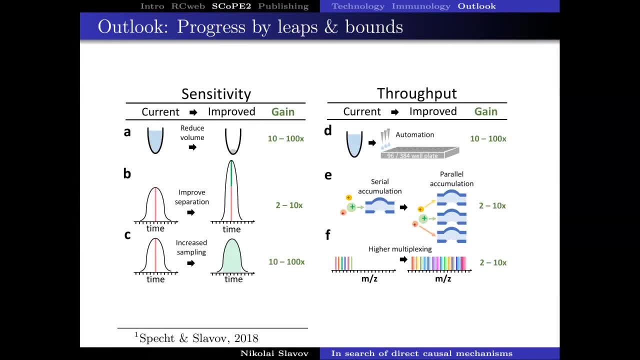 polarization if we don't explicitly add cytokines. And then if we were to add a cytokine, then we can still repeat the measurements and likely we would still find heterogeneity. but now that will be different and one has to think what is a good question to ask there and how do I design the corresponding experiment? 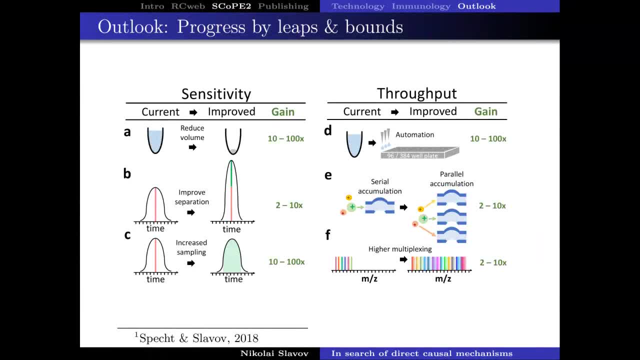 And especially like in terms of you know. I mean there is a theory which says that when there is inflammation, like for instance in the gut, for IBD generally, macrophages move, like there have been studies wherein if there is a wound in the body peritoneal, 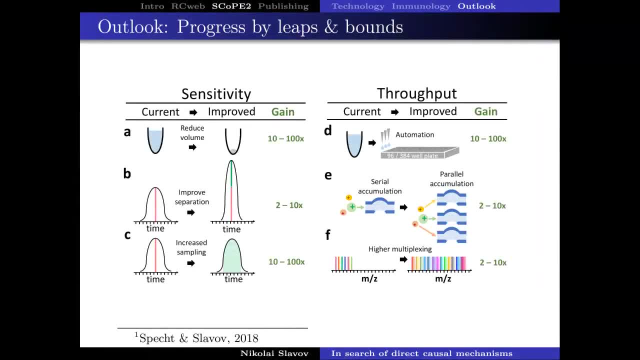 macrophages really move to the wound, And so I was really wondering like, for instance, in this case right, if the monocytes they sort of differentiate into these, you know, anti-inflammatory macrophages in the gut, for instance, right. 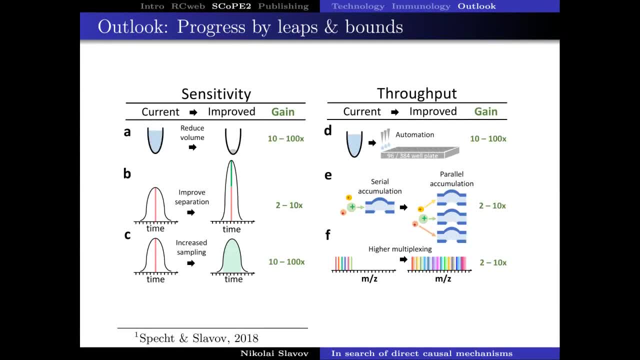 And then perhaps those kind of models could be, you know, formulated and studied Absolutely, and that would be very good to do with primary cells taken directly from the gut of either experimental animals or patients. if that's possible, Yeah, there is certainly the scope for doing that kind of analysis. 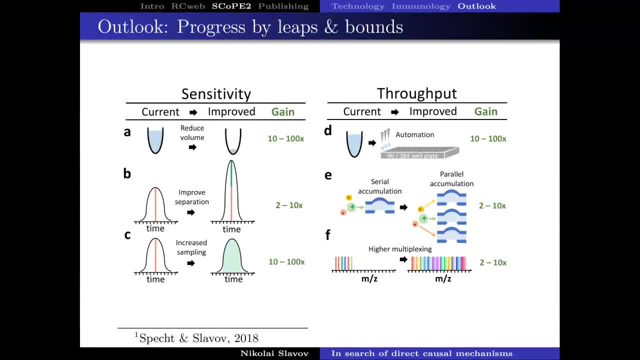 Thank you. I have a couple of questions that are sort of related. So you were discussing How, with the scope method, you have a higher copy number per cell than as compared to RNA-seq. Is it that you measure more per cell or that more exists per cell? 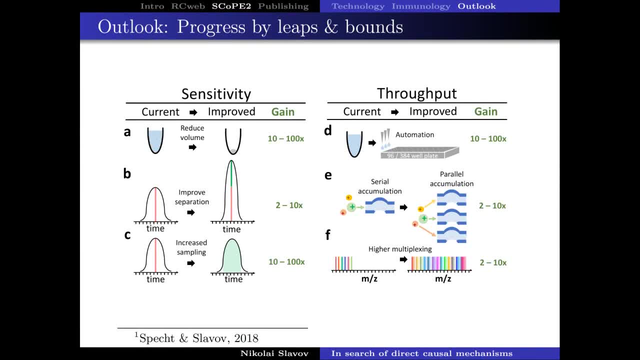 And is it relative to single-cell RNA-seq? you're comparing, That's right. We are comparing relative to the single-cell RNA sequencing for the same gene. So we intersected the genes. We didn't want to compare a lowly abundant genes in one set to highly abundant genes. 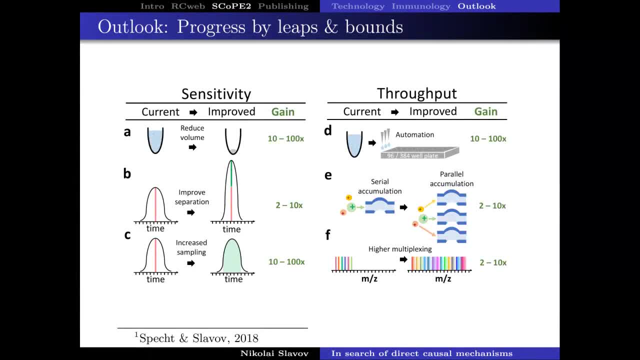 in the other. So there are a lot. Our capture efficiency with scope 2 is lower than for 10X genomics. 10X genomics or single-cell RNA sequencing methods. they have capture efficiency between one. Well, it can be less than 1%, but let's say 1 to 20% capture efficiency. 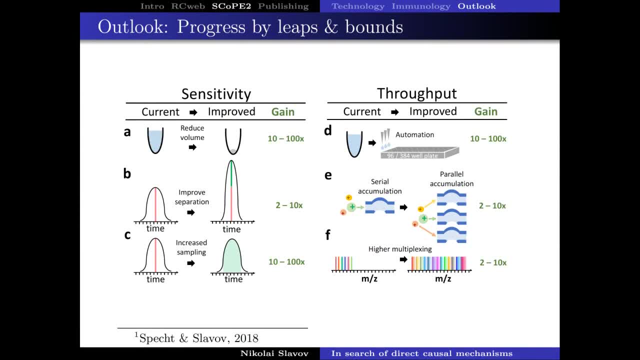 Sometimes it's lower. Our capture efficiency is definitely below 1%, So we capture a smaller fraction of the protein molecules in the cell. but because on average these proteins are about 1,000-fold more abundant than messenger RNAs, oftentimes more oftentimes. 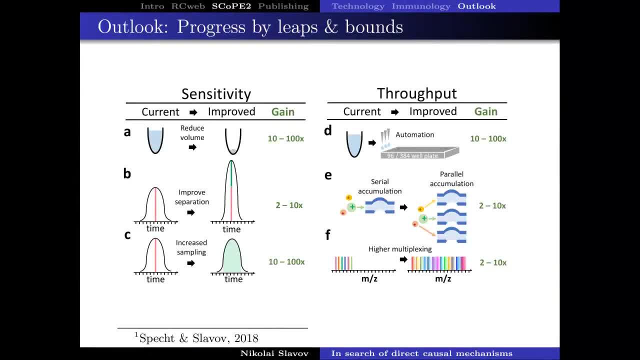 10,000.. So for each messenger RNA in a cell, usually they're between 1,000 to 10,000 protein molecules. So because there is this much higher abundance to begin with with the proteins, even if we have lower capture efficiency, we end up detecting counting larger number of protein. 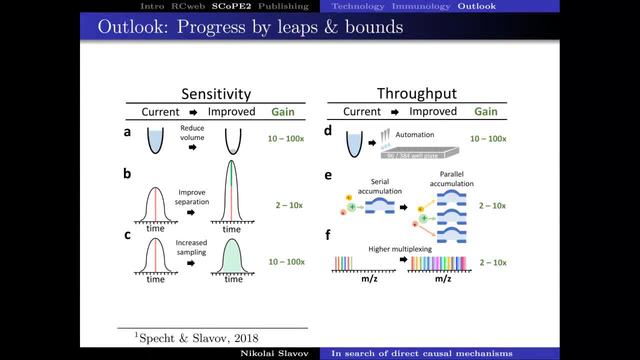 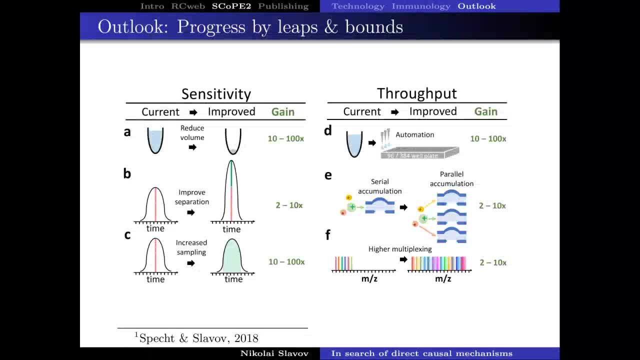 compared to the estimate for the abundance of the messenger RNA. Cool, So then. So that makes sense. So then, for the messenger RNA, you know how the distribution usually is of the negative binomial, which is similar to the Poisson that you mentioned. 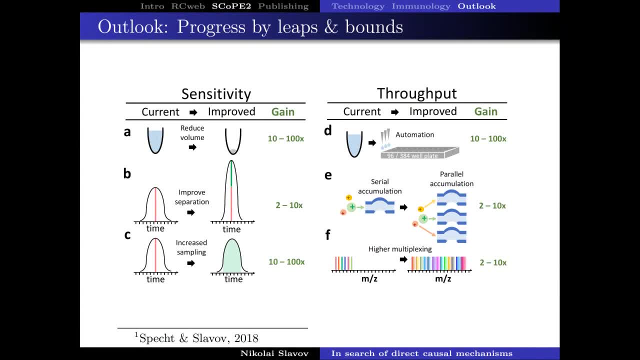 Is there an analogous distribution that's used to model like full changes in proteomics? That would be wonderful, Great question. So, with the single-cell RNA sequencing, it is well known that in a good experiment the counting noise is one of the primary contributors to the noise in the measurement. 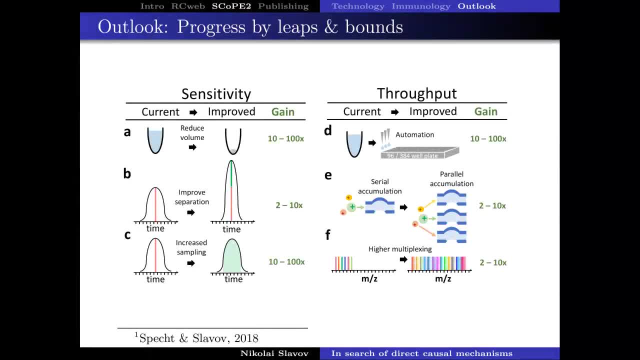 With the protein measurements. it is not clear at this point that the counting noise is our primary limitation. We have other aspects, such as variability in sample preparation and potentially co-isolation that can be used, So the distribution can be very substantial. contributors to the noise. 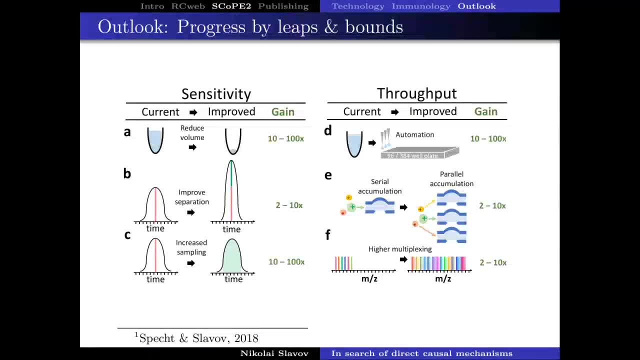 So the distribution might be different. It may not be just the counting of molecules. I think as the field matures it will be very important to model that noise distribution. But this is very new, very early days, and nobody has actually derived clearly what that. 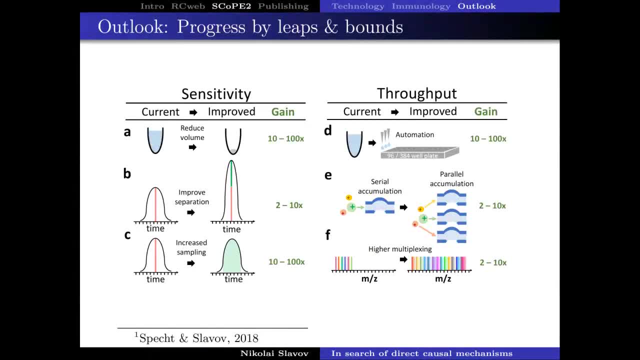 noise distribution is going to be- And my expectation is that it will not be negative- binomial Poisson. Yes, It's going to be a binomial Poisson distribution. If we get to that point, it will be phenomenal because we have the ability to further increase. 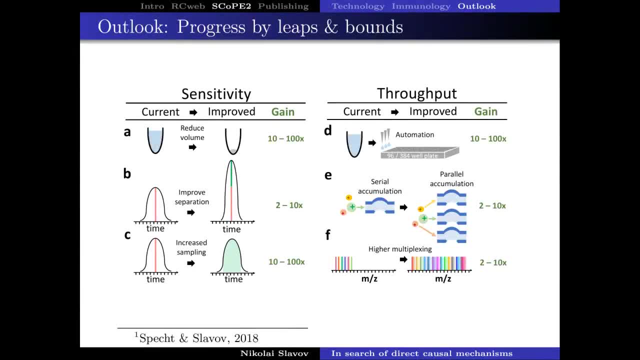 the sampling efficiency And if that's our main bottleneck, error bars can become arbitrarily small. But for that we would have to further reduce the noise from sample preparation and co-isolation and other aspects. which is all doable, all exciting things to do. 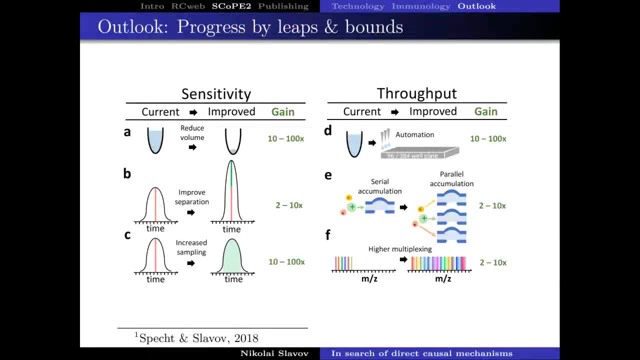 But they don't quite think we are there And we certainly don't have a good estimate for what the noise distribution is. It took a couple. So if you think of how this developed within the single cell RNA sequencing, the methods became very quickly adopted by hundreds and thousands of labs and the first papers publishing 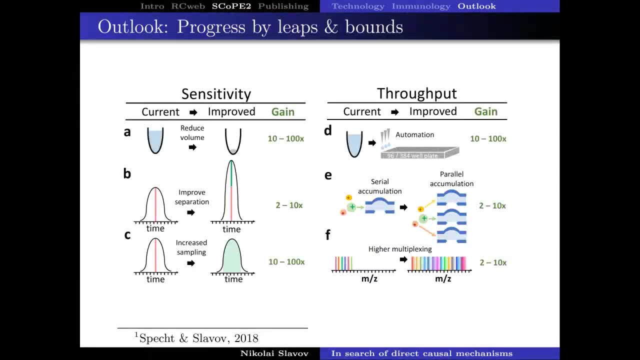 estimates of what the noise distribution looks like came three, four or five years down the road And after the first methods were developed. Cool, So is there is what about for bulk proteomics? Is there like a distribution that people usually use? It's usually the empirical distribution is commonly used. 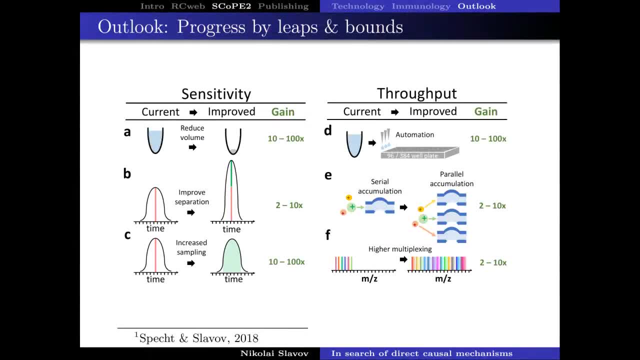 So bulk proteomics is clearly not limited by counting errors. It's limited by other errors and it's usually empirical. there, Okay, Thank you. Other questions? No, Okay, Thank you. Well, in the last 10 minutes of the class, I'm going to very quickly return to the theme. 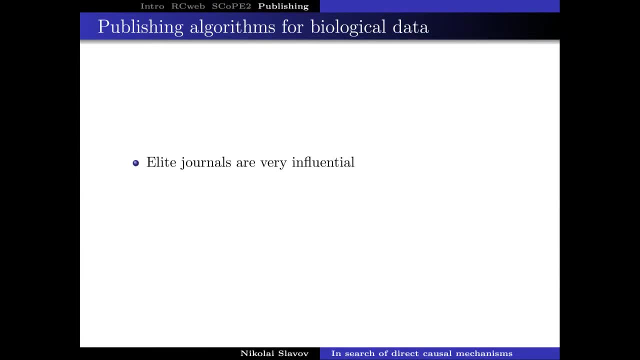 of publishing. So we have discussed that one of the- that if you want to have an impact in the public research enterprise, your results should be shared and they should be widely known There. There are more than one ways of making your results widely known and then to share them. 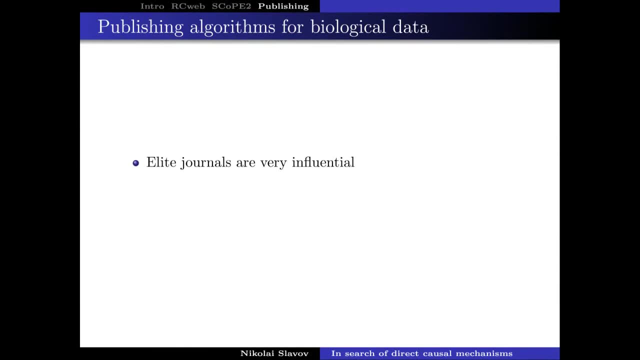 But one of the important ways to gain visibility and to share them is by publishing in influential journals and elite journals, And this is particularly true in biological sciences, but also in other fields. Usually, the more competitive the field, the more important elite journals are. 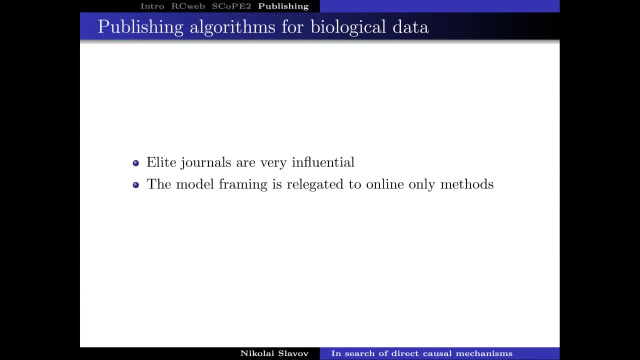 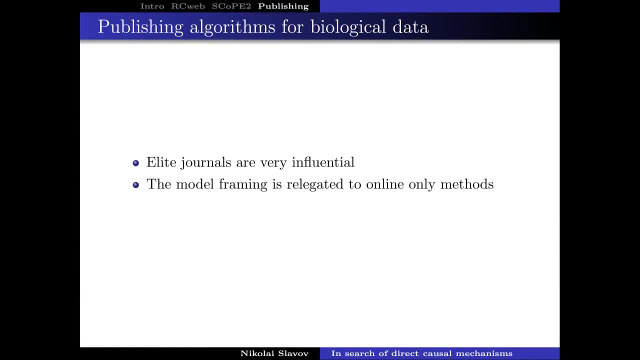 And when one writes and publishes a purely computational paper in these journals, the model framing can be relegated to the online only methods. So it is common to put technical details in online only methods. Many people who may want to use a method may not want to be immediately confronted with 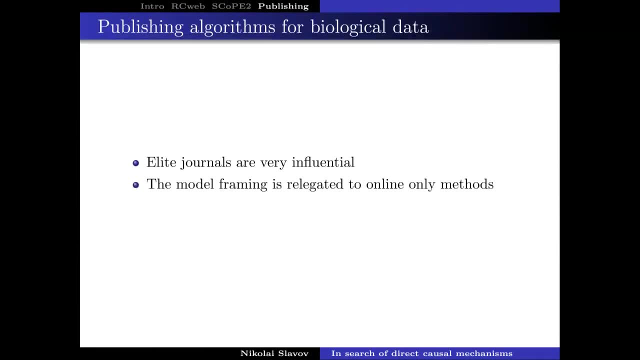 details of the implementation, But at least conceptually, what is the base of the model and how it works should be introduced in the paper. Because if the thing is relegated, If the thing is relegated to online only methods, who knows who reads it? 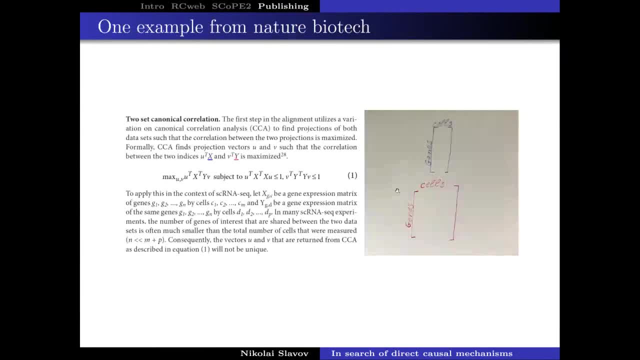 Maybe the reviewers never read it, And I have certainly come across a number of such examples Here. I'm going to share one of them of a recent Nature Biotechnology paper where, after reading the paper, I did not know what the method is actually doing, because the paper doesn't. 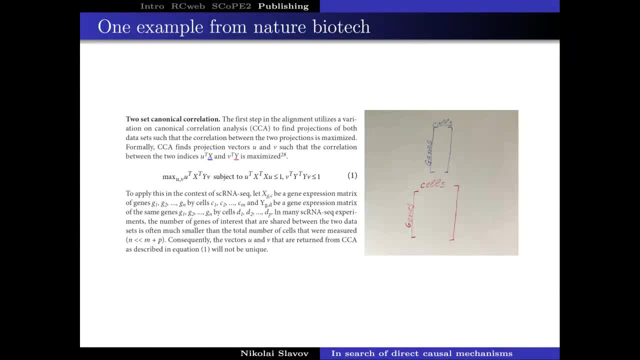 describe it. And then I went to the online only method to see what the method actually is. And then I went to the online only method to see what the method actually is. And then I went to the online only method to see what the method actually is. 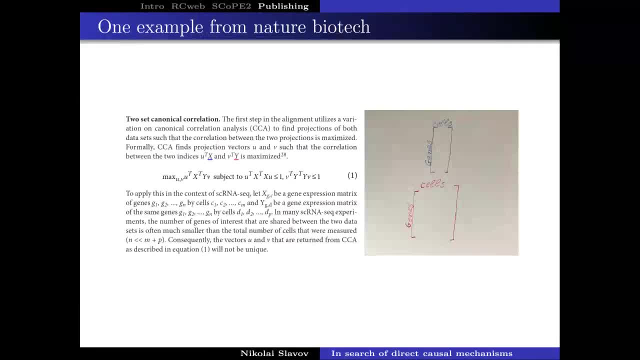 How it's being framed And the paper was trying to project into the same space single cells measured as part of different single-cell RNA sequencing datasets. So here, to the right, I'm showing the two matrices- one blue, one red- that have single 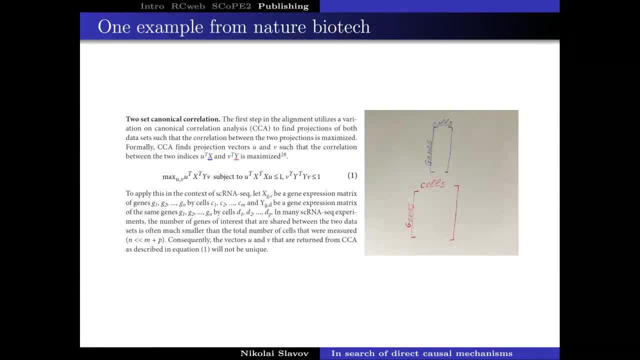 cell RNA sequencing data. They should be projected into the same space. And then, when I try to understand something, I think of what the corresponding models, really math corresponds to. So here we have the matrices: the blue is X and the red is Y. 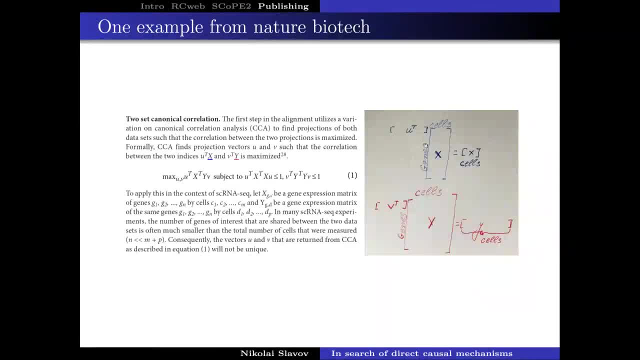 Here I have them labeled. So the method is being formulated as multiplying the blue matrix with this blue vector transposed horizontal vector on the left, And the red matrix is also multiplied by a horizontal vector on the left, And then the resulting vectors here will be correlated. 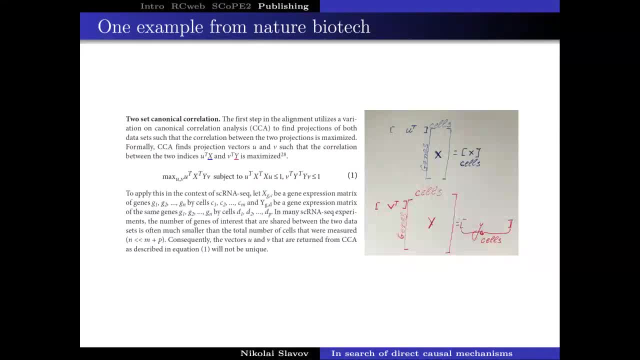 Now the problem is that this first equation formulating the problem formulates it in such a way that it's not possible to compute generally. Why will that be the case? Because when you do these multiplications here with the blue matrix, you will end up with a horizontal vector. 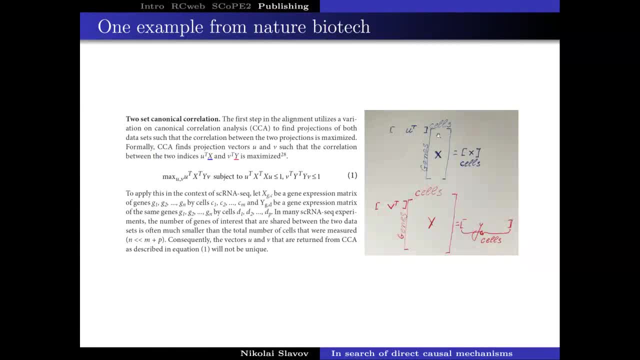 whose number of elements equal to the number of cells in this dataset. You do the same operation for the red matrix and you get another vector whose number of elements equals the number of cells in the red dataset, And the two datasets may not even have the same number of cells. 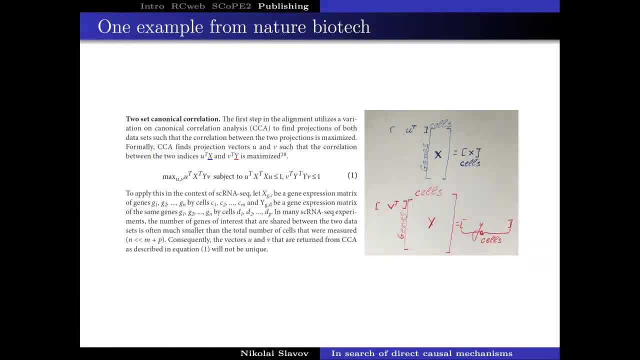 You cannot possibly correlate these vectors. It's just not defined linear algebra operation, And if somehow you happen to have the same number of single cells in these datasets, the correlation is not likely to be meaningful because the single cells would usually be ordered in an arbitrary way. 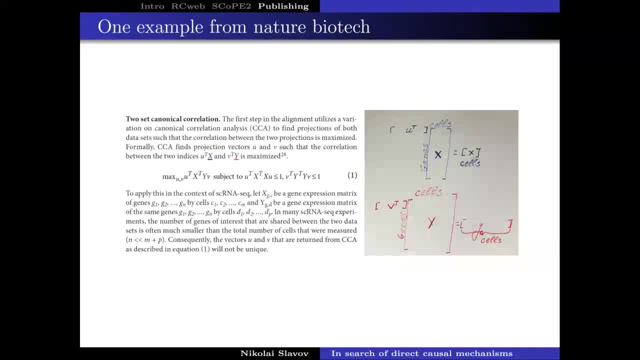 So why did I pick this particular example out of the many other examples that I could have picked? Because when I brought this example to the attention of the senior author, the senior author told me that he will ask the graduate student who did the work and never get back to me. 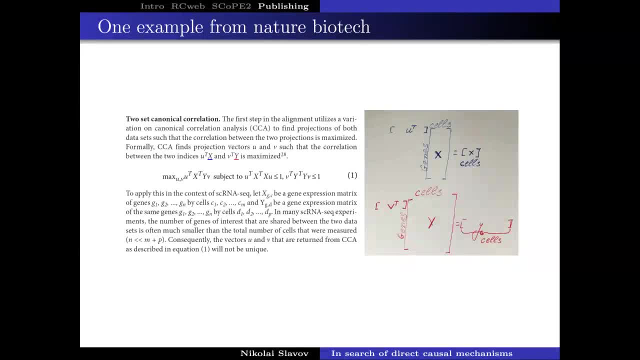 And I felt that this is particularly inappropriate because the senior and corresponding author would normally take the responsibility for such a thing, And this is clearly not something about an experiment done by a student in a way that the PI doesn't know, but it's something that, simply by looking, 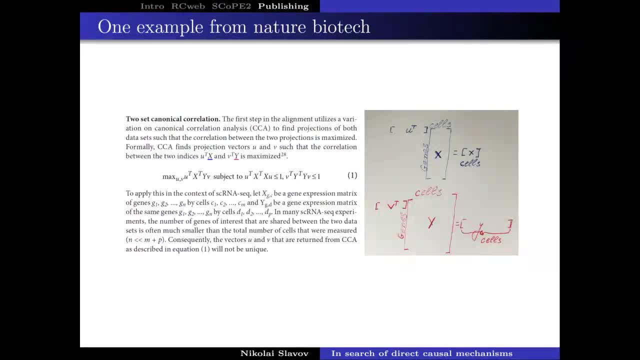 at the contents of the paper. one knowing linear algebra, one can immediately see that there is an issue with the formulation of this problem. It's also emblematic of the kind of problems that arise if something is being relegated to supplementary information because that alone might signal. 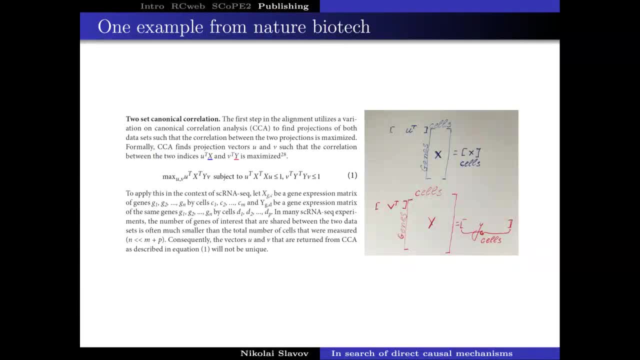 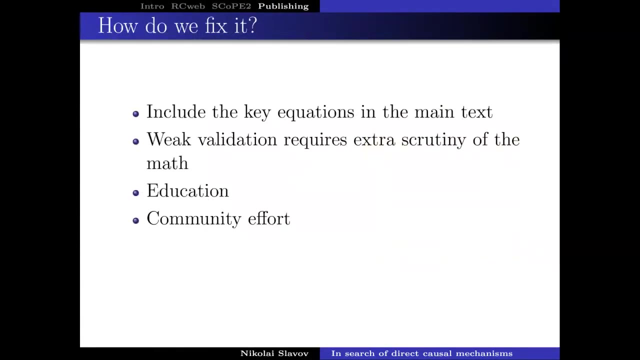 that perhaps it's not as important And the framing of the problem is important, in my opinion, and it can also result in lower probability of the reviewers being able to catch it, because maybe they didn't peruse the online only methods. So I don't mean to despair and to say 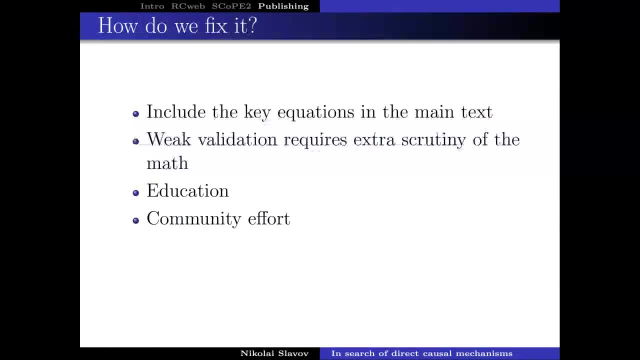 that this makes publishing useless and that the system is broken. No, the system is working to a degree. It's certainly suboptimal and has many problems, but to avoid that and to help minimize the probability of those things happening, i think it's very important to include equations. 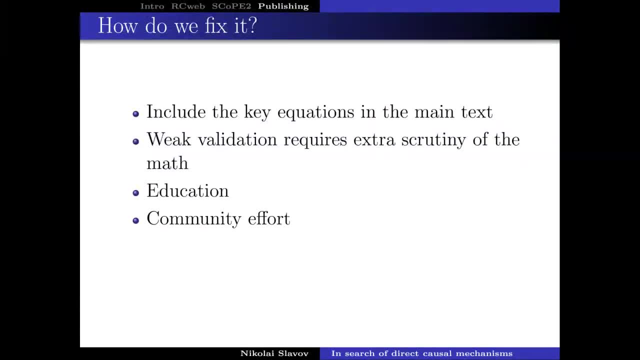 especially important equations in the main text of your papers and if it's very hard to validate your results empirically- as it's often the case with single cell measurements because there isn't another orthogonal measurement usually that you can easily do- then it's even more important that 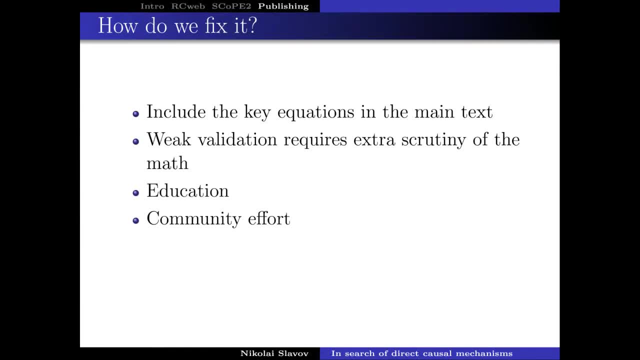 computational algorithms be very carefully examined. and of course, all of that can work if the scientists and engineers are well educated and have the required skills to understand methods. you shouldn't use algorithms and methods as black boxes. i put in my data, i get the plot and i include it into my paper. you should really understand what what that algorithm is doing. 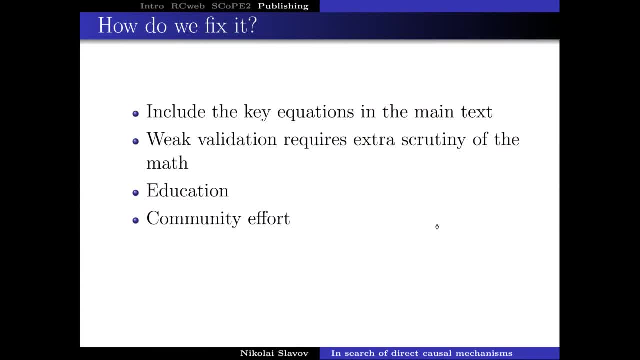 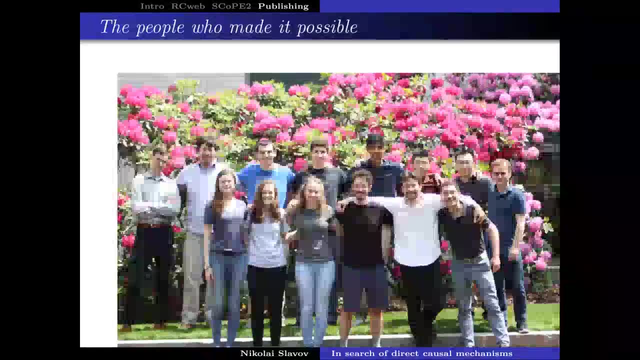 and ultimately that has to be done as a community effort by by everybody, uh. so i'm gonna finish with that my presentation, uh, thanking uh.